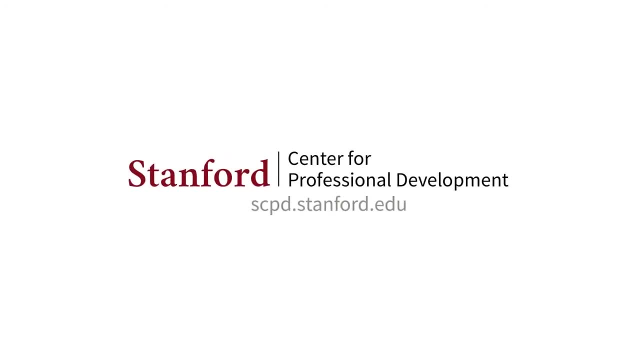 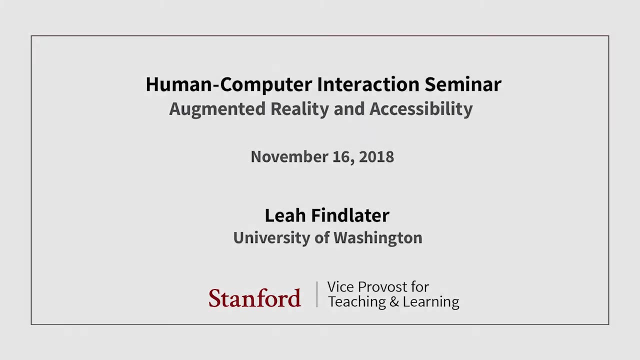 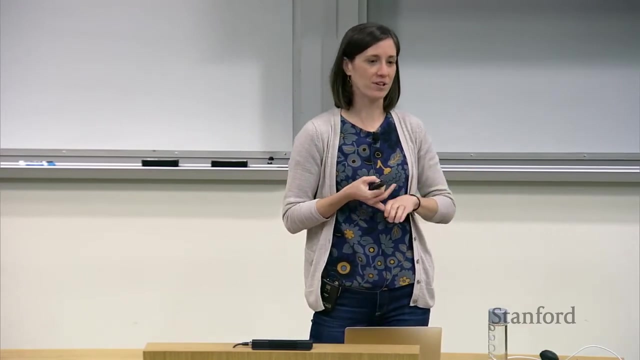 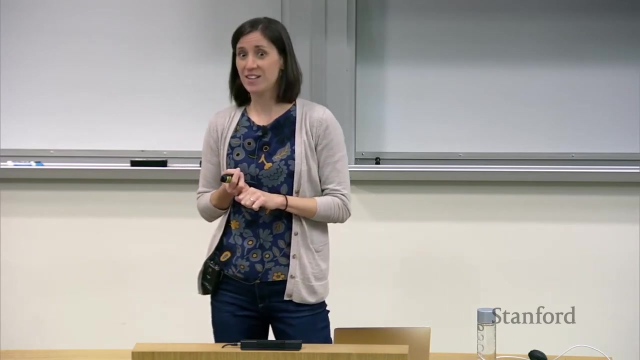 Before I get started, I want to just mention that the work I'm going to talk about is in collaboration with many people, mostly at the University of Washington and the University of Maryland, And then the students who led most of this work include Mitu Malu Drew. 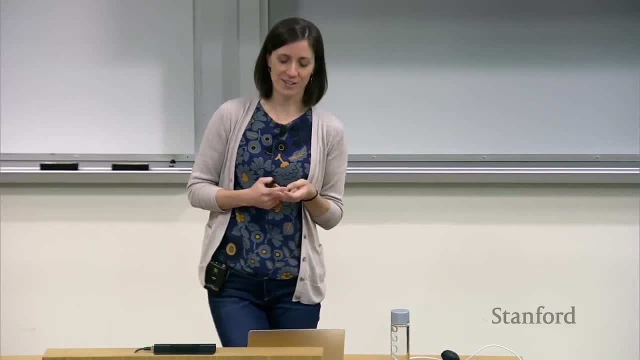 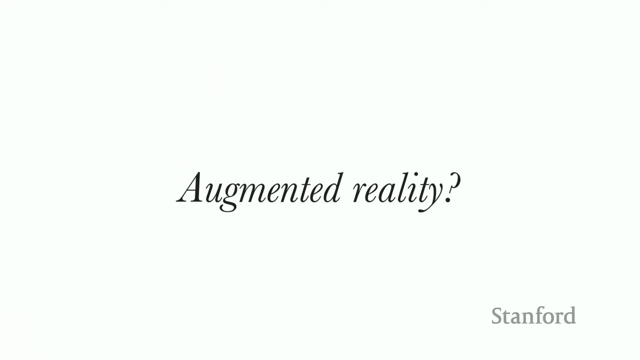 Jane Kristen Williams and Hallie Profita, who is actually at the University of Colorado. So let's start by taking a moment to consider augmented reality. What comes to mind when you think about augmented reality? Can you shout out some technologies or applications? 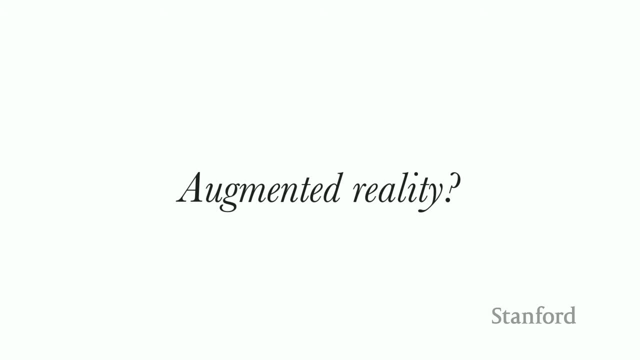 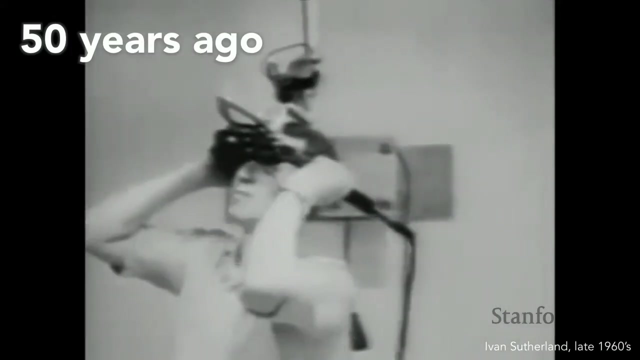 HoloLens, HoloLens, okay, Google Glass, Google Glass. Did you have one more now? No, Okay, all right, great, So thank you. So here are a few more examples that I've put together. So this is about 50 years ago on Ivan Sutherland's. 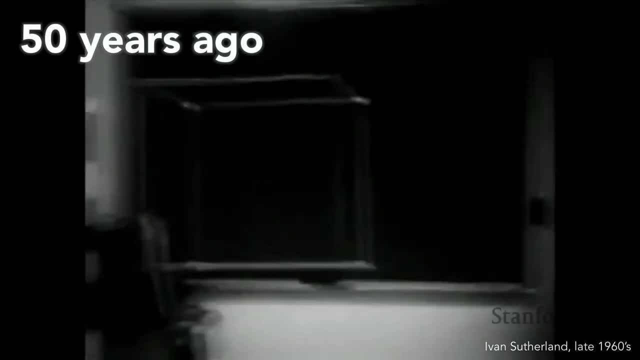 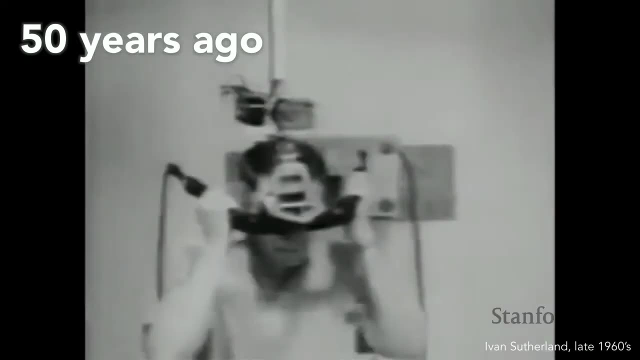 Sword of Damocles, And this was perhaps the first head-mounted display. It overlaid visual information, while not really on the real world, but it was see-through so you could also see the real world. So, arguably, augmented reality. And then, about 25 years ago, AR research in 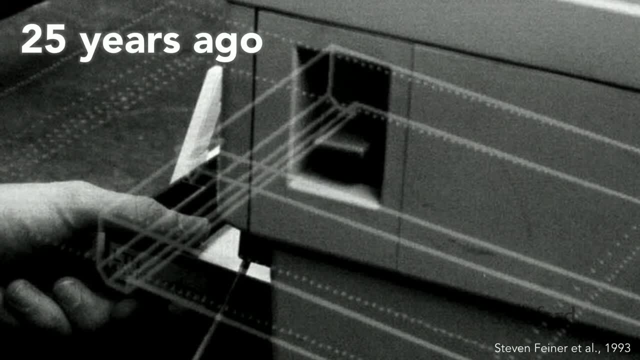 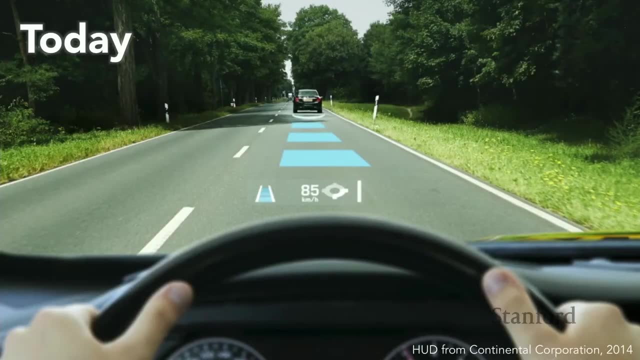 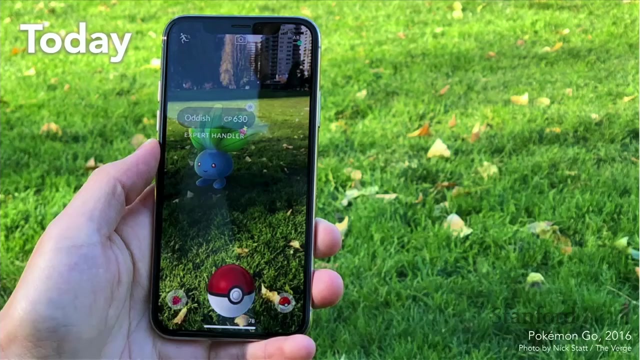 HCI really started to take off, And so this is an example from Steve Feiner and colleagues writing augmented instructions here And now. today, we actually see AR in mainstream use. We have things like heads-up displays, head-mounted displays like the HoloLens here And then of 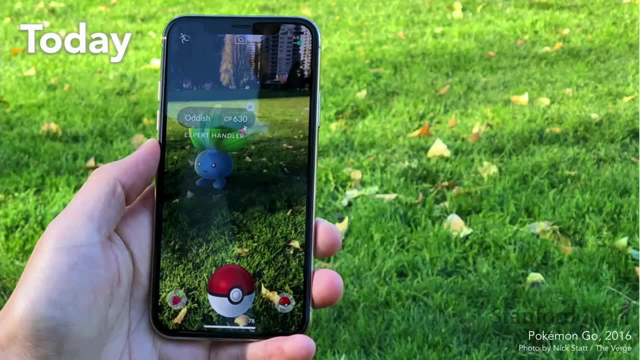 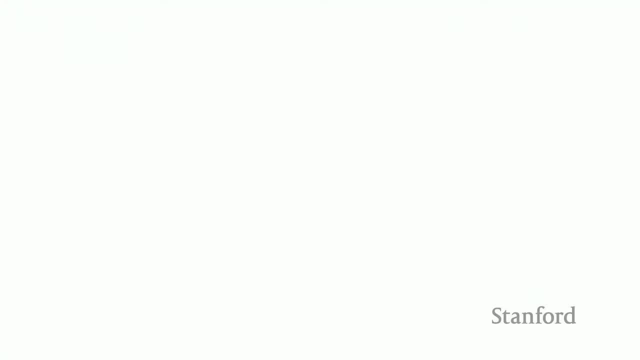 course, AR games, which was also mentioned by you. So this is Pokemon Go. How many people have played Pokemon Go? Quite a few, Okay. So let's pause for a moment and think about how AR can support people with disabilities, so people with a range of physical, sensory. 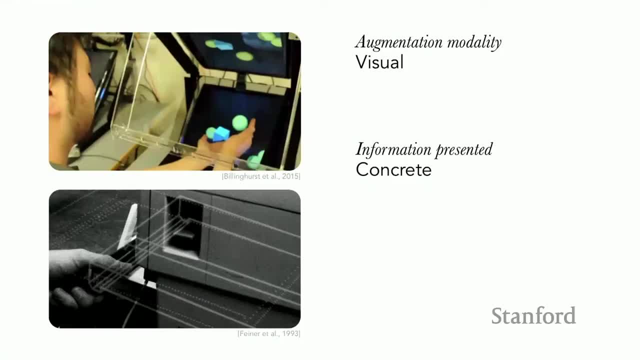 and cognitive abilities. Okay, The examples that you shouted out, as well as the ones that I just showed you, I think all of them augment the real world with virtual, concrete, visual information, And that is typically what we think of when we think of augmented reality. But visual information is, of course, 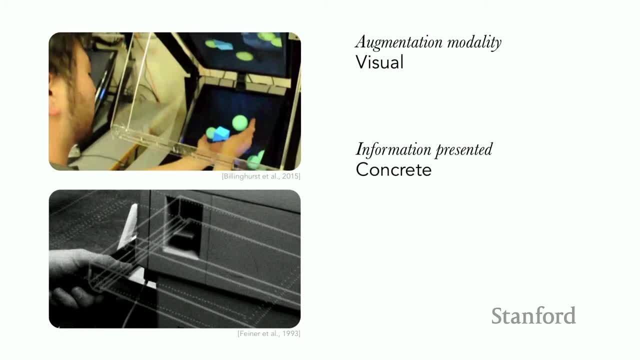 not accessible to blind users, for example, And so if you look for AR examples and blind users, you might get things like audio or haptic output to describe who's in the room, or navigation instructions and so on. So auditory and haptic modalities have been 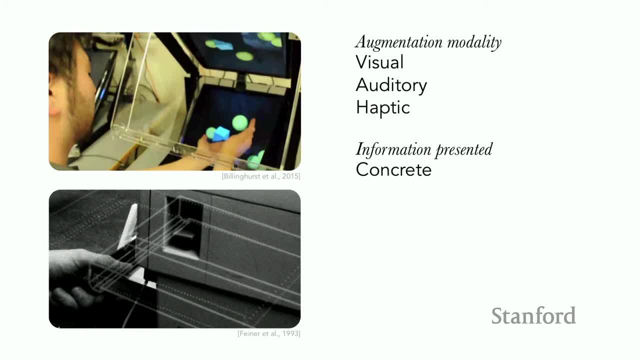 much less explored in AR But could be. And then we don't have to focus only on concrete information. We could think about more abstract information, And that can be particularly important, for example, in augmenting cognitive abilities like language production. And then, when we're talking about augmenting abilities just generally, some enabling technologies. 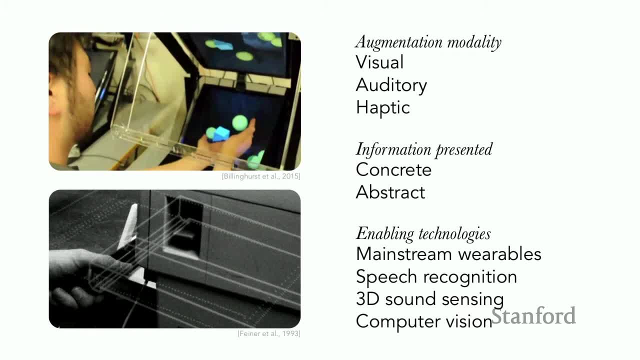 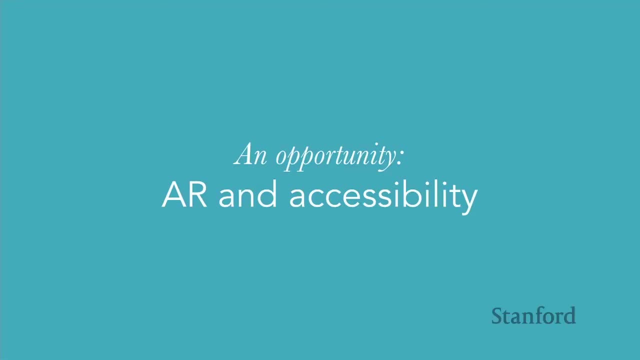 that I'd like you to keep in mind include mainstream wearable devices, speech recognition, which has greatly improved in the past decade, of course, 3D sound sensing and computer vision. So, with all of this in mind, for AR, today I wanna talk to you about how we can use AR. 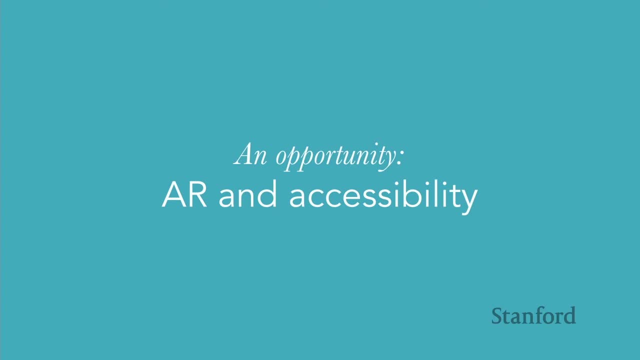 to improve real-world accessibility for people with disabilities, And I think this is an area that holds tremendous opportunity and there's a lot of exploration that can be done here. So there's some work, but sort of relatively little. So consider how AR could address. 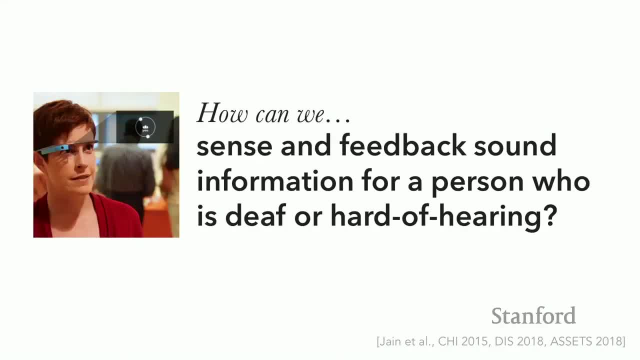 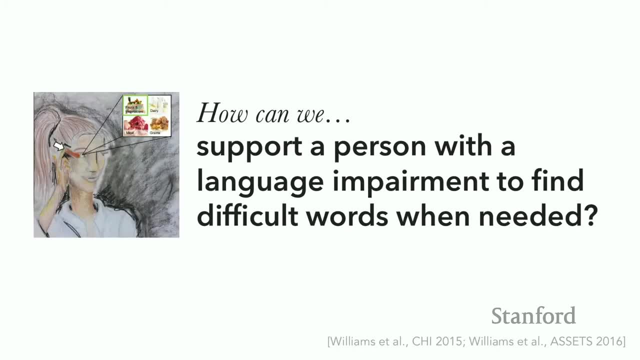 some of these questions that have motivated our work. How can we sense and feedback sound information to a person who is deaf or hard of hearing? How can we support a person with a language impairment of finding difficult words when needed? Or how can we augment a blind person's sense of touch? 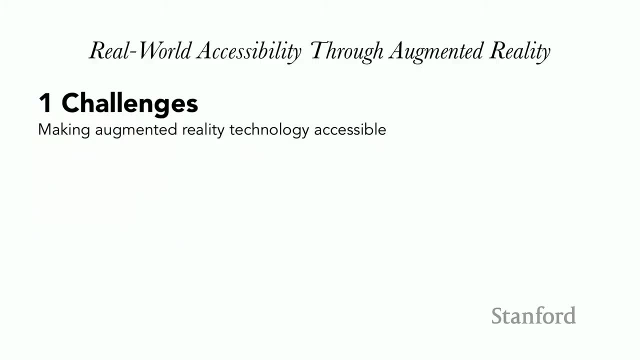 to help interpret non-tactile information. So, toward the vision of improving real-world accessibility through augmented reality, we've followed three threads of research. The first is to address accessibility challenges with augmented reality technologies themselves, so making those technologies accessible. The second is to use existing technologies. 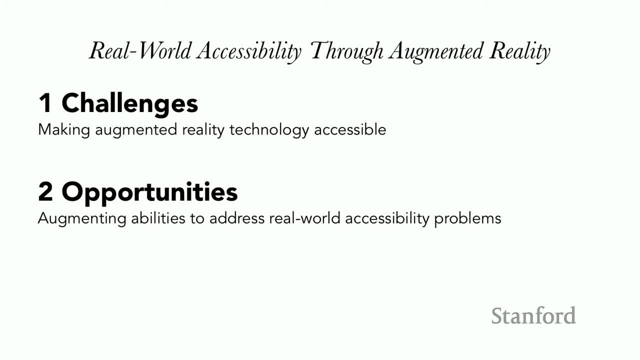 and create new ones to augment abilities in a way that addresses real-world accessibility problems. And then the third thread of work is to consider some of the practical issues that we will need to address if we want to actually have some of our solutions be adopted in the real world. 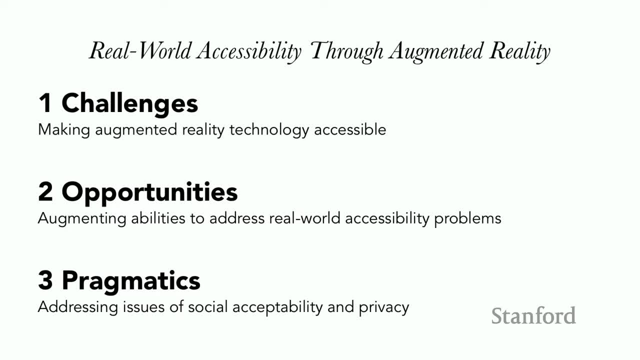 So these can include social acceptability and privacy. So I'm going to spend most of my time on the second and third threads in this talk, but I want to give you first one example of this first thread of work on, to just emphasize the importance. 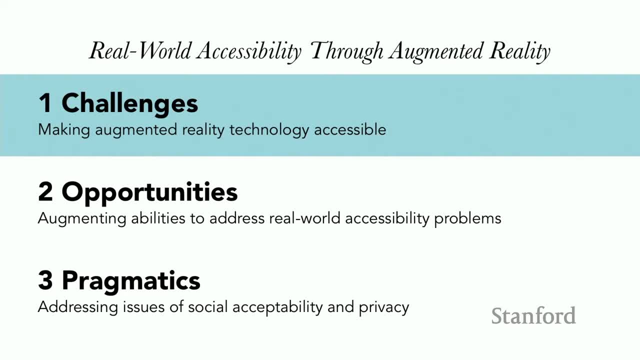 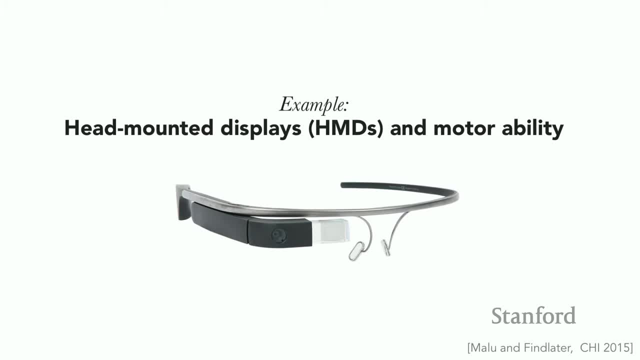 of considering accessibility when we're designing new AR technologies. So in some of our earlier work on AR and accessibility, we were looking at head-mounted display use by people with motor impairments. Of course, this is Google Glass here: The way that you manually control Google Glass. 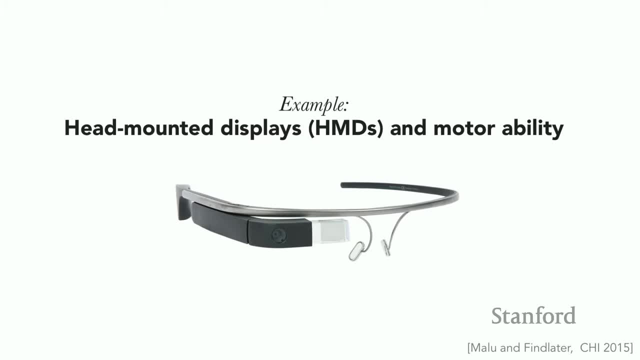 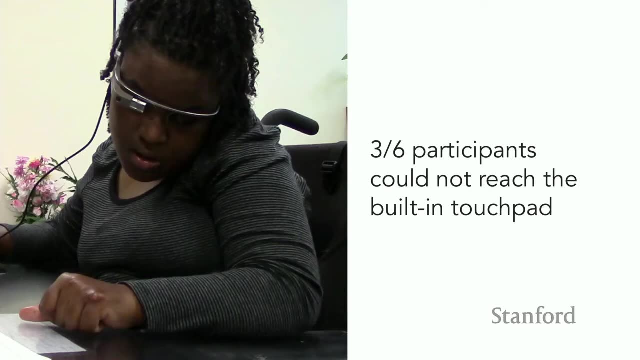 is by swiping or tapping on that side, that touchpad on the side of the device. In our very first study we recruited six participants with motor impairments and three of those six participants could not actually touch the side of the device. 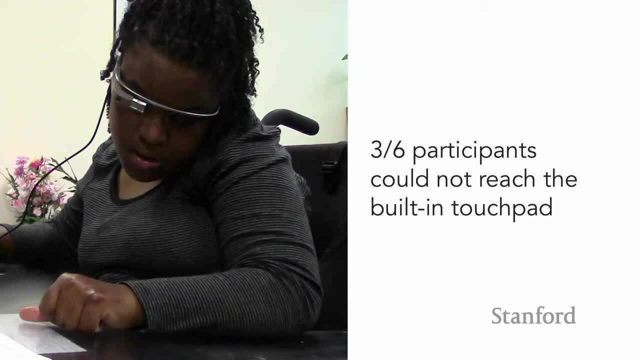 They could not reach up and touch it, So that is obviously a big problem. for manual input. You can use speech input for this device, but speech input is not accessible to everyone. For example, someone might have dysarthria and of course it's not always appropriate. 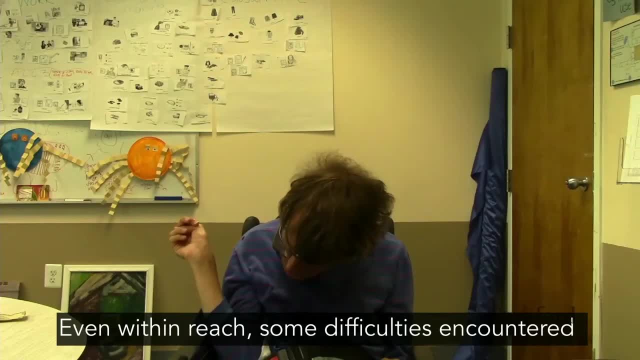 So even for the three participants who could reach up and touch the side of the device, there were still some issues. This video clip here is gonna show a participant swiping the side of the device, but with such force that he displaces the device. 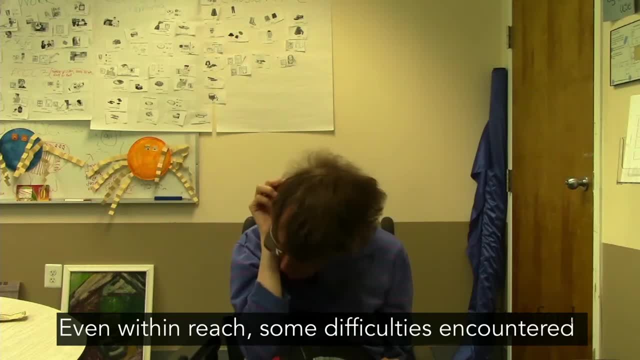 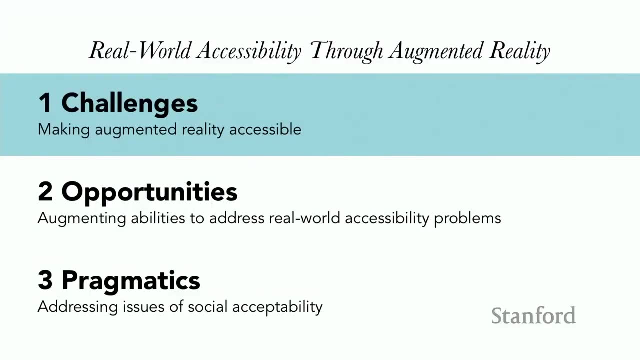 and then can no longer see the screen properly. All right, so that is just one quick example to emphasize the importance of considering accessibility when we're creating new AR technologies, Because if we don't make these technologies accessible, then we won't be able to take advantage. 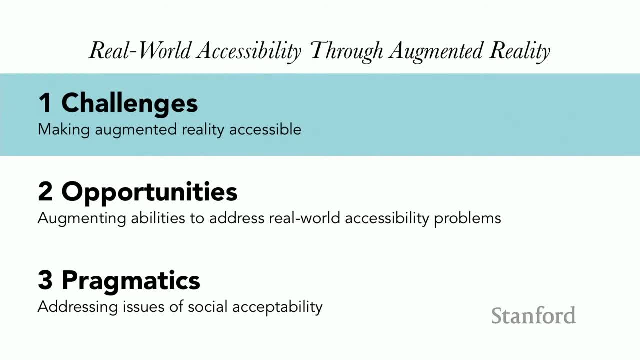 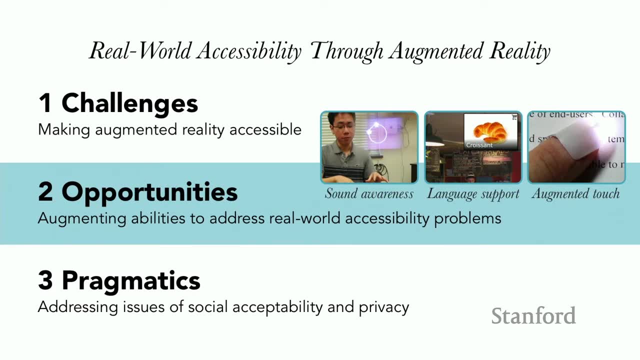 of the opportunities that they also provide. Now I wanna turn to exploring some of these opportunities, and I'm gonna talk about three projects where we've built and evaluated systems to augment sound awareness, language support and physical touch. starting with sound awareness. 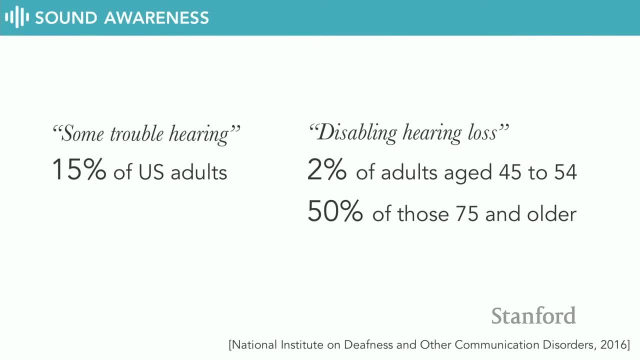 So in the US of adults report some trouble hearing- This is in the US Census- And the rates of disabling hearing loss, which is the exact phrase that's used, are much lower: About 2% of adults aged 45 to 54, but they increase substantially with age to about 50% of adults 75 and older. 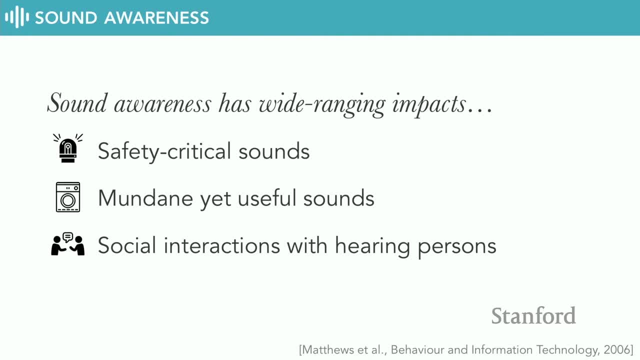 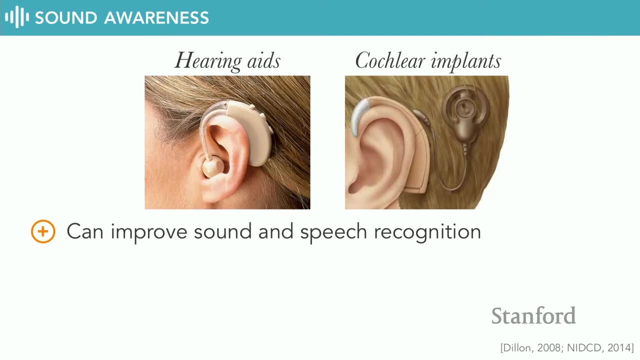 Now sound awareness has wide-ranging impacts for people who are deaf or hard of hearing, from safety-critical sounds like fire alarms to mundane yet still useful sounds like the clothes dryer, ending a cycle to conversations, spoken conversations with hearing conversation partners. Now, hearing aids and cochlear implants can help with sound and speech recognition. 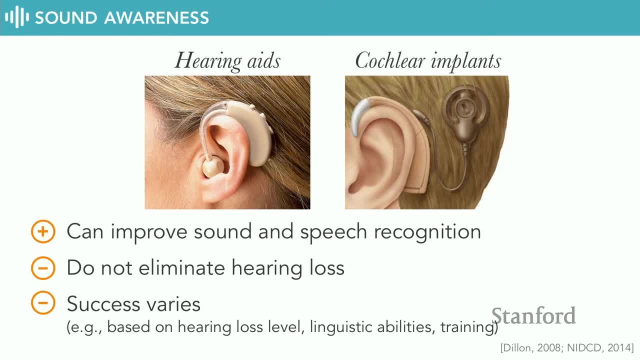 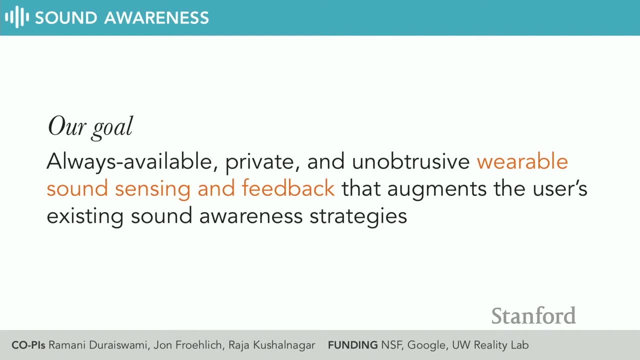 but they do not eliminate hearing loss, and their success can vary based on a number of factors like the user's hearing loss level, their existing linguistic abilities, as well as training and support. So our goal in this project is to- Oh yes. 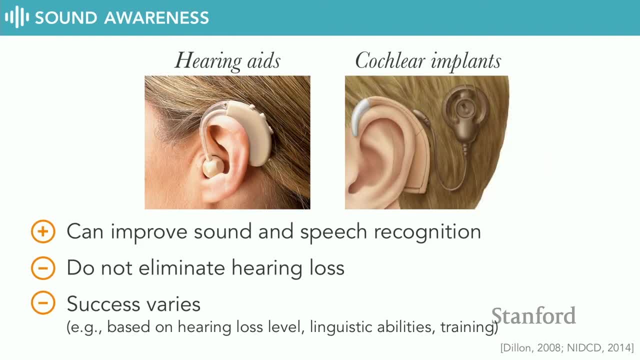 Sorry, Not being as much of an expert in this area. I wonder: why would we not consider something like a hearing aid or a cochlear implant, an augmented reality system? I had sort of always thought of it as sort of a visual overlay, but you're taking a much broader. 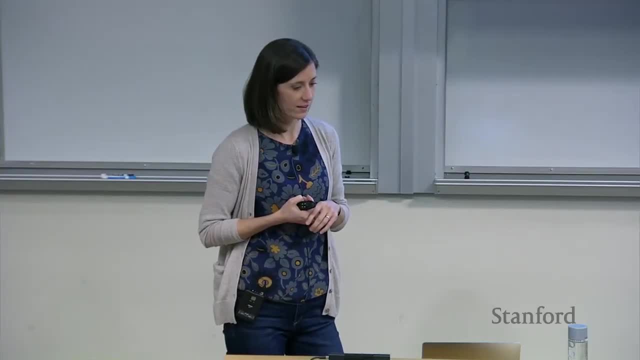 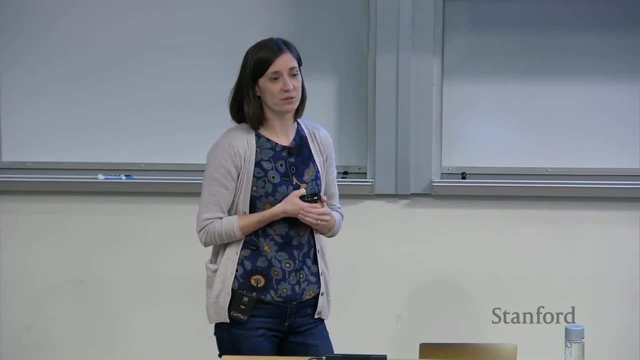 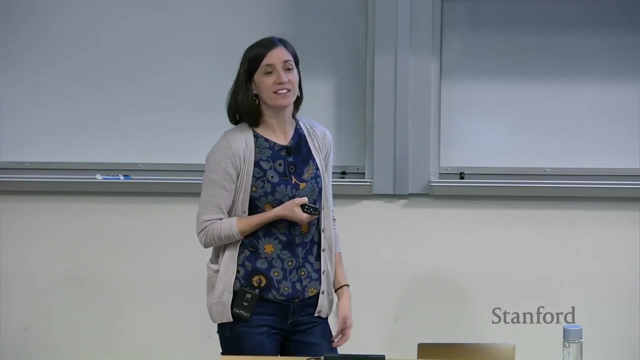 definition. so does this fit in as an AR system or not? Yeah, I think it just depends on how broadly we define AR. So I could be convinced to say that a hearing aid or a cochlear implant could be considered an AR solution, I mean, 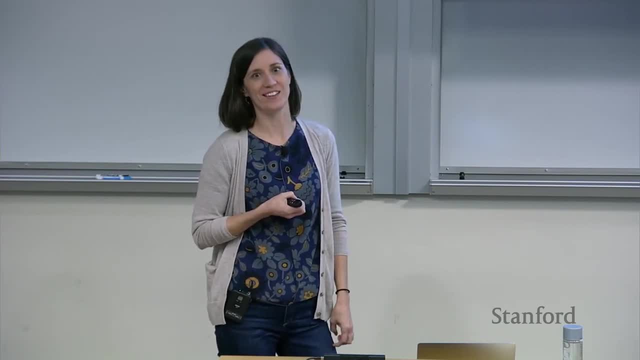 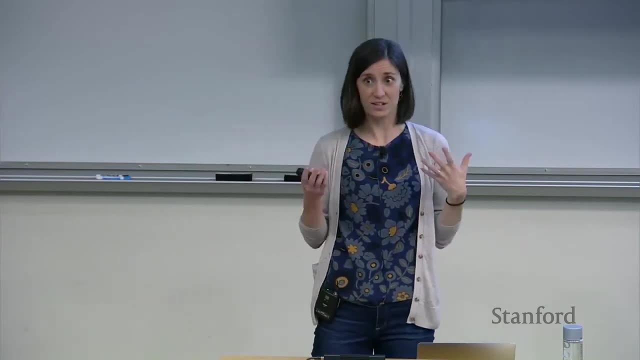 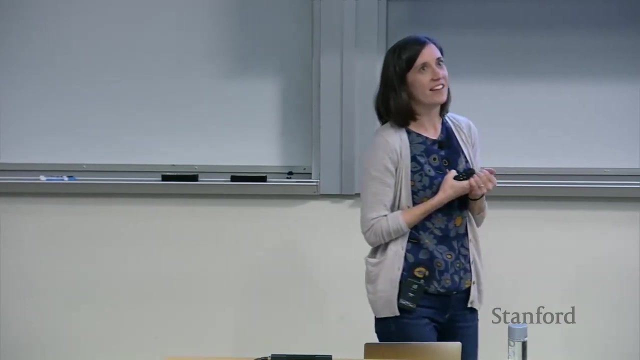 once you think about AR broadly, then, beyond this typical setting of concrete visual information, and even registered in 3D space, which is a common definition of AR, then, yeah, there are lots of things that could be considered AR. I think that it gets especially exciting. 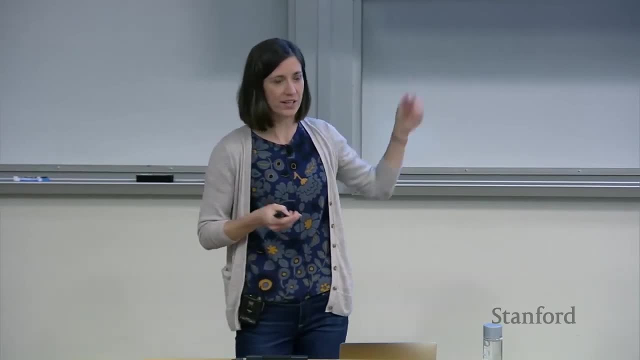 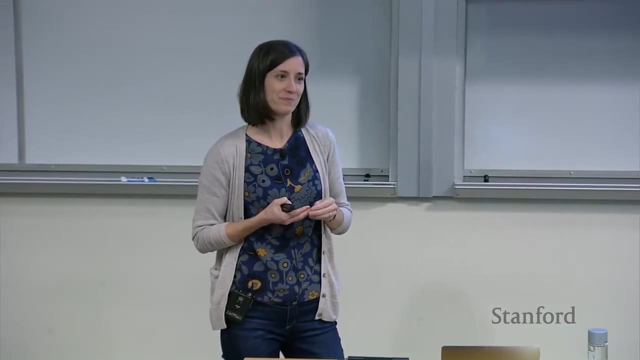 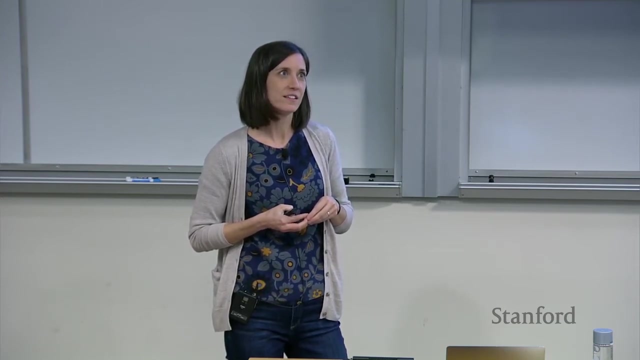 when we start to introduce smarts into the system, and there certainly are hearing aids that provide more intelligent filtering than others and so on. But yeah, I would expect inside the accessibility community these kinds of things would not be considered augmented reality, though Like people wouldn't introduce these in their papers as augmented 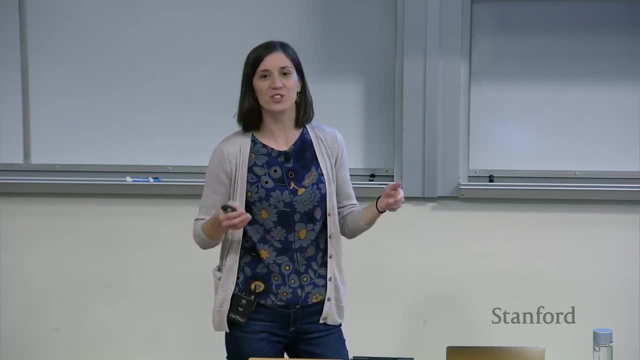 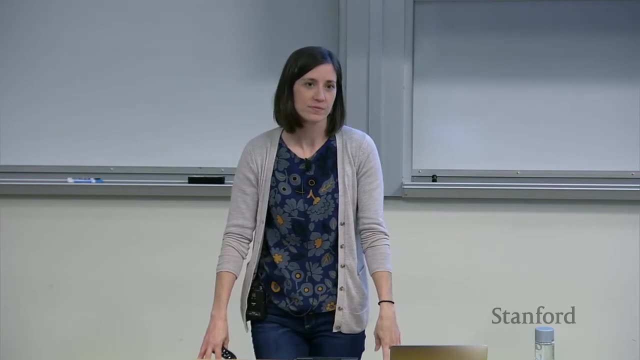 reality systems? No, I mean. so Is there a philosophical discussion that we could have about this? Do they ever have information other than the sound or speech? For example, do you ever hear like a beep to say: oh, the person's over there who's talking versus theirs Is? 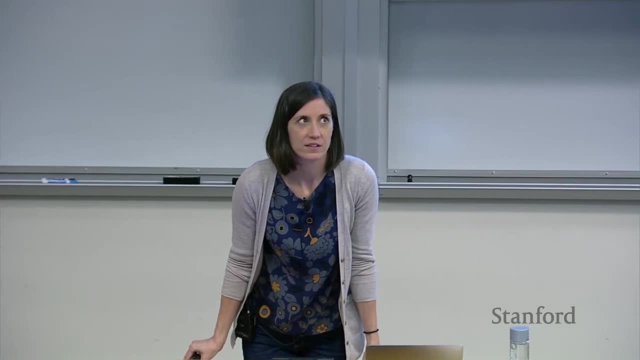 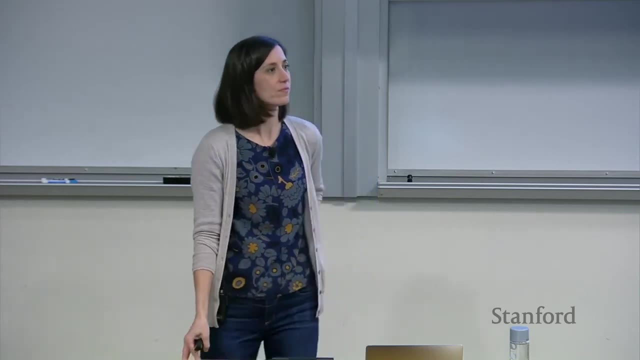 there any ever additional information In the existing stuff like that? Yeah, any such system Do they ever augment? Well, there is the shift-shifting version of the hearing aid which if you have or hearing some frequencies, it'll shift those frequencies. 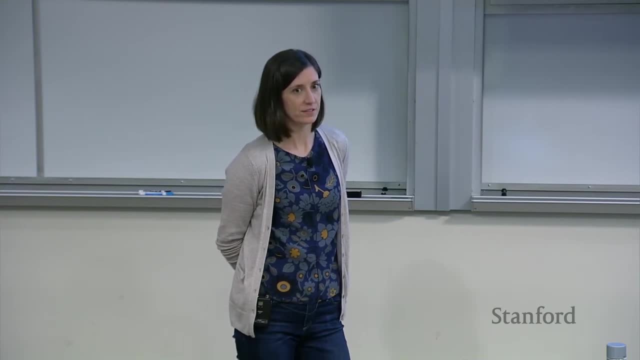 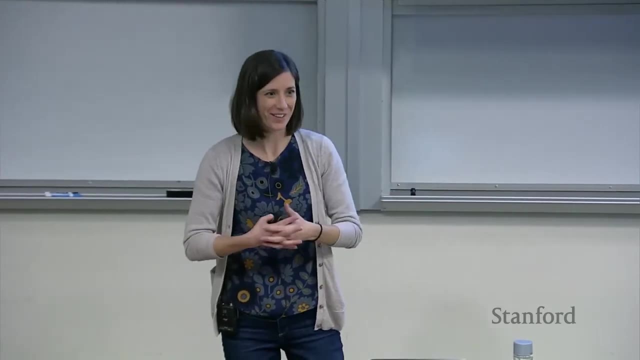 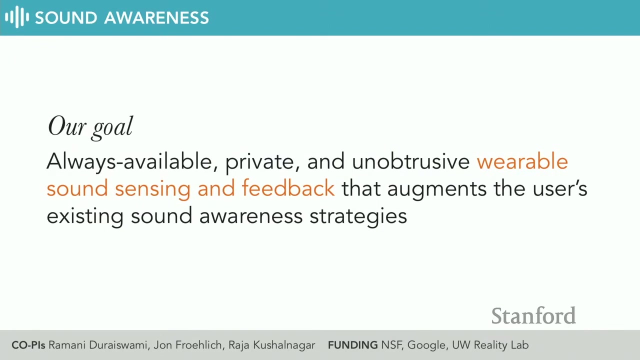 So it's changing. Interesting Thanks, Yeah, I mean, I think that we're going to see sort of worlds coming together more than they are currently, And that's what the trend is. Okay, So our goal in this project is to provide- always available, private and unobtrusive 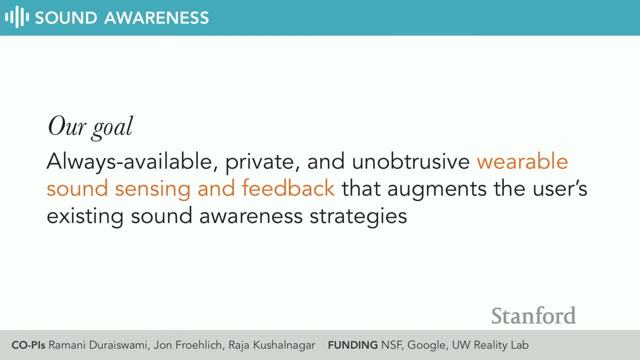 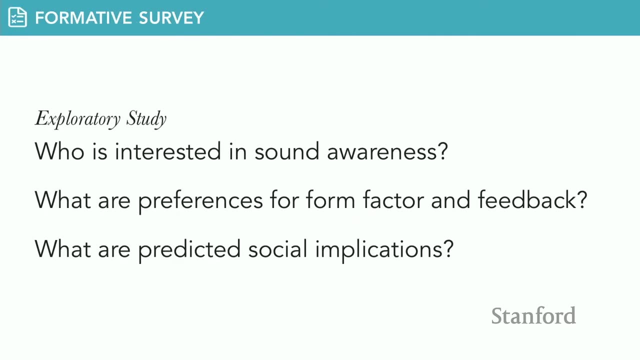 wearable sound sensing and feedback and to do so in a way that augments the user's existing sound awareness strategies And that could include using a hearing aid or cochlear implant and other cues. So this is a large project and I'm going to talk about a few studies here. The first 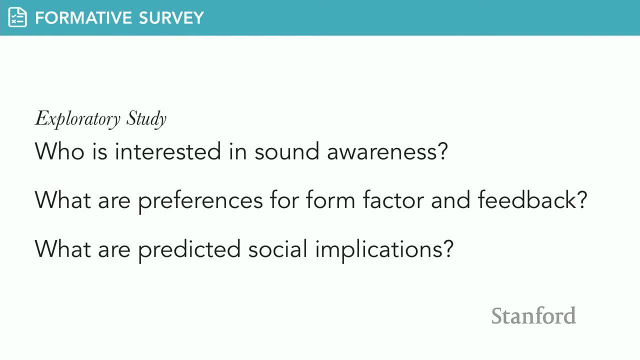 one is an exploratory study, So here we were interested in understanding who among people who are deaf or hard of hearing is hearing, What preferences do they have for form factors and feedback modalities, And what are some predictive social implications that we might want to keep in mind when we're designing. 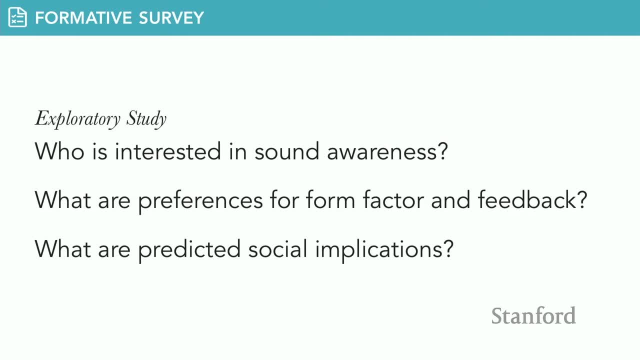 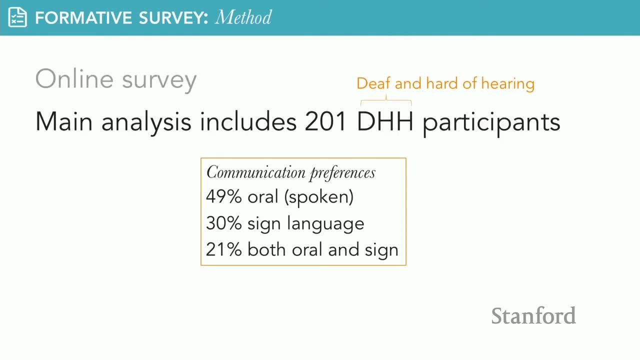 new technologies. So here we conducted an online survey and we recruited over 200 deaf and hard of hearing participants And if you look at their communication preferences, about half of them preferred oral or spoken communication, 30% preferred sign language and then the rest preferred 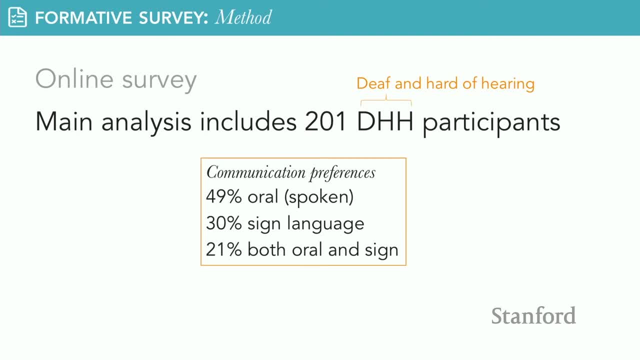 some mixed language And the rest preferred some mix of those two. And this is important for sound awareness because you can imagine if somebody is deaf, embedded in deaf culture, prefers sign language, maybe lives at home with other deaf, sign language fluent family members, then they might not be as interested in sound awareness as somebody. 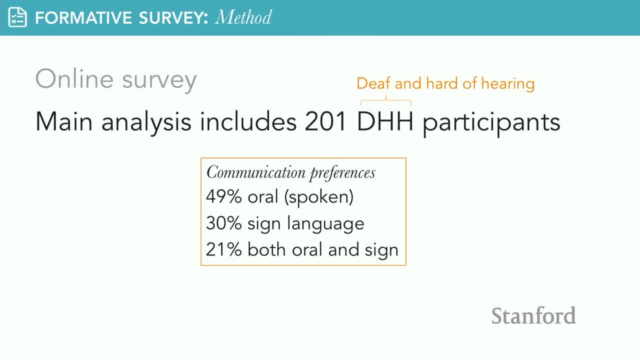 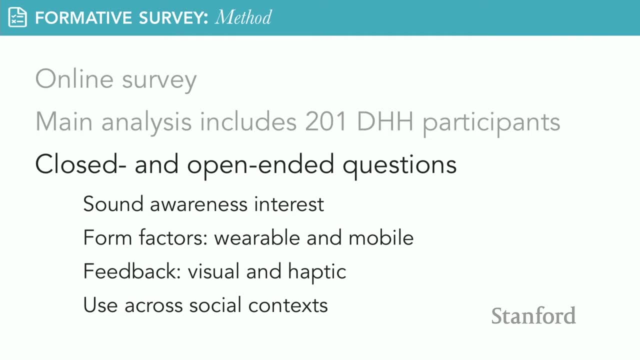 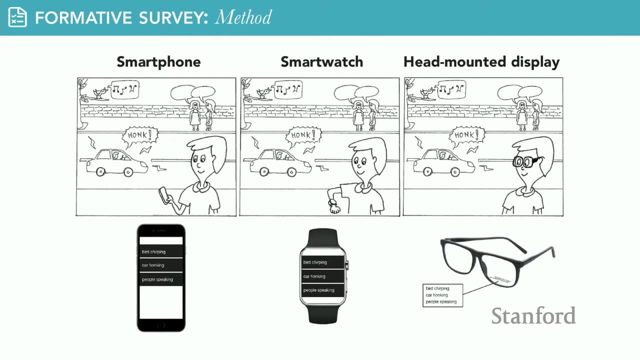 who has age-related hearing loss and has been relying on sound for decades. So we had questions about sound awareness, interest, form factors, feedback and sound social contexts. So we showed participants or described a set of scenarios, and here you can see some of 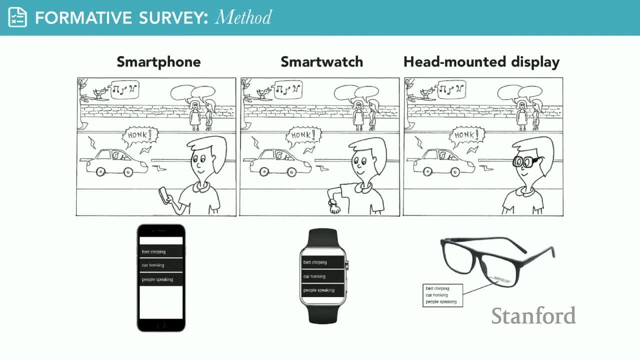 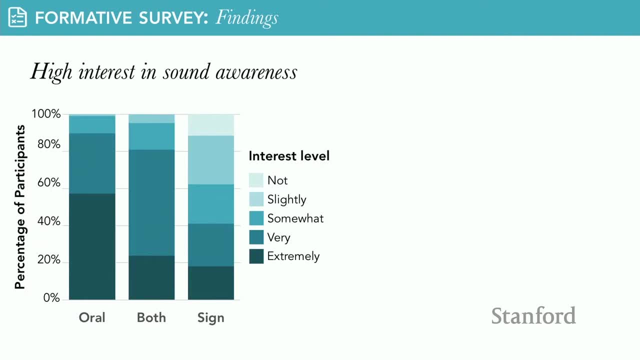 these that showed both speech and non-speech sounds occurring, and then feedback through visual and haptic modalities on a smartphone, a smartwatch and a head-mounted display. Overall, we saw that there was high interest in sound awareness. In this graph, what you're seeing are the three communication preference groups on the 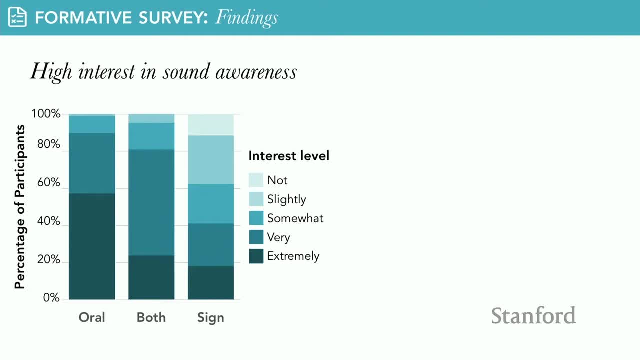 bottom oral both and sign And then darker colors indicate stronger interest in sound. So 73% across all the participants were very or extremely interested in sound awareness. A logistic regression analysis to understand what demographic factors were predictors for sound awareness interest levels showed that this communication preference was the most. 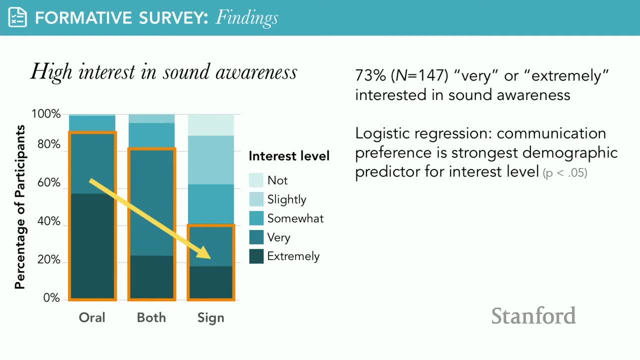 important predictor and was significant. So the sign language group, for example, was less interested in sound than the oral communication group, But still the sign language group- more than half of those people- were at least somewhat interested in sound In terms of general interest in sound types and sound characteristics. the results here: 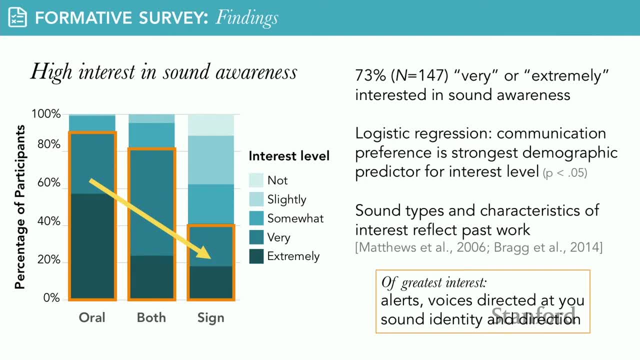 largely reflect past work, including some of James Landay's from a while ago, And this includes- so you don't remember- Tyra Matthews. Okay, so this includes urgent alerts, voices directed at you, sound identity, and so on. 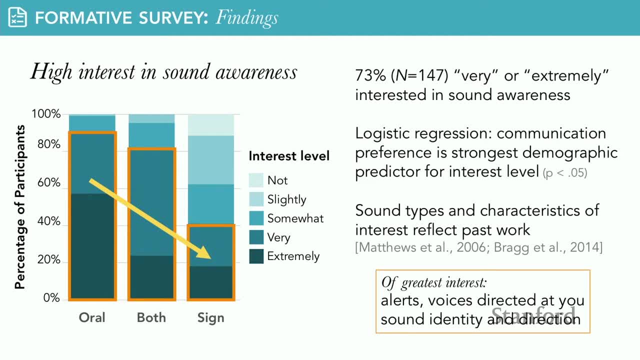 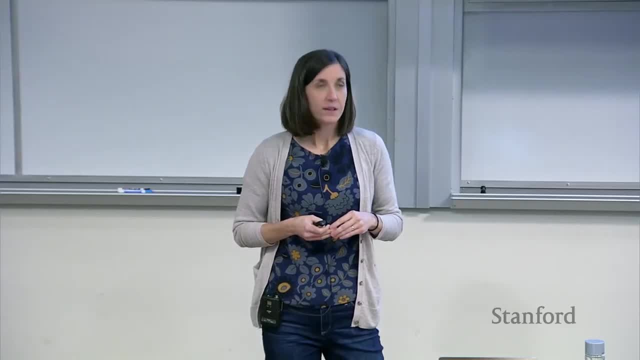 And of course, there were more Yep. Do you have any indication why people who use sign language are less interested than people who use oral communication? That doesn't like seem to make a lot of sense, Right? so why people who use sign language are less interested in sound than people who? 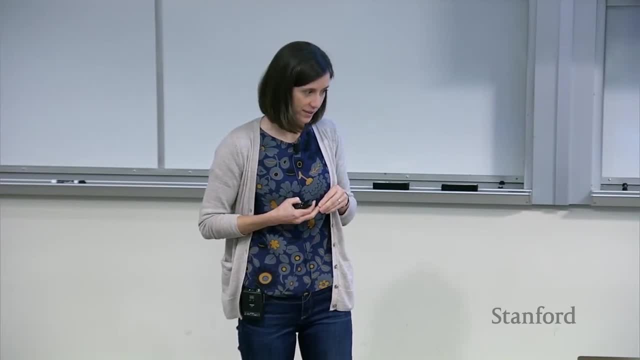 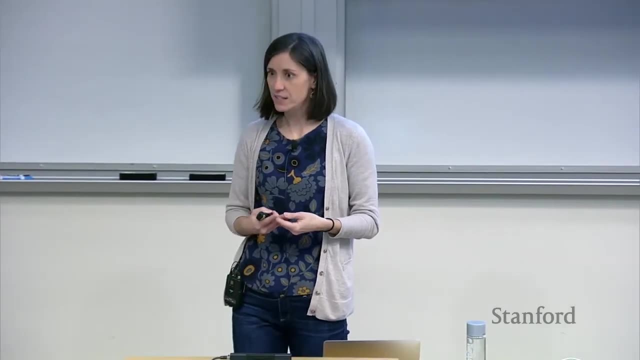 use oral communication And I think that it has to do with a number of factors So that it might have something to do with cultural identity. So you're in a culture that embedded perhaps in a culture that doesn't have a lot of interest. 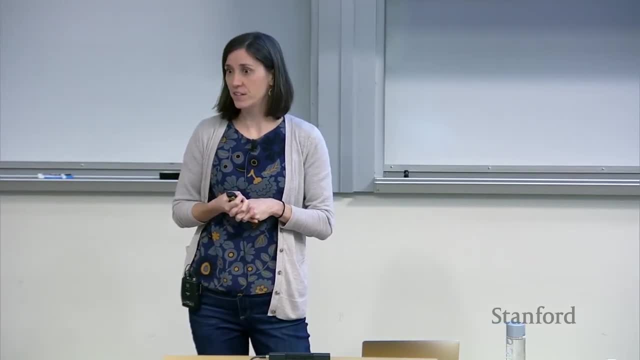 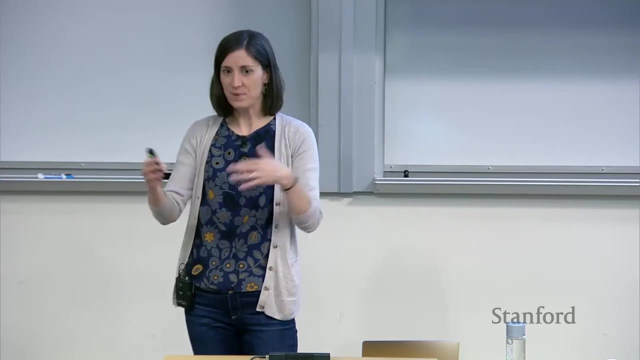 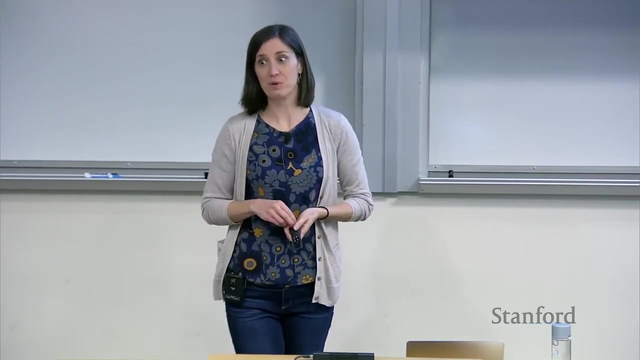 in sound. You're in a culture that does not rely on sound, that has developed other ways of communicating, other ways of just handling. you know awareness of behaviors in the world and states in the world, And so that could be one reason. 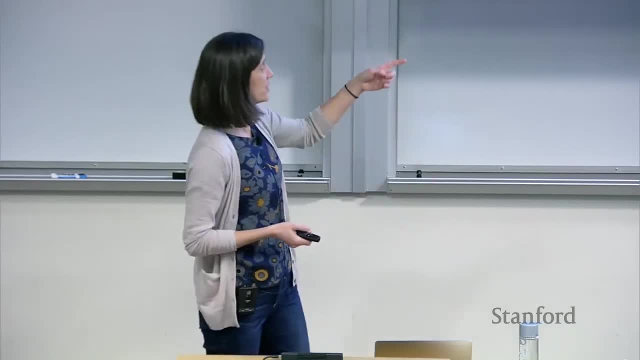 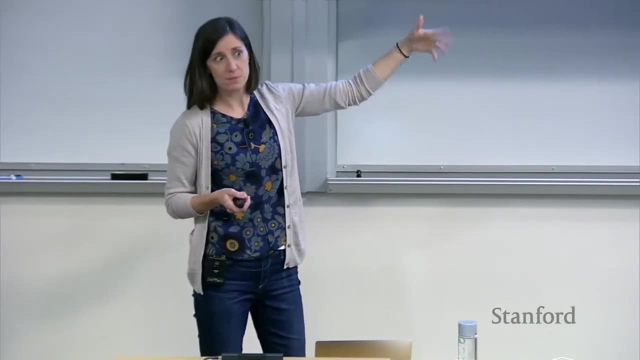 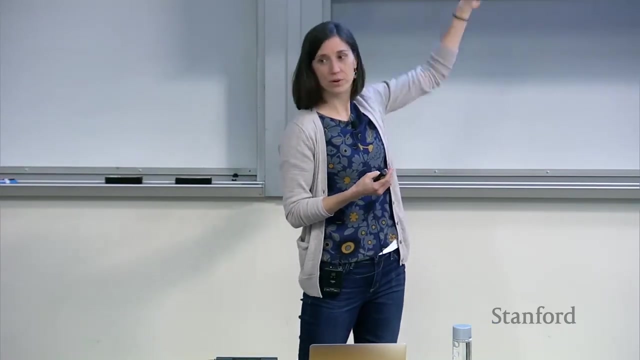 I mean there are some aspects of sound awareness that this group was particularly interested in, like real-time captions They were very interested in. the sign language group was Probably because spoken communication is more difficult for this group than for groups that had more that actually obviously preferred spoken communication right. 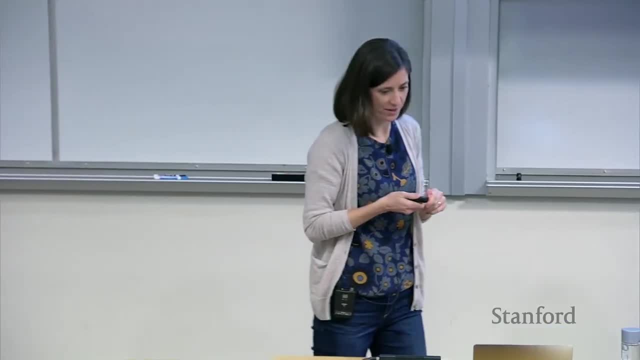 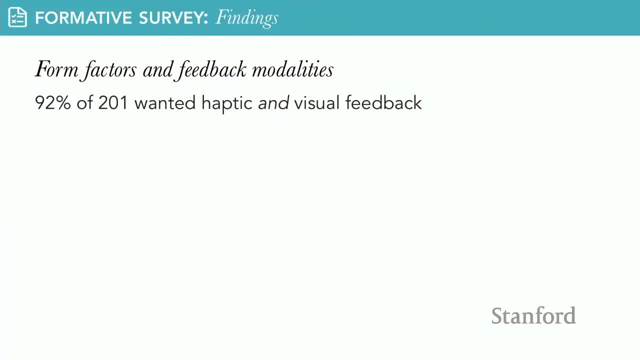 So anyway. so there are different. there's some different characteristics going on there. So, in terms of form factors and feedback, almost all participants wanted both haptic and visual feedback, And they most commonly wanted this when asked about an ideal setup on two different devices. 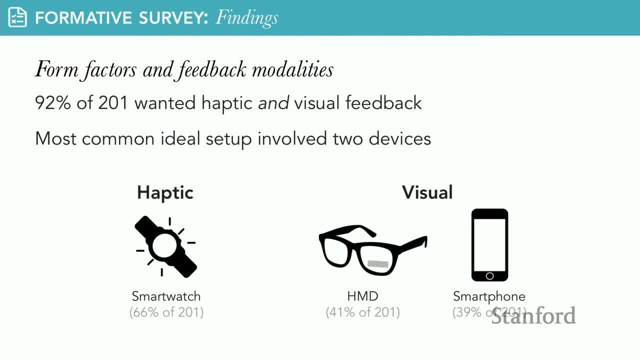 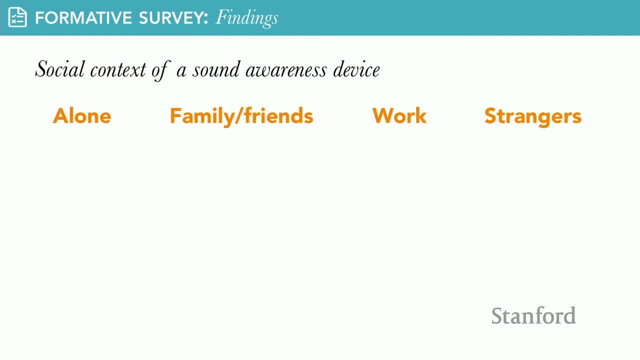 So haptic feedback on a smartwatch and then visual feedback on a head-mounted display or a smartphone. In terms of social context of use, we asked about four contexts. So use of a sound awareness device when you're alone, when you're with family or friends. 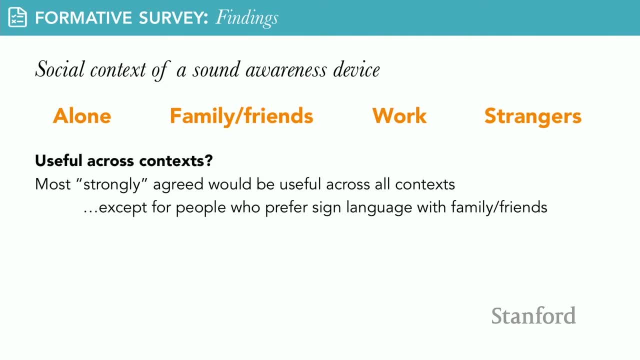 when you're at work or when you're with strangers, And most participants strongly agreed that a sound awareness device would be useful across all of these contexts. There's some indication that people who prefer sign language may find this useful. They find it less useful with family and friends. 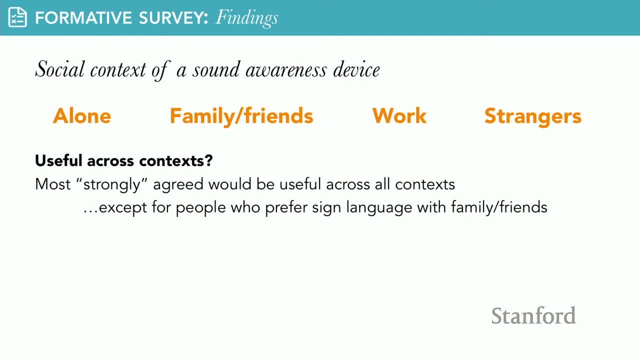 Again, perhaps because they're using sign language to communicate and may have some other sound strategies. don't need to rely on sound. In terms of social acceptability, did you have a question? Yeah, What does sound awareness mean? Sound awareness right means that if sounds are occurring around you, you're getting some. 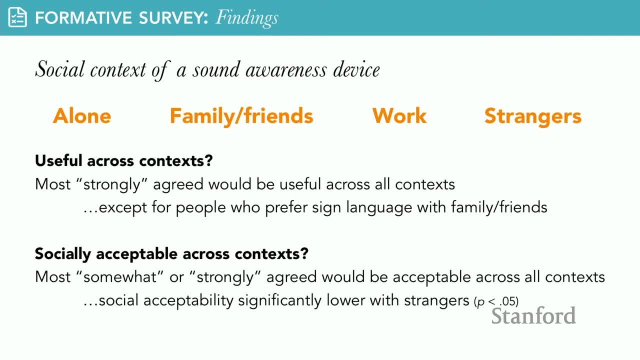 information about those sounds in some way that can allow you to act. But you know, if you're communicating with people or there's a door knock, What kind of awareness do they need then? Do they want Right? Well, so there's so a few slides ago I had some and I went quickly over this, but we 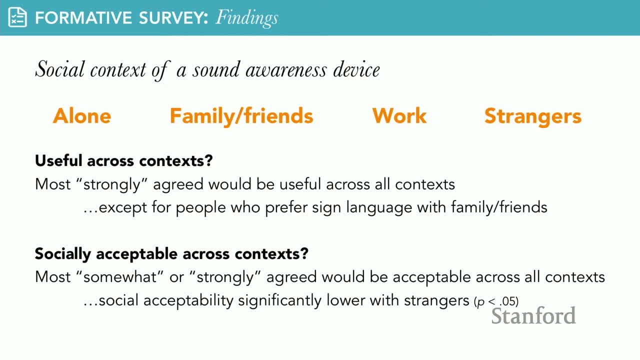 had asked people about the different sounds that they were interested in, And there is some. in general, there are clear indications that, like urgent alerts and voices directed at you, Those are things that everyone wanted to know about. But there is some difference in terms of especially these three communication groups. 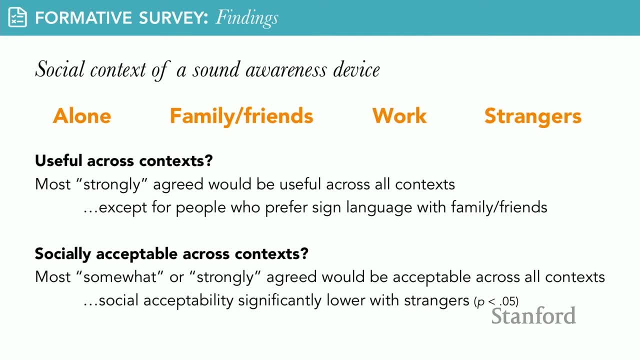 in terms of some of the other sounds. once you get into things like mechanical background noises inside or birds chirping and other nature noises, Like there are some differences there. I mean, I think there's this. if you step back and think about it, there's this bigger. 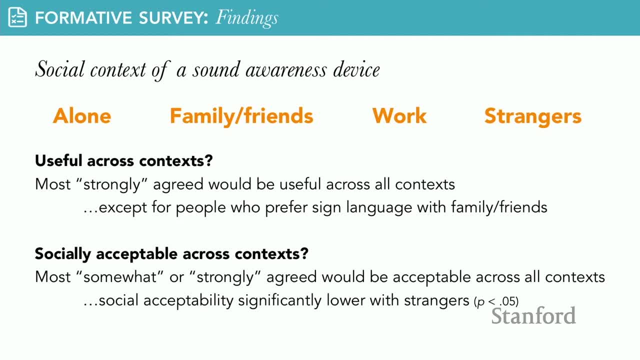 question of what, why, what's the purpose of sound awareness? It's actually to understand something about what's going on in the world, And so you know- maybe you want to know- there's a bird chirping. You don't need to know that there's a sound of a bird chirping. 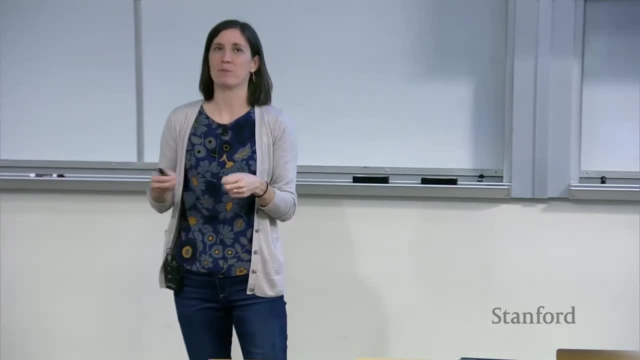 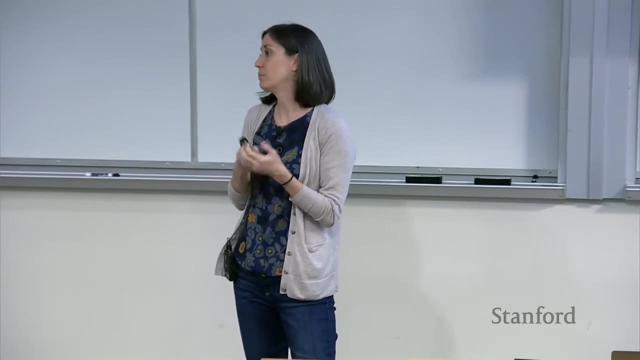 You know, somewhat nuanced, but you could imagine if you had a system that could know all of this stuff, that there might be that people would know. There might be that people some people might prefer might not be like. I do not. 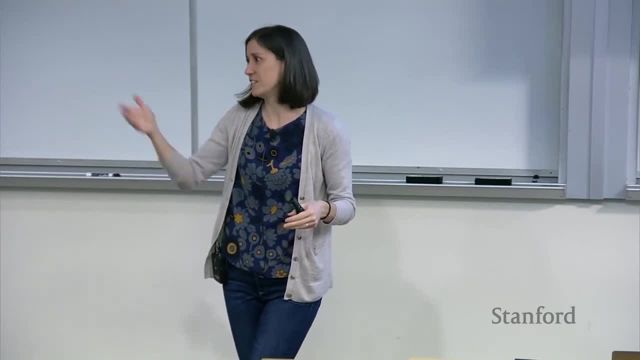 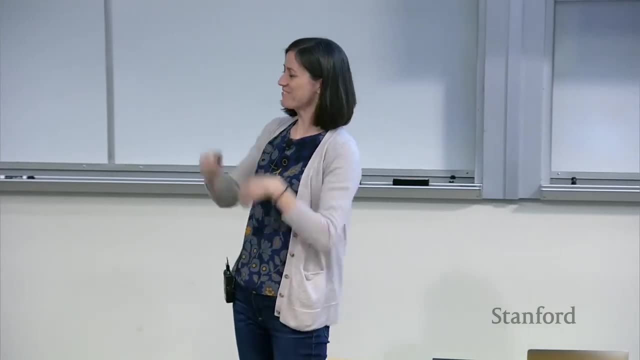 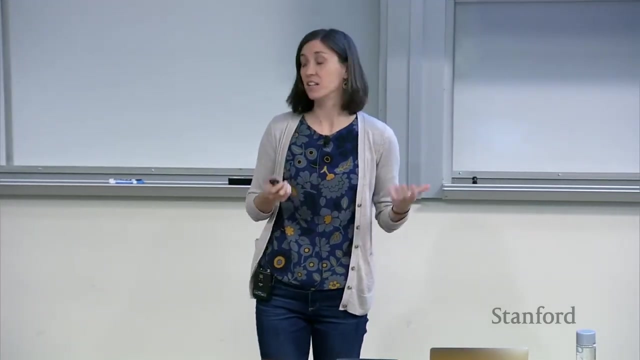 care about the sound at all. I just want to know what the thing is that's happening, And the sound is just one way of getting at that. So, anyway, I think there's more to understand here, And I don't know that there are big differences that were evident in this study in people. 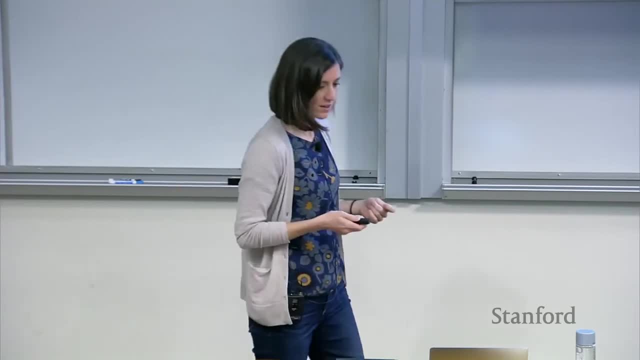 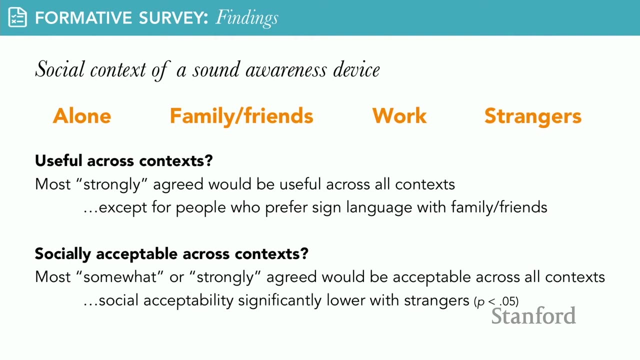 interpreting what sound awareness is differently, though. Did I mention the social acceptability thing, Okay, So the main significant difference here is that there was lower, significantly lower, social acceptability when considering use of a sound awareness device around strangers than in the other three contexts. 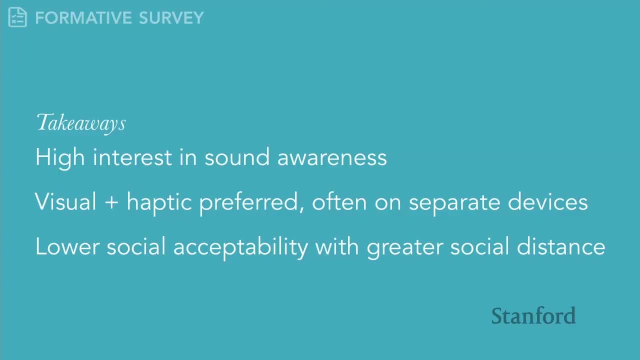 So takeaways for this study include high interest in sound awareness, preference for visual and haptic feedback, often on separate devices, and then lower social acceptability with greater social distance. So now I want to move on to supporting spoken social interactions. 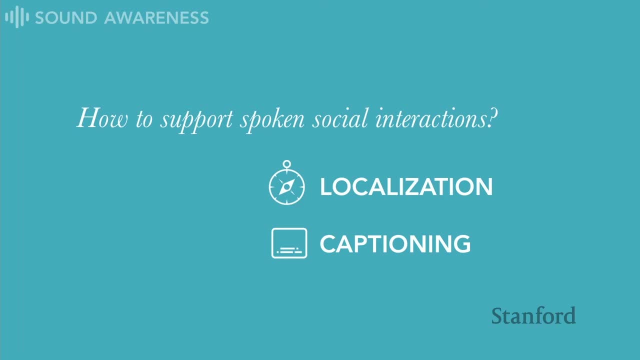 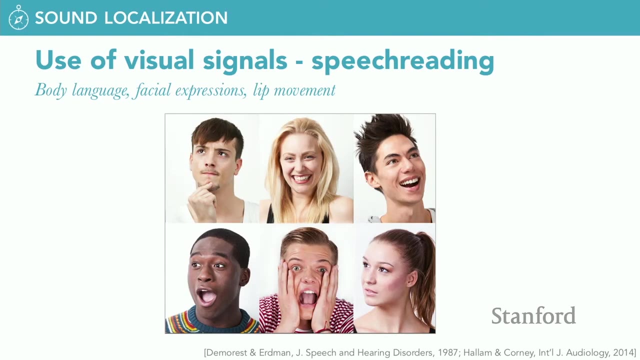 And we've looked at this in two ways: providing localization of sound, so where sound is coming from in a room, and then real-time captioning, So for localization. people who are deaf or hard of hearing make use of visual cues when they are engaging in spoken conversation. 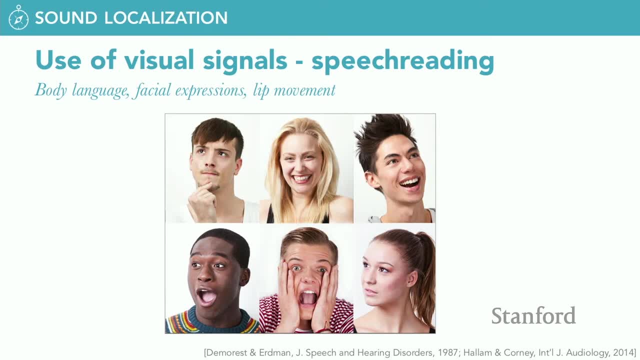 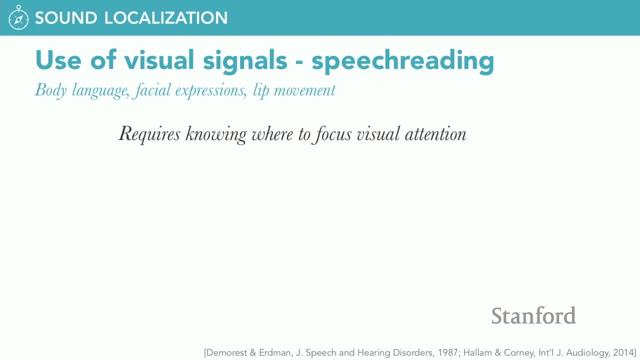 So this is called speech reading or lip reading. So body language, facial expressions, lip movement and so on. But being able to make use of those cues requires knowing where to look. So here's a quote from one of our participants, for example. 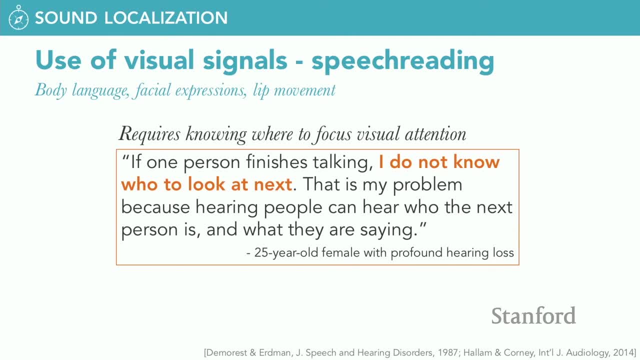 If one person finishes talking, I do not know who to look at next in a group conversation setting. That is my problem, because hearing people can hear who the next person is and what they are saying. So our approach is to visualize sound on a head-mounted display. 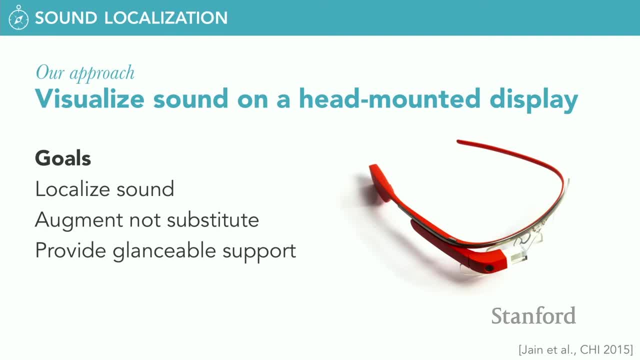 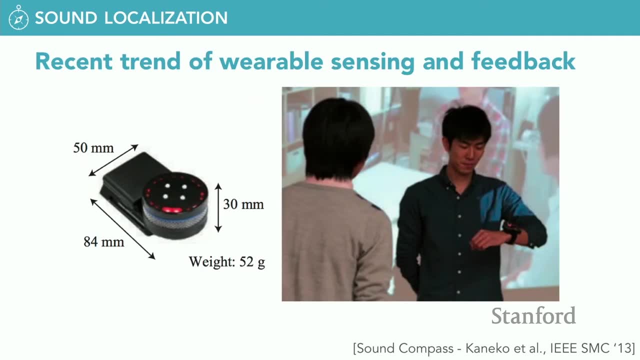 We want to localize sound augment, not substitute the user's existing sound awareness strategies and then provide glanceable support. So there's some recent work, a recent trend of providing this localization of sound, This localization of sound on wearable devices. 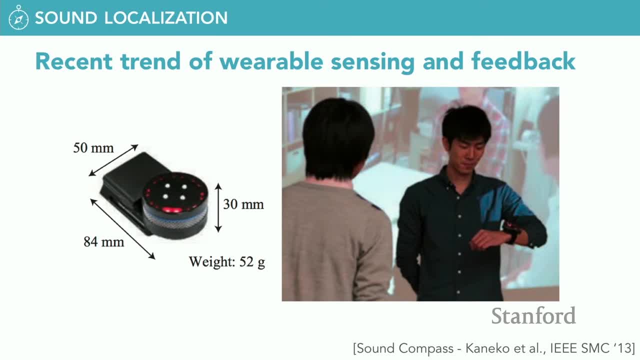 And what you see here is a wrist-worn device that provides sound feedback in four directions. One issue is that you need to look away from your conversation partner in order to make use of that information. So imagine you are wearing our head-mounted display. 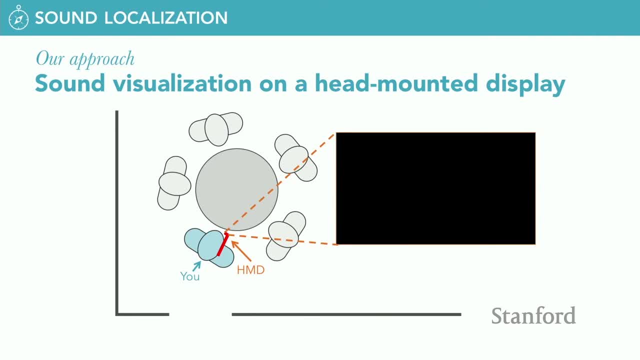 You're sitting at a table with a bunch of other people and then someone to your right talks. A sound visualization shows up on the right of the device, the display. Someone across talks. That shows up at the top of the display, And then someone comes in the room behind. 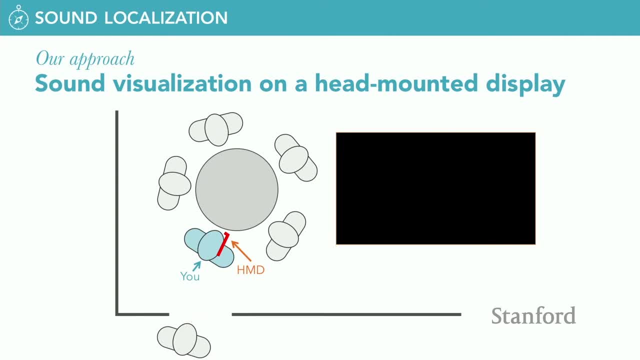 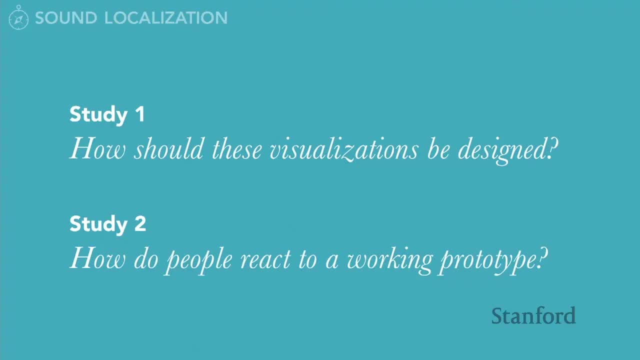 And that shows up at the bottom of the display. So you can imagine designing these visualizations in many different ways. and what kind of information do you present additionally, and so on. So that's the first thing that we looked at. 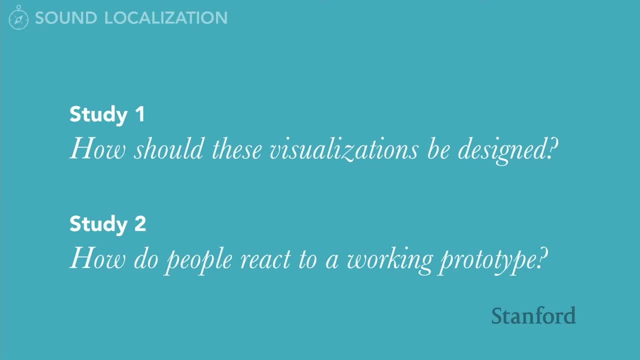 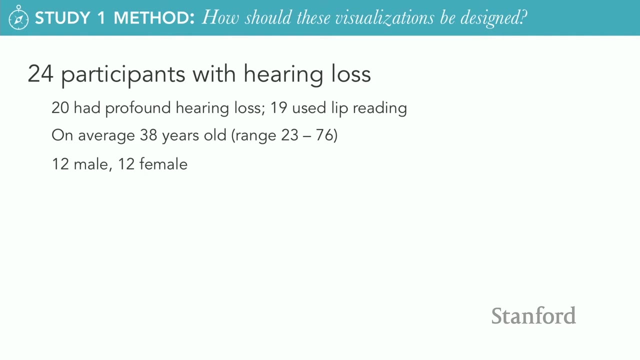 And I'm also going to talk about a smaller second study where we built and evaluated a working prototype. So let's start looking at the design of these visualizations. In this study, we recruited 24 participants with hearing loss. They completed semi-structured interviews. 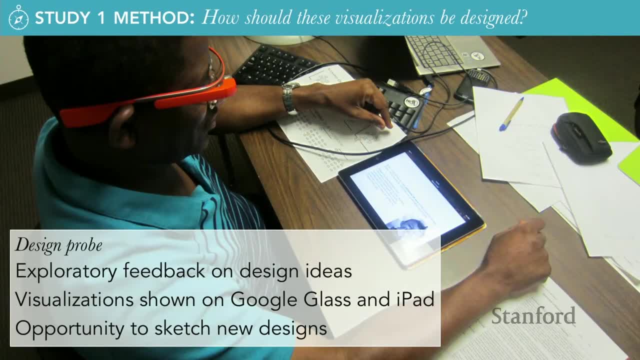 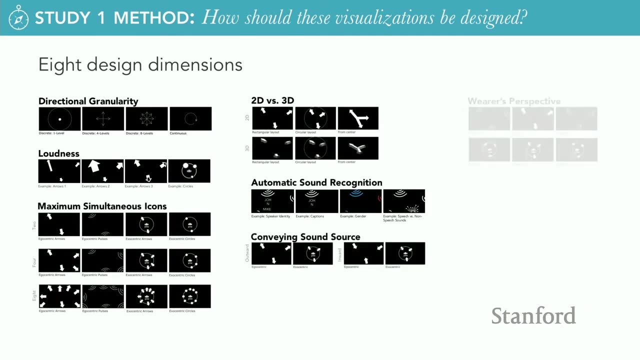 And we used a design probe to elicit exploratory feedback on design ideas. Here we showed visualizations on Google Glass and on an iPad And participants had an opportunity to sketch new designs. So we looked at eight design dimensions. I'm not going to describe them all in detail, but I'll give you one example which is directional. 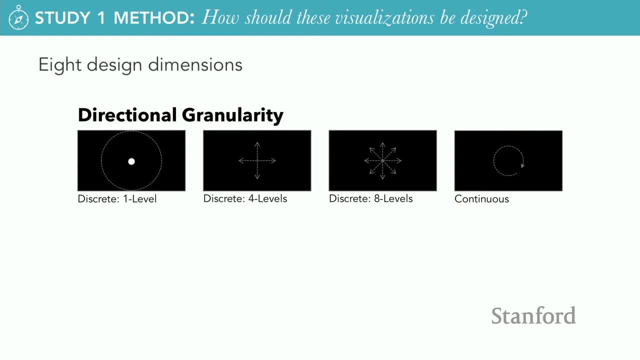 granularity. So here we had four levels of directional granularity, from simply a sound occurred or not To continuous directional granularity. And there are implications here both for in terms of utility and possibly cognitive load, with the higher information granularity conditions, As well as for the sensing hardware. 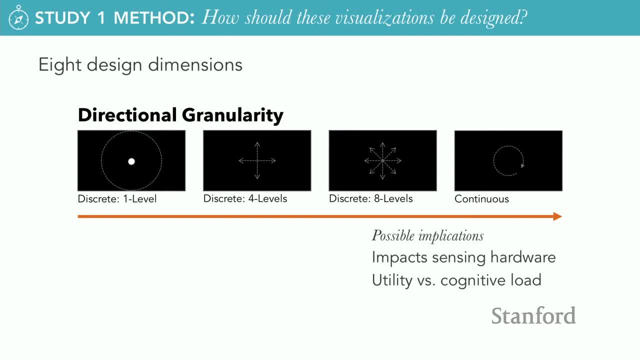 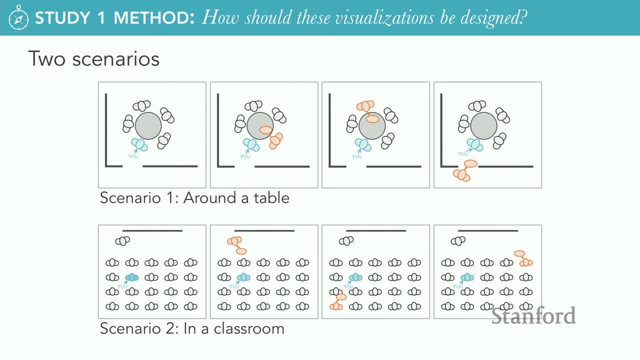 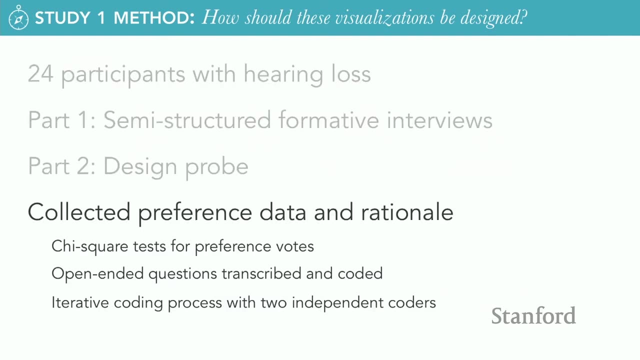 So if you don't need, if you need less precise directional granularity, then you can use fewer microphones, for example. We evaluated these ideas within two scenarios- This around the table conversation scenario and a classroom setting- And then we collected preference data, votes as well as open ended rationale. 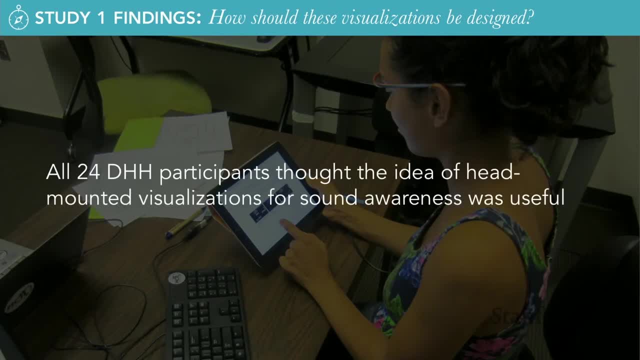 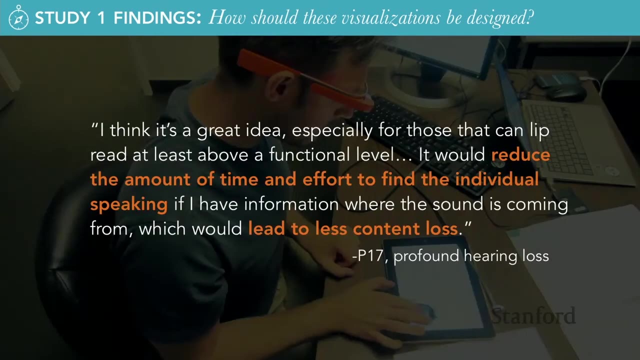 So an overall finding from this study is that all 24 of the participants thought the idea of head mounted visualizations for sound awareness was useful. So this is reflecting some of the earlier findings as well, But focused on head mounted displays. Here's a quote from one participant with profound hearing loss. 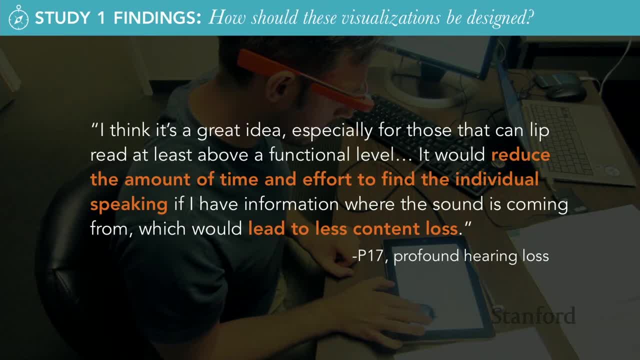 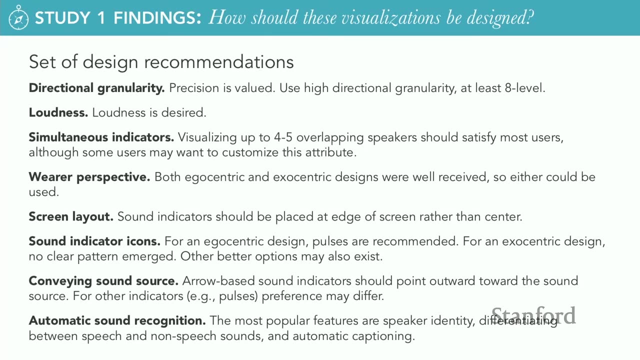 I think it's a great idea. It would reduce the amount of time and effort to find the individual speaking and would lead to less content loss, So this emphasizes increased efficiency as well as more meaningful communication. potentially Another outcome from this study is this set of design recommendations. 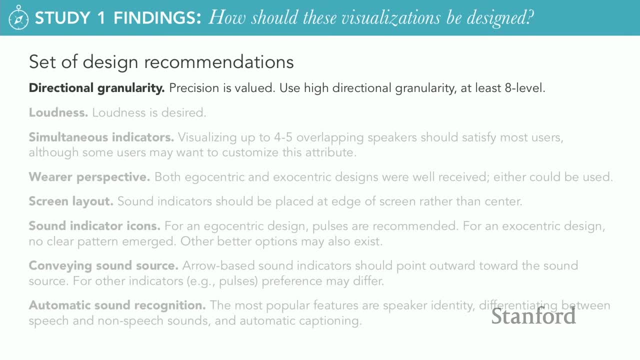 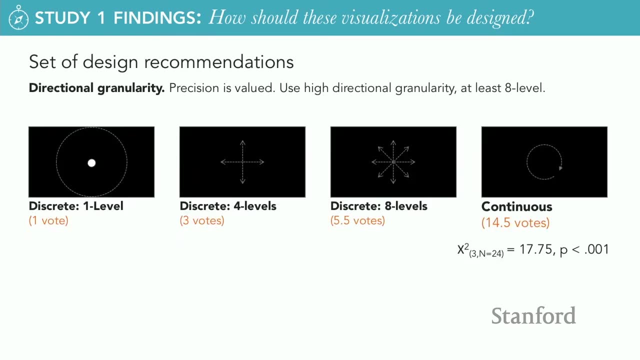 And so these are based on those preference votes. So, for example, for directional granularity, precision is valued. Use high directional granularity, And this is based on the significant difference in terms of those preference votes. And some of the open ended rationale that people provided were, for example, the more 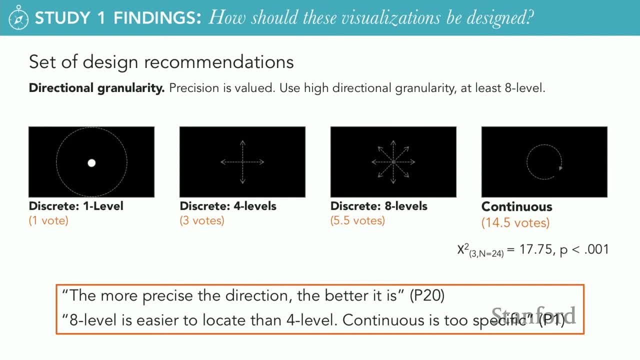 precise the direction, the better it is. And then also some comments that reflected the potential tradeoffs with cognitive load and higher precision. Eight level is easier to locate than four. level Continuous is too specific. I think there's some open questions there about what we actually want to do with a working 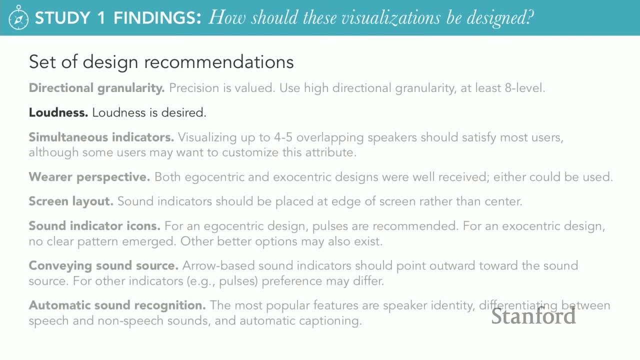 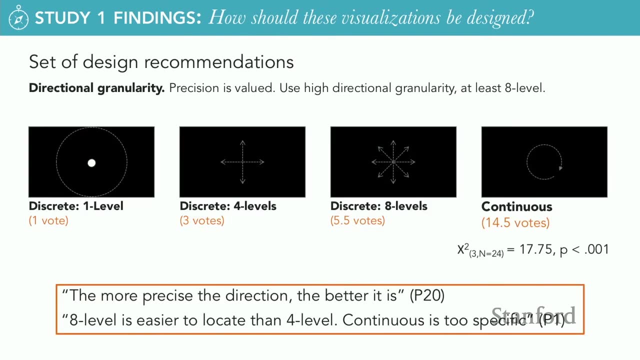 system. So another example is that participants were interested. Yes, Do you know? when someone picked one level, did you look at their rationale? Yes, we did Well because? so what we did was, in our analysis, we focused on the quantitative preference. 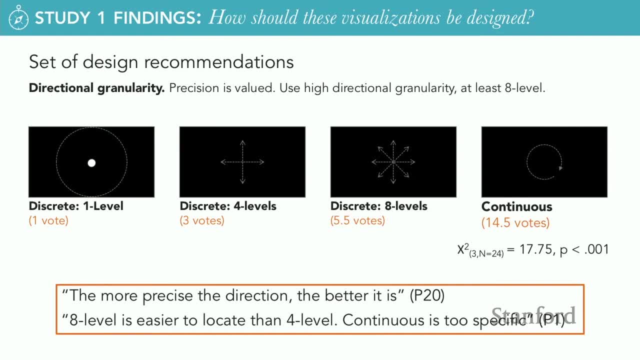 votes first, And then we sort of grouped together. you know why. what did people say? who preferred this level versus? and then what did people say who preferred this level? And I don't remember all the details from the rationale, but this quote here the more. 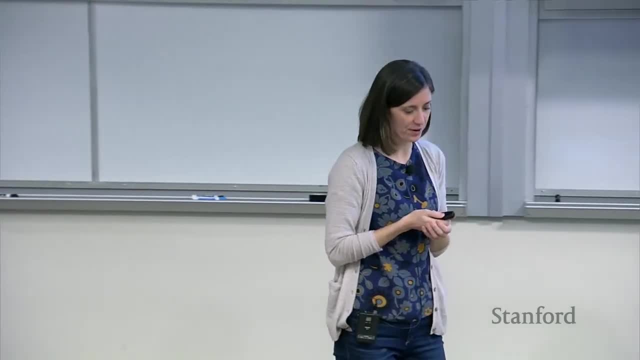 precise the direction, the better it is, is representative of the eight direction and continuous preferences, Which was the by far the most common kind of sentiment. Yeah, Well, yeah, I don't remember the details on that, Yeah. 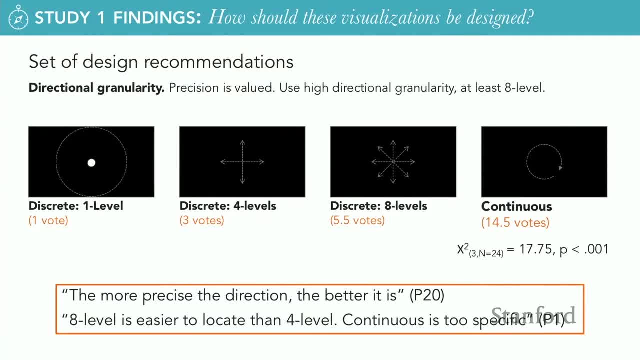 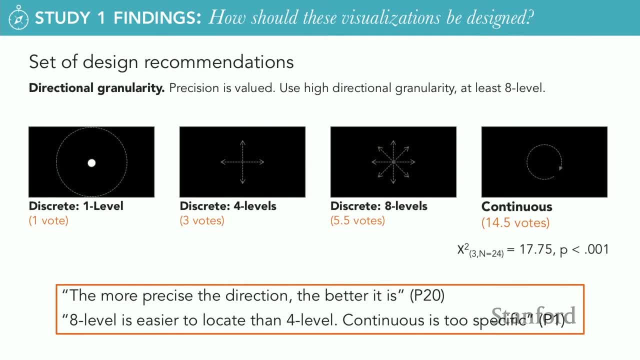 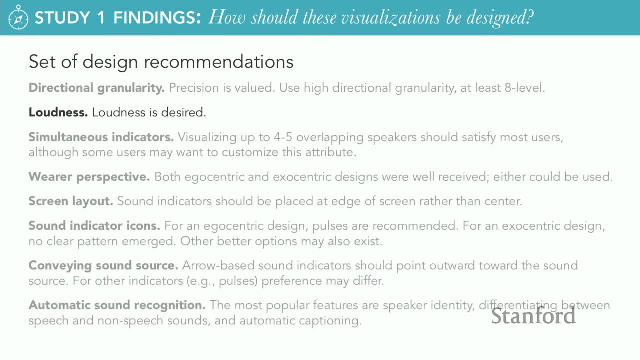 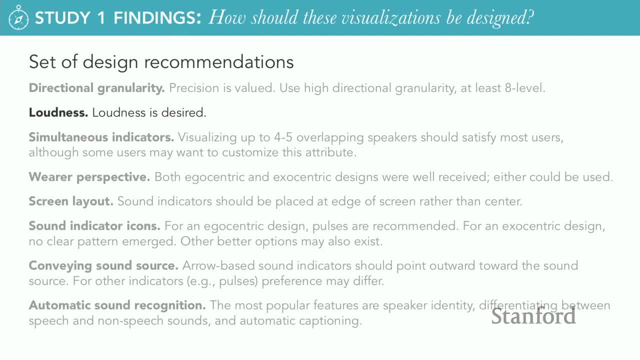 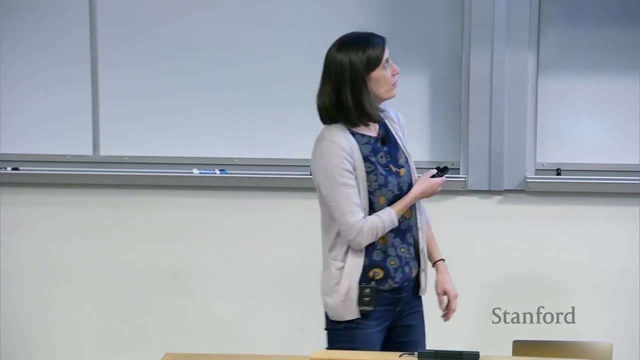 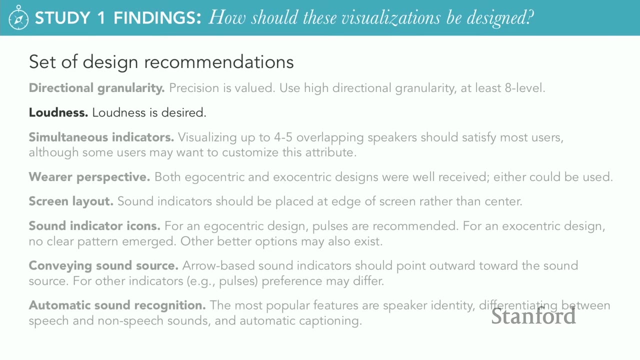 to which how precise you want them to be visually indicated Right, Or how do you localize the sound with any precision. So we didn't do that at all in this study. This was just about showing design methods, design probes, but I will come back to that question in a little bit, okay. 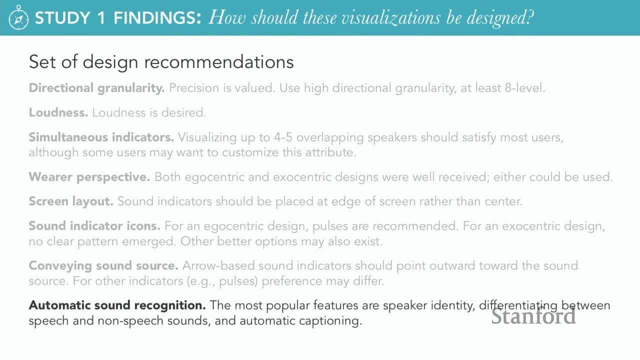 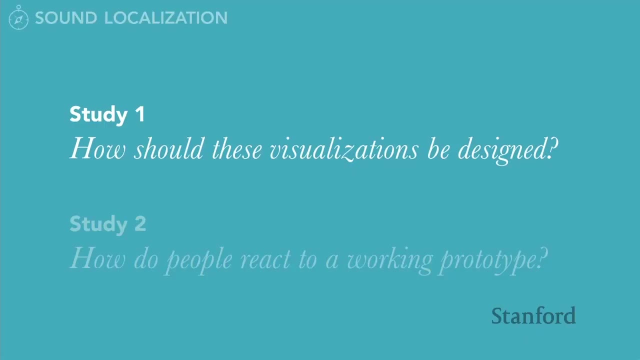 Okay, so loudness is also desired, so magnitude of sound in addition to direction, and then more advanced features like automatic speech recognition- just differentiating between speech and non-speech sounds, for example- were also highly popular. So I'm gonna come back to captioning actually shortly. 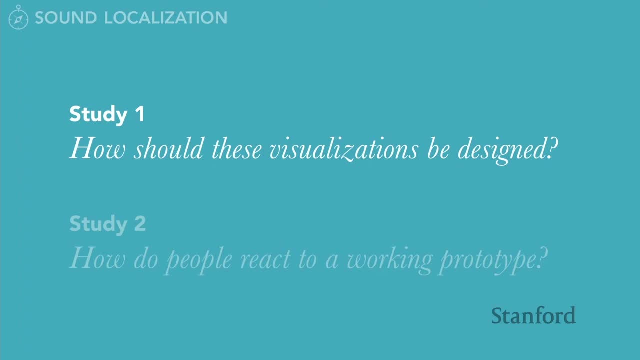 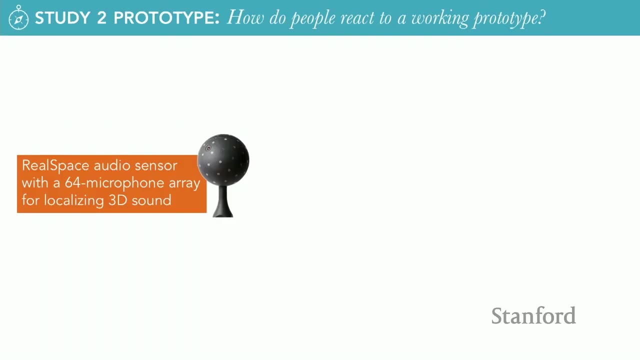 Okay, so once we, building on these findings from this study, we then built a working system which we evaluated with a smaller number of participants. So here is to answer your question. what we had done at this stage was we used a non-wearable 3D sound sensor, which, yeah, which is? 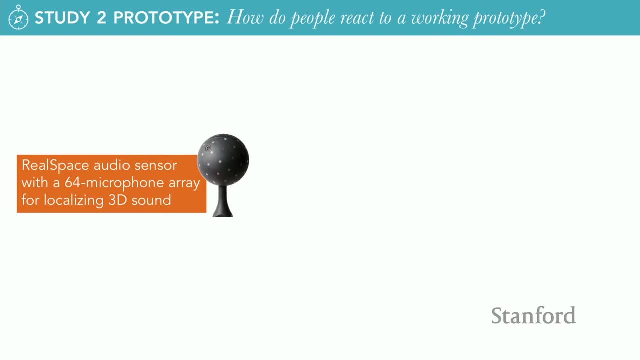 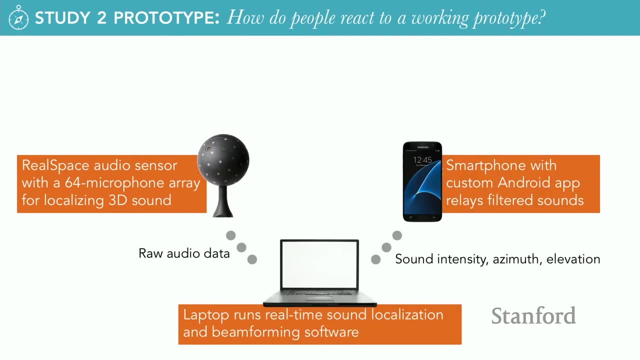 it's about the size of a head. that's true. it looks like the Death Star. This is developed by one of our collaborators, Ramani Dharaswamy, at the University of Maryland. Anyway, we connected this to laptop and a smartphone and then the head mounted. 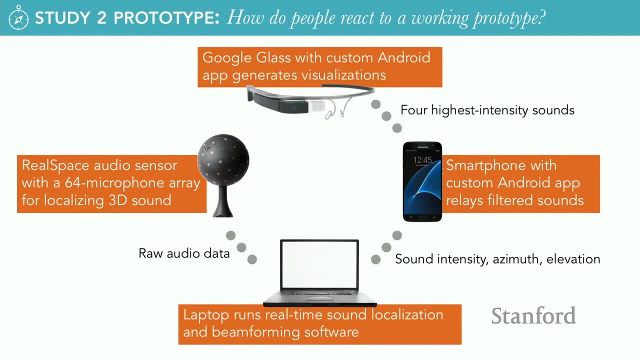 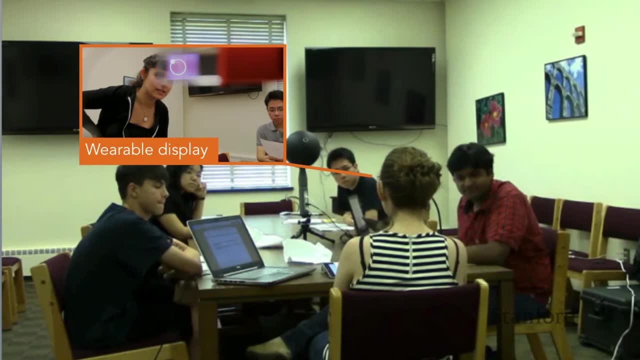 display and then we could actually visualize the sound, We could actually visualize the location of sounds in a room. So this is the setup for this particular study And, again, the non-wearable sensor was fine for at this stage in the research. 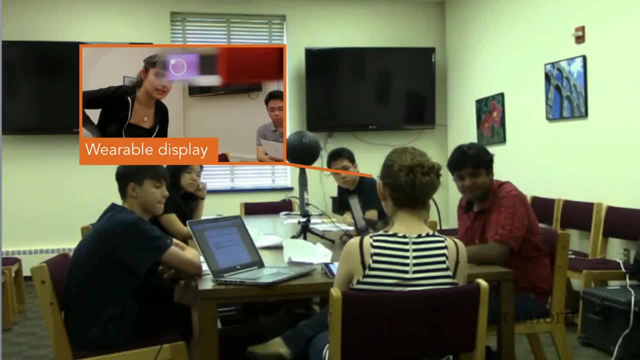 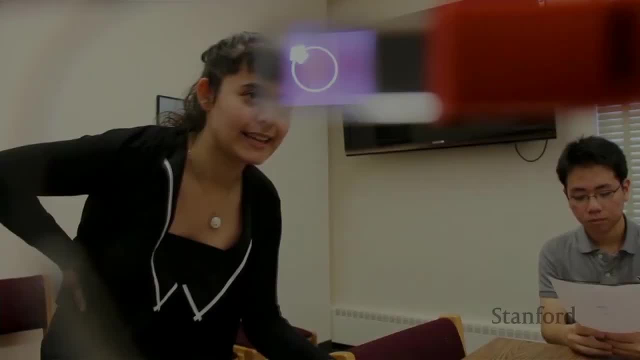 but we are working on a wearable version right now. So here's a participant sitting at a table wearing the head mounted display and some research assistants around the table, And this is how the display looked. So there's an arrow here that's gonna move around as different people talk. 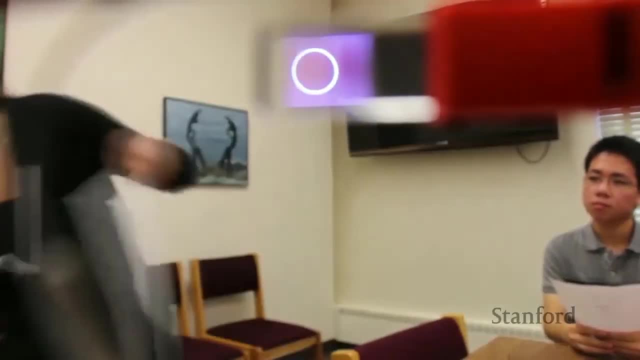 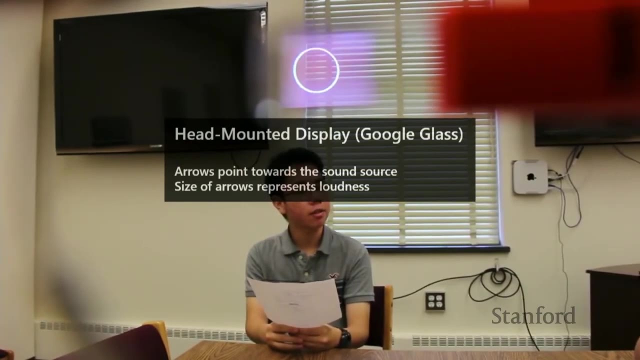 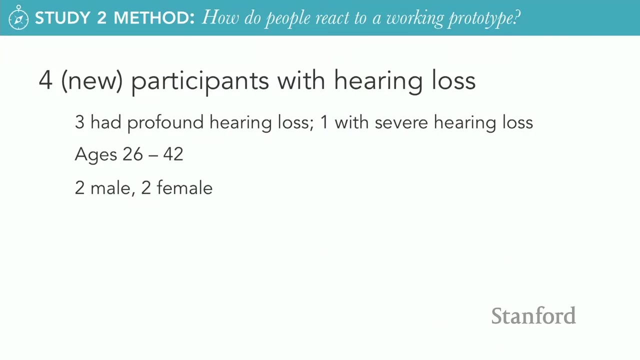 But I'll be right back in case you need me. I just realized something: We've never had a completely successful test with any of the equipments. I blame myself, How do I? Okay, so we had four new participants with hearing loss. use two of the designs. 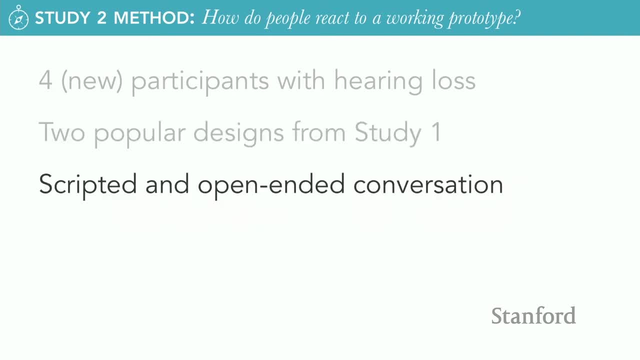 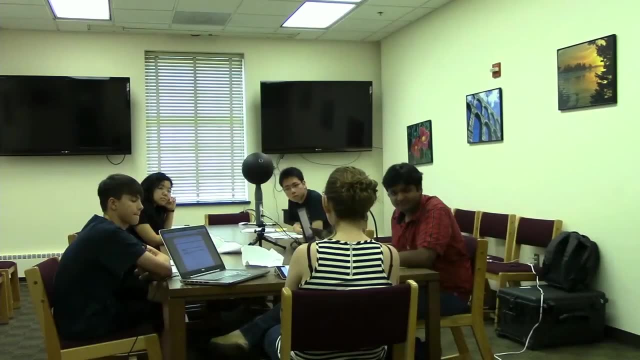 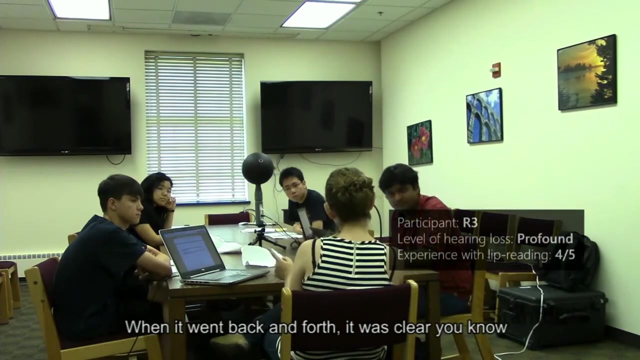 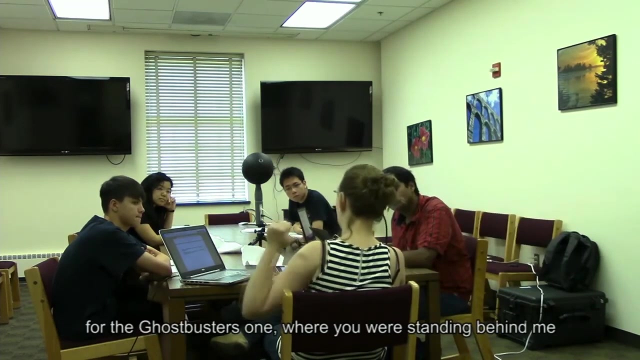 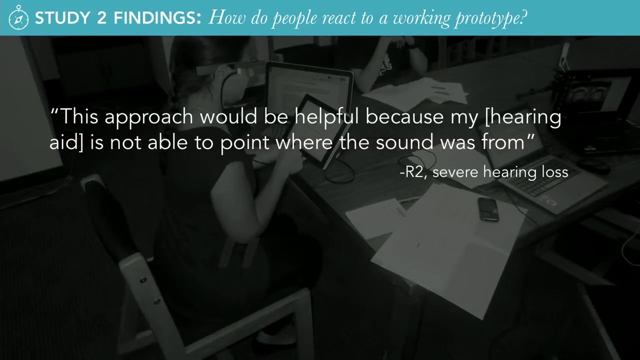 that were most popular from study one And participate in scripted and open-ended group conversations with those research assistants. Now here's a quote from one of the participants on the experience of wearing the device when someone walked behind her and spoke. So in feedback in this study we saw some positive reactions as well as some concerns. 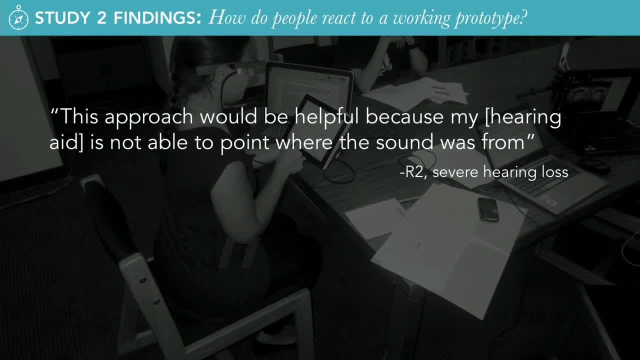 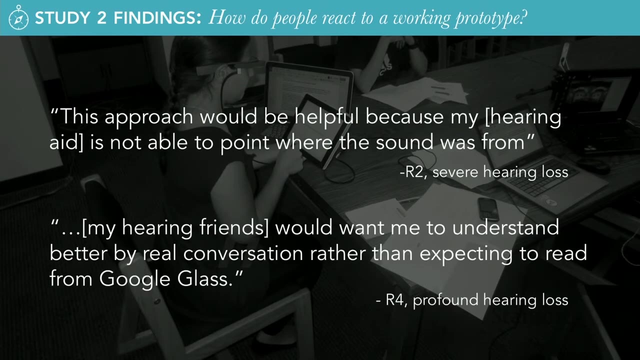 So, for example, this approach would be helpful because my hearing aid is not able to point where the sound is coming from, so that localization advantage. And here is a question, A question about whether technology mediated communication is always appropriate. So in this quote here, my hearing friends would want me to understand better by real 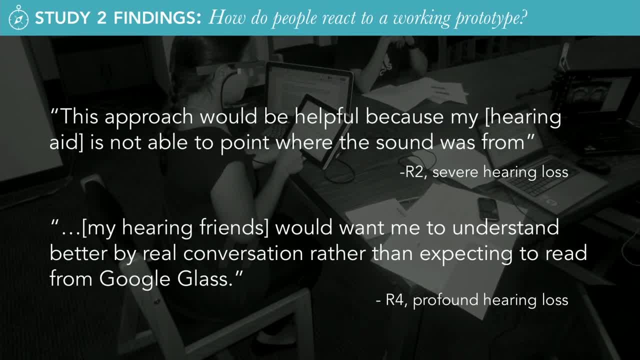 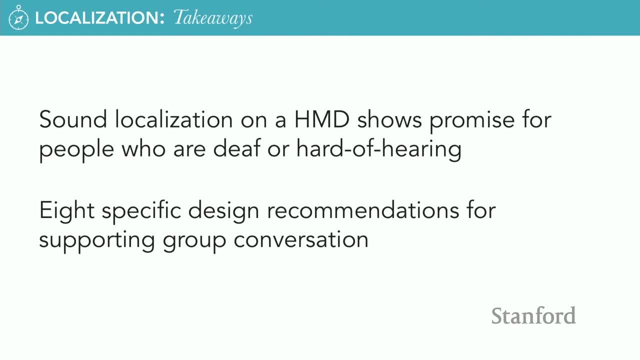 conversation, rather than expecting me to be looking at Google Glass. Okay, so some takeaways from here are that sound localization on a head mounted display shows promise for people who are deaf or hard of hearing, And we have eight specific design recommendations that deserve some further. 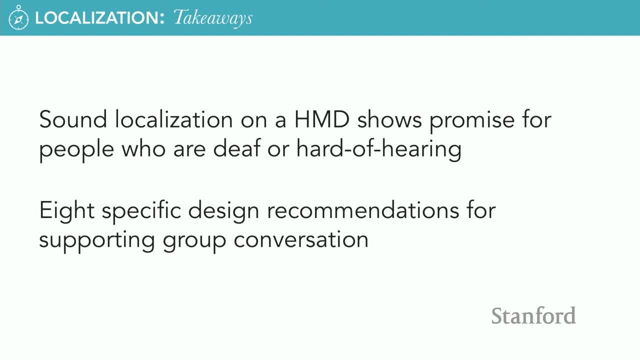 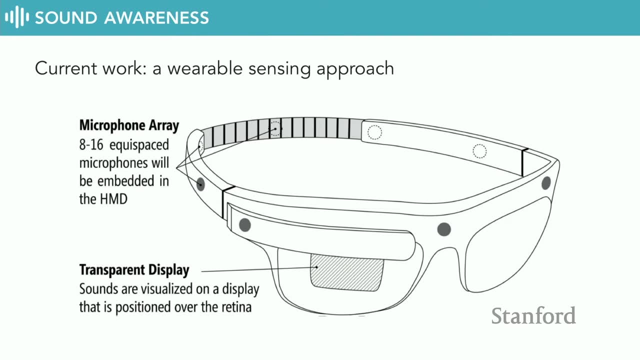 attention with In in further work with a working system, And then currently we are working on a wearable sensing approach. Again, this is with Romani Duraswamy at Maryland, And did you have a question? Yeah, Well it. this may be a limitation of current technology, so 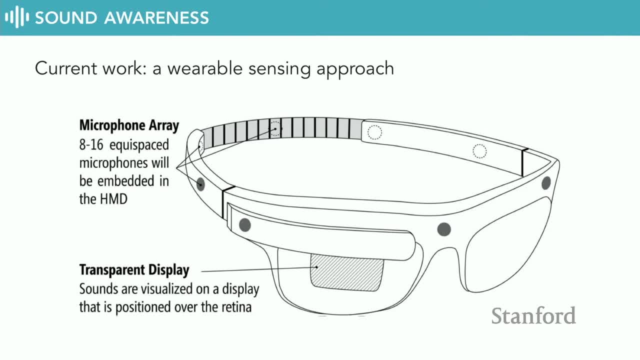 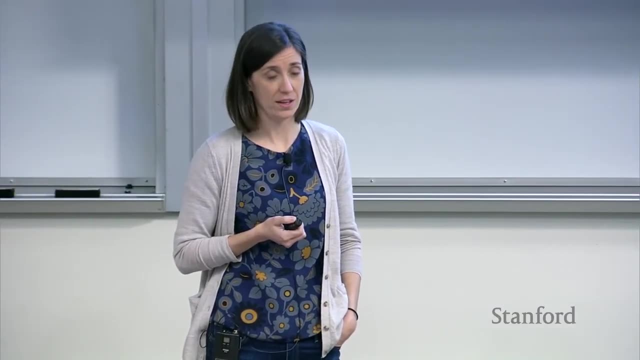 I'm wondering if you think it is or not. My experience with folks who wear hearing aids is that by sort of making everything louder, it also inhibits my ability to sort of focus on particular parts of the conversation in a loud room, And I'm wondering how many sort of false positives this kind of thing would run. 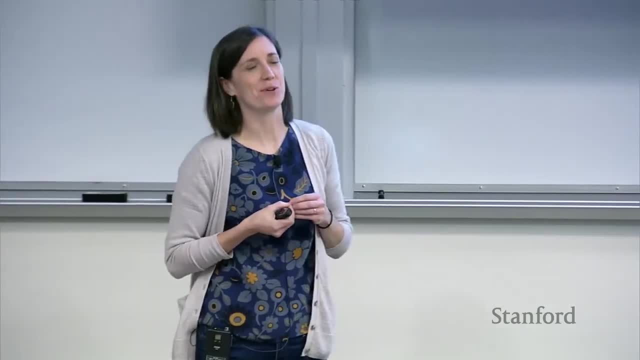 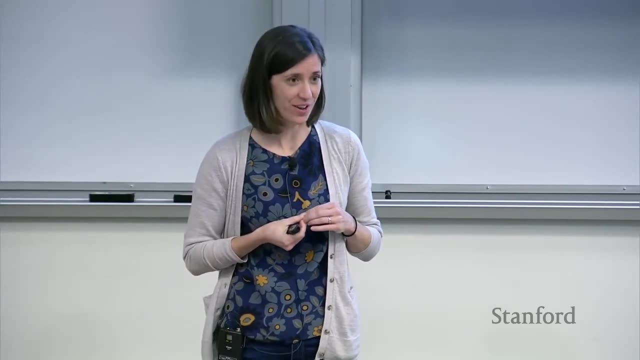 into as well? Right, yeah, I think there are. so actually we just got an NSF medium on this project. So there, because there is a lot to to that, we don't know about how to do this. I mean, what sounds do you filter out? 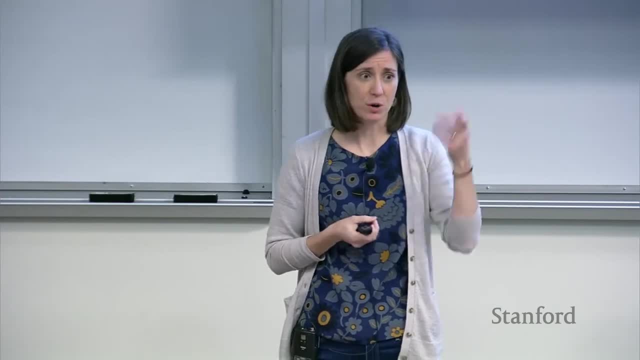 Could we just filter based on loudness? Do we need to know something about identity? Do we show the louder sounds in a different way than the quieter ones? Do we just show speech because you're in a conversation? Do we eliminate all the nonsense? 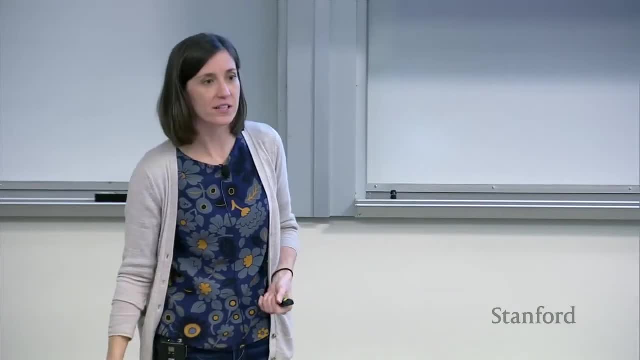 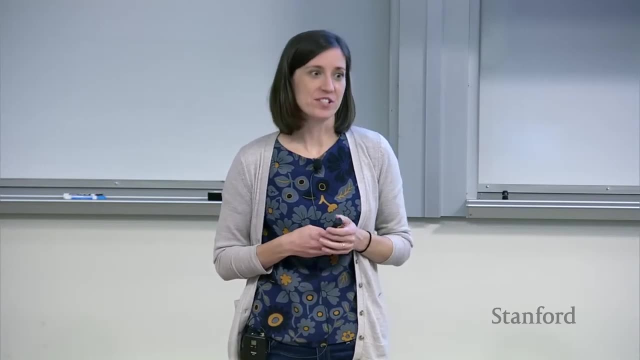 Do we eliminate all the non-speech sounds In the? in our study? actually there was some paper rustling and one of the participants said: I want to know that, even though it's a conversation. So there there are lots of questions about how do you actually do this feedback. 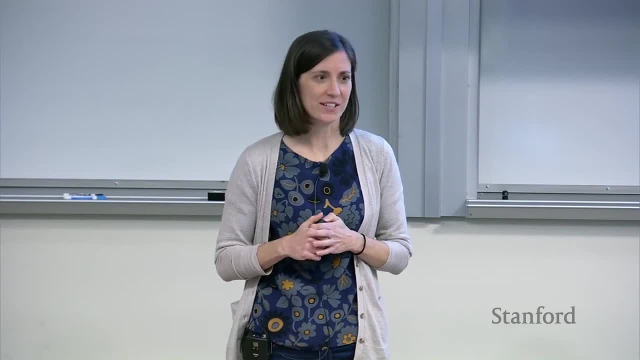 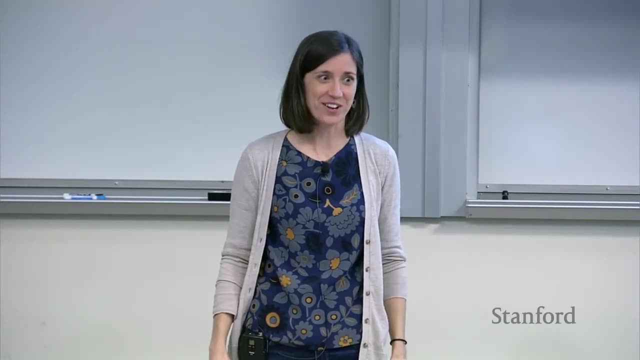 in a way that is not, that is useful and not overly distracting, And that probably changes based on context. and how does that work There? yeah, lots of great questions, Yeah, Okay, and also with the next thread of work, that is this: 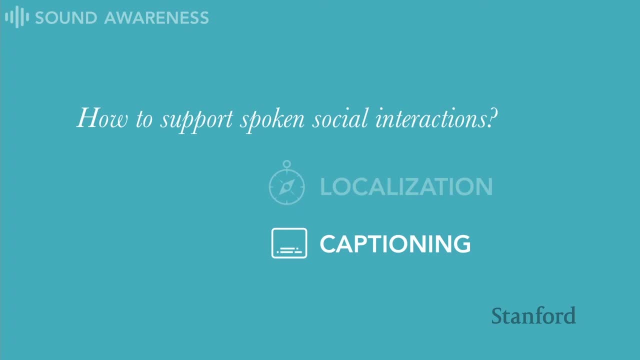 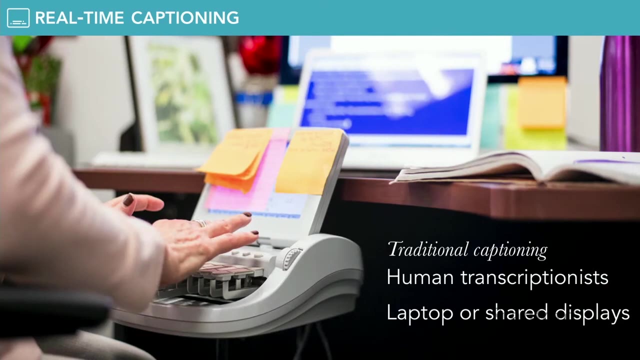 that's the case too. Okay, so this thread of work we are looking starting to look at real-time captioning on a head-mounted display. So traditionally real-time captioning works with a human transcriptionist and then captions shown on a laptop or a shared display. 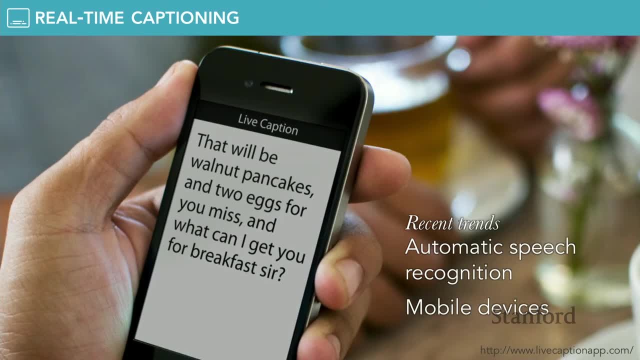 We're seeing more and more use of automatic speech recognition these days, And this is actually good enough that this is useful in many situations. Also not useful in many situations and can lead to miscommunication, And it's not as good as human transcriptionist. 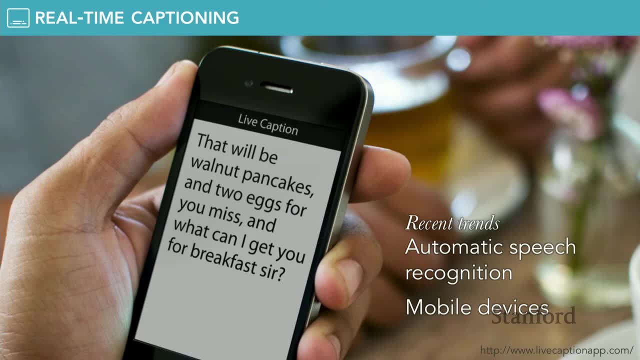 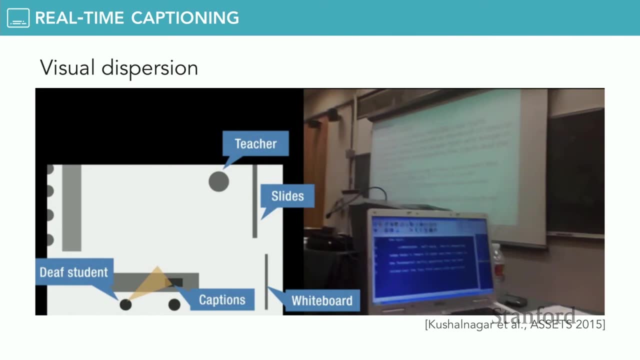 But? but it's an exciting development. And then also more applications on mobile devices. Now, regardless of whether using a laptop, a shared display or a mobile device, an issue that can arise is visual dispersion, And this is a picture from Raja Kashalnagar, one of my collaborators on 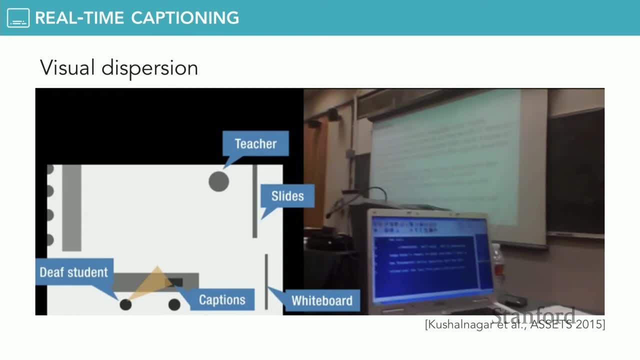 this project at Gallaudet University showing captions on a student's, captions on a laptop for a student in a classroom, Slides shown at the front of the room. There's also a teacher, someone there in the room. There are other students. 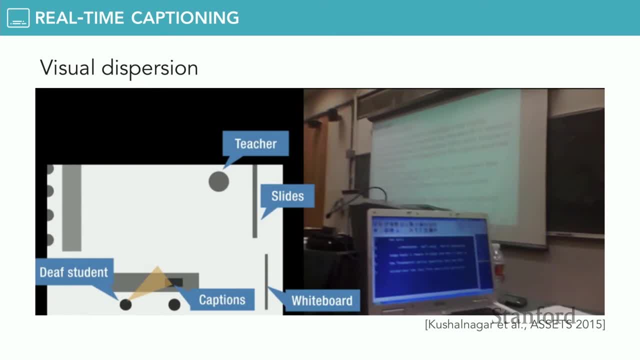 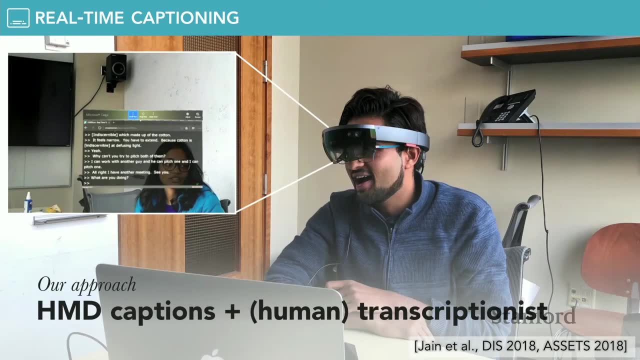 This student themselves probably has a lot of experience. This student probably has a laptop or a paper where they're taking notes, So the captions are just adding to this visual load. So what can head-mounted display captions do to possibly reduce this visual dispersion issue? 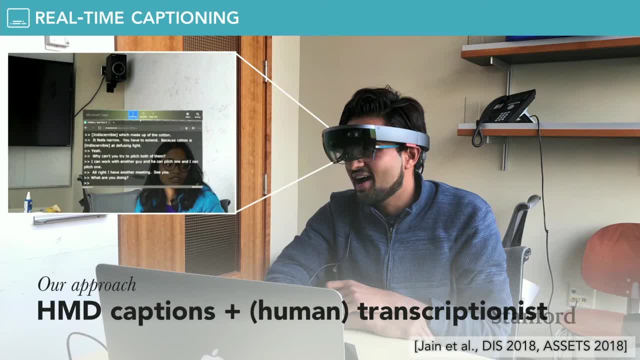 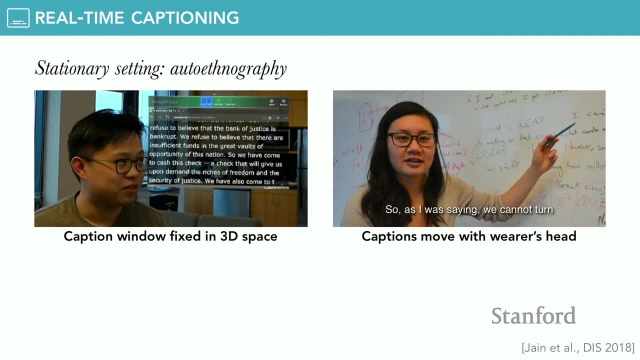 So in this work we've been using Microsoft HoloLens And we've conducted a few studies so far. So the first one is an autoethnographic study in a stationary setting, And here we looked at two early captioning designs. 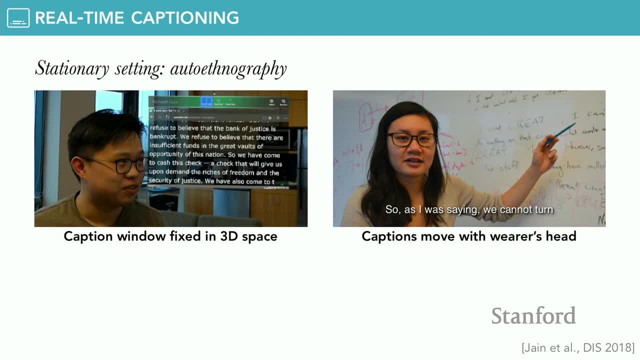 So one is a window where the captions show up and you can move that window around and place it, attach it to physical things in the room. You can also resize it and you can duplicate it, So I could put one over each of you know several people's heads. 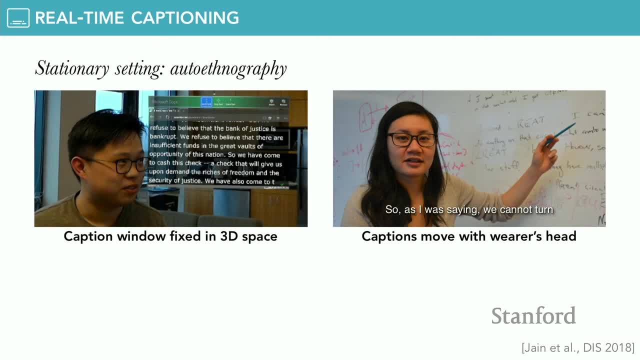 And then the second one is a simple one line caption, but that moves within your field of view. So our first author on this project, Drew Jane. he's a student at UW, He's hard of hearing and he used this system for seven meetings and 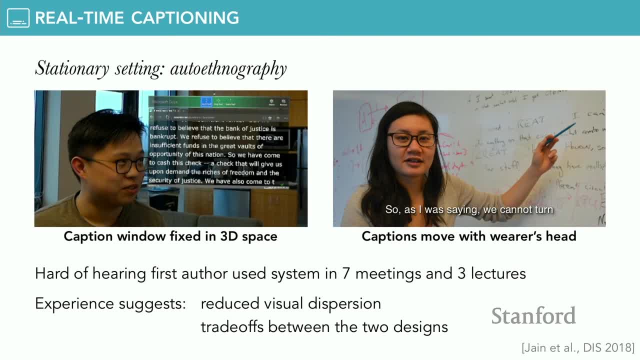 three lectures in a quarter where he was also using laptop based captioning, in other, like in the classroom, His experience suggests that he did feel that there was reduced visual dispersion with the head-mounted display than with the laptop And that there were trade-offs between these two designs here. 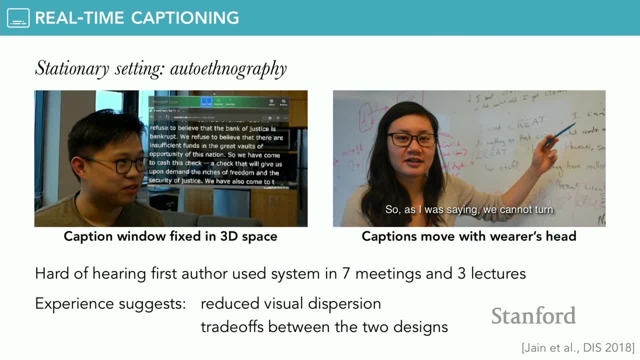 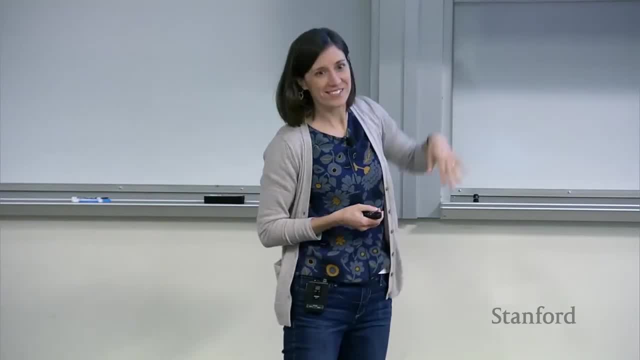 So, for example, with the 3D the design you could put a fix in 3D space. he would use it to maybe put below the slides or on top of the instructor's head And then that way they wouldn't get in the way of the slides or 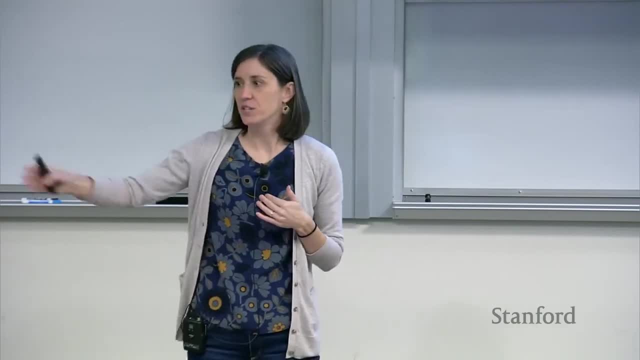 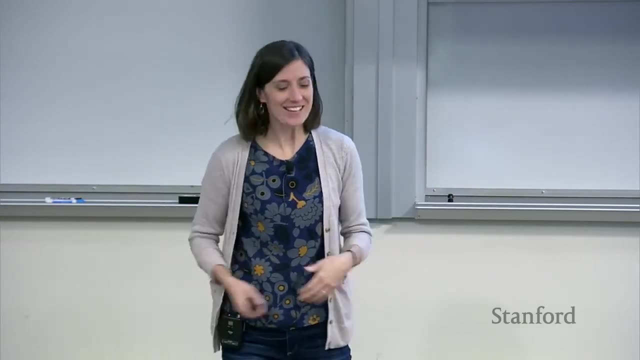 in the way of the instructor's face, But then, when he was in situations where the speakers were moving around more than the other, design was more useful. And before I get any questions on it, yes, the HoloLens is not comfortable to wear for long periods of time. 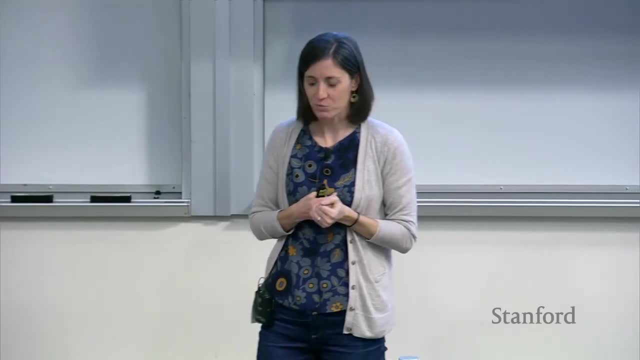 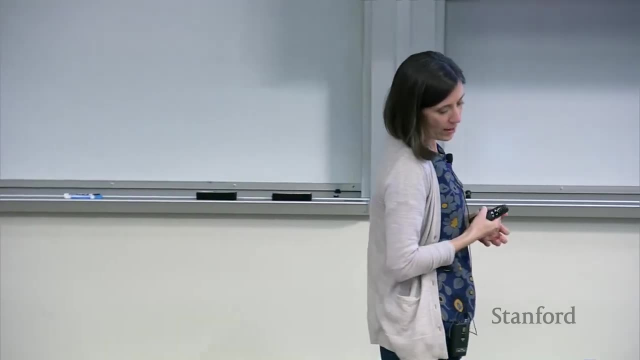 So that was one of the outcomes from his ethnography as well. So he tended to wear it for about 30 or 45 minutes and then really wanted to take it off. So in follow-up work we refined the system and evaluated it in a mobile. 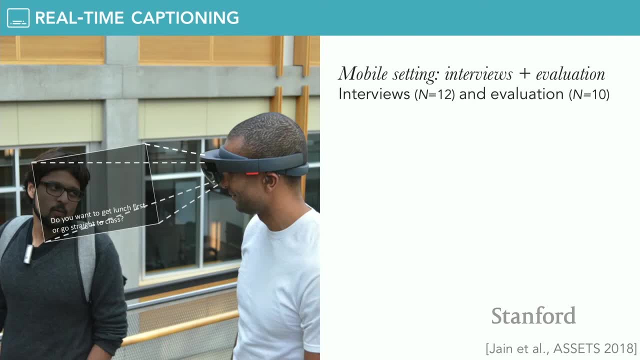 context where visual attention is extremely important for understanding Your environment and make sure you don't trip, for example. One of the motivating findings from this particular study is that participants felt that mobile conversations are especially difficult because if they look away from their conversation partner, especially if it's a hearing conversation. 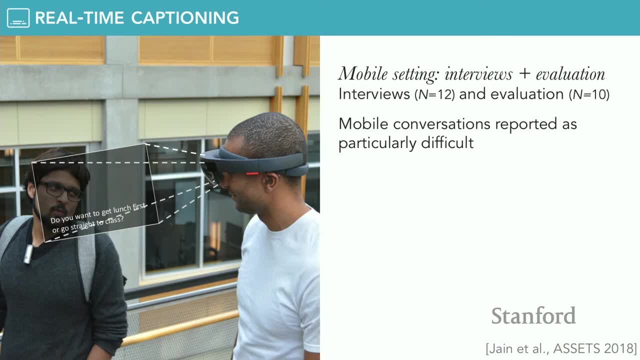 partner. that person might not stop talking until your visual attention can go back to them, whereas a deaf person might be more likely to do that. They're just used to doing that. So the head-managed display captions participants and I have a question and 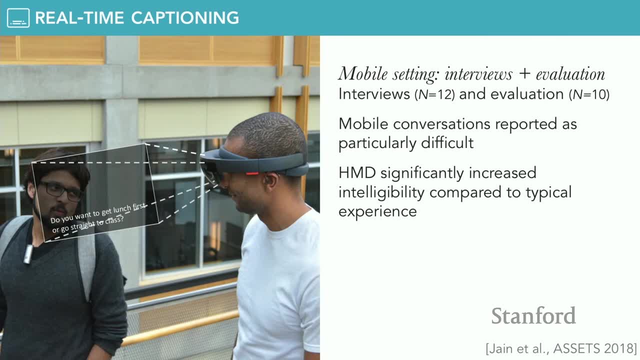 participants felt increased intelligibility compared to a typical mobile conversation experience And there are- sort of related to Michael's question earlier- many open design questions about how to present head-mounted display captions that were highlighted in the participant feedback, like how to minimize distractions. 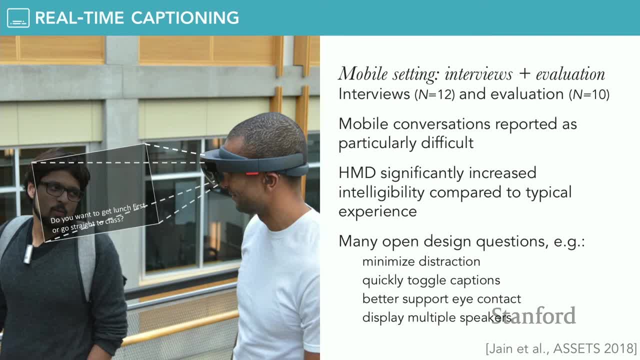 be able to quickly toggle captions on or off. They're distracting. if you're trying to think, for example, Better support eye contact, That HoloLens is a fairly dark screen, just as one example Displaying multiple speakers. So, anyway, many, many questions around real-time captions that I 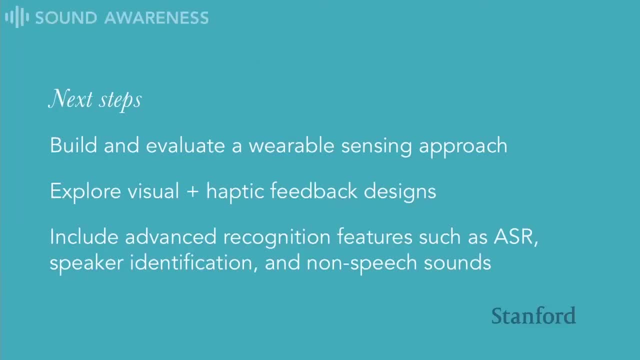 think are going to be interesting to explore. So, in terms of next steps, we are building and evaluating a wearable sensing approach and exploring visual and haptic feedback designs. We've focused so far on only visual, but there's a desire for haptic, for sure. 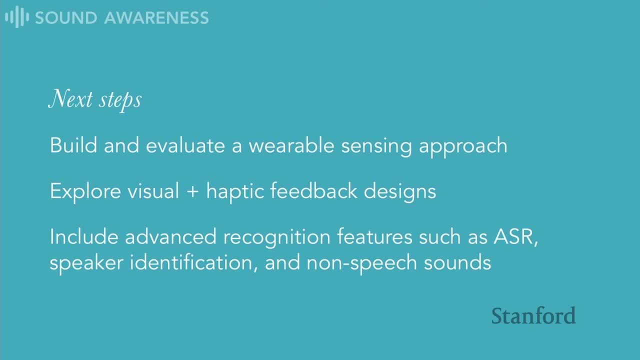 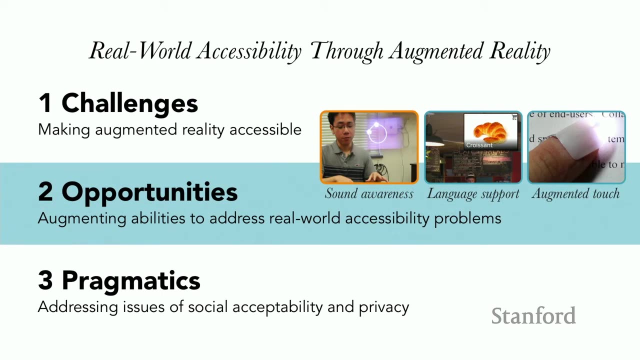 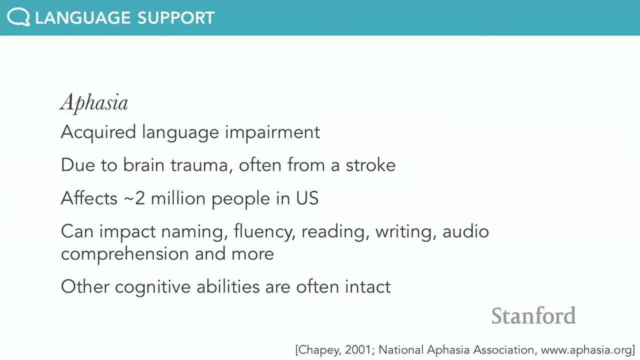 And then more advanced recognition features like ASR and speaker identification and so on. All right, So let's move on To a second project. This is on language support. So here we are working with people with aphasia, which is an acquired language impairment, most often due to a. 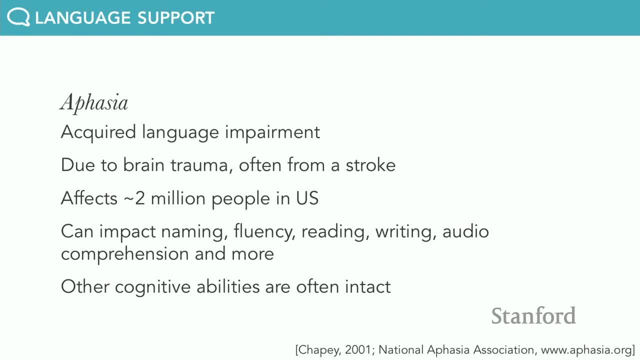 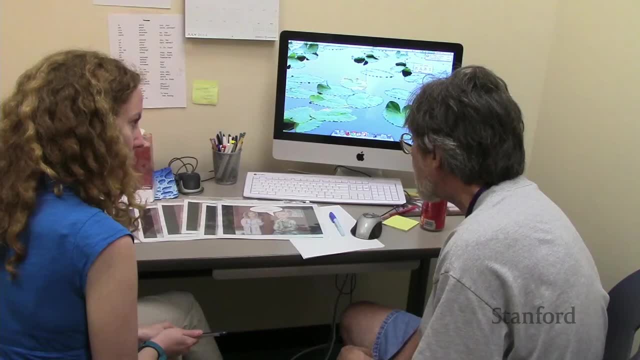 stroke and affects about 2 million people in the US. So let me play you a little clip here from a participant in our study who has intact audio comprehension so he can understand when the researcher- in this case Kirsten Williams, our lead student on this project- 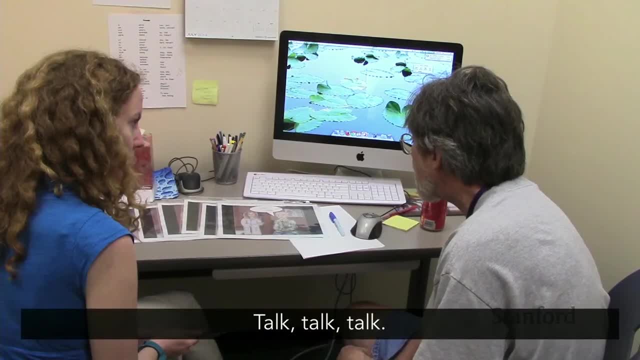 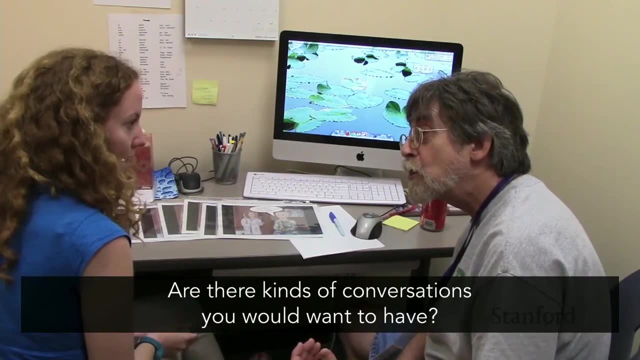 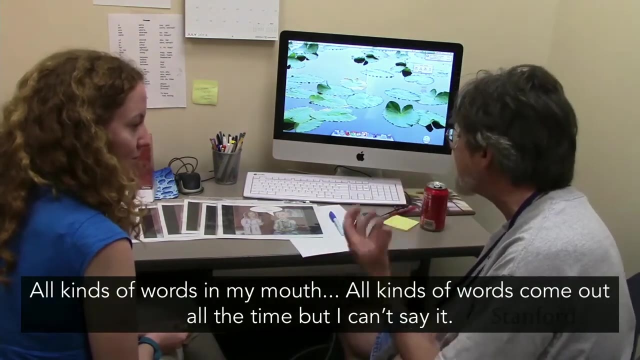 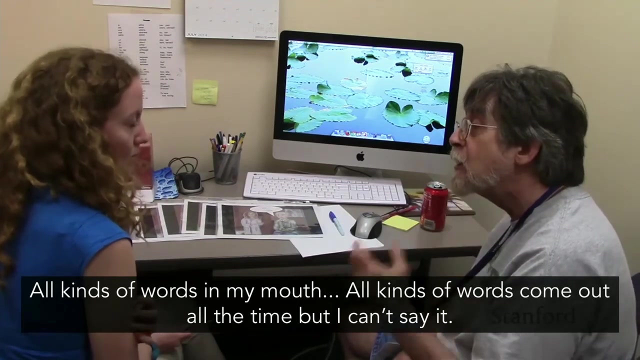 speaks to him, but he has trouble expressing himself. Talk, Talk, Talk. Are there kinds of conversations you'd want to have? Yeah, Like what? All kinds of words in my mouth. All kinds of words come out all the time, but I can't say it. 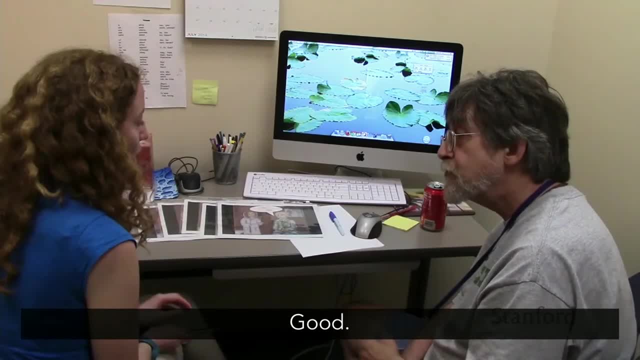 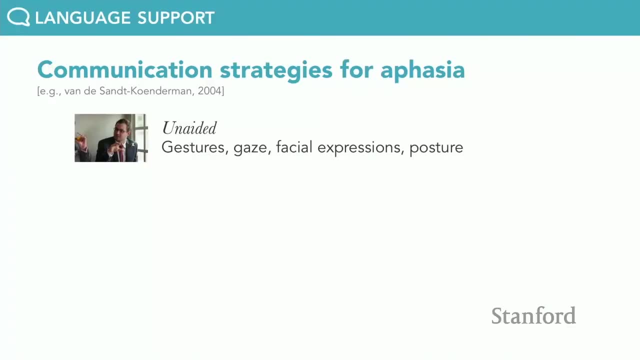 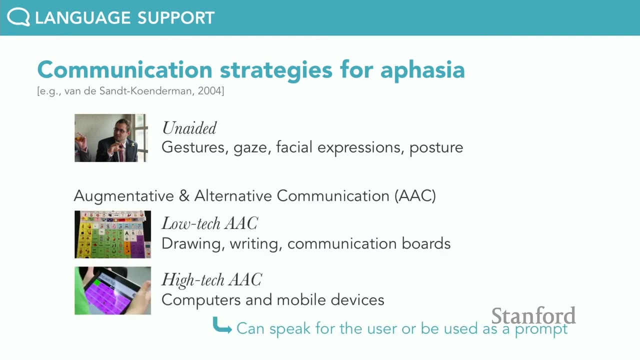 Good, So he had trouble saying the specific words he wanted to say, which is a problem that we're trying to address here. So communication strategies for aphasia range from unaided strategies like gestures and gaze, similar to what we were already talking about- paper-based strategies like drawing, writing or communication boards, and then high-tech strategies on computers and mobile devices. 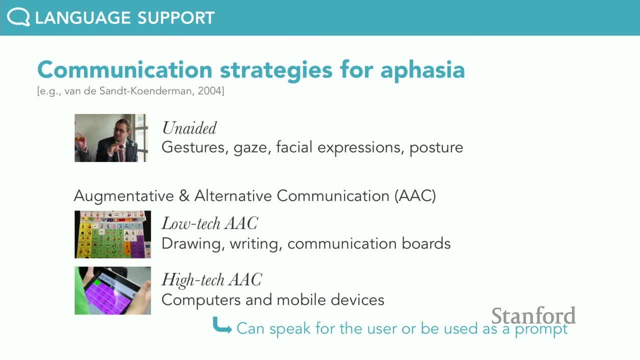 And the way these tend to work is that the user can look up a word and then either the device can speak for them using text-to-speech or they can say the word themselves, if it can prompt them to be able to do that. 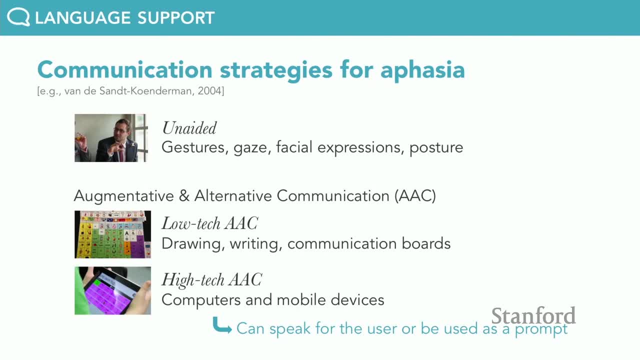 Yes, Just a detail on what they're dealing with. Is this a production issue? Like they can think the word or recognize it when they look at it, but they can't say it. It totally depends on the person. There are different kinds of aphasia and some people with aphasia can actually speak fairly fluently, but it doesn't necessarily make sense. 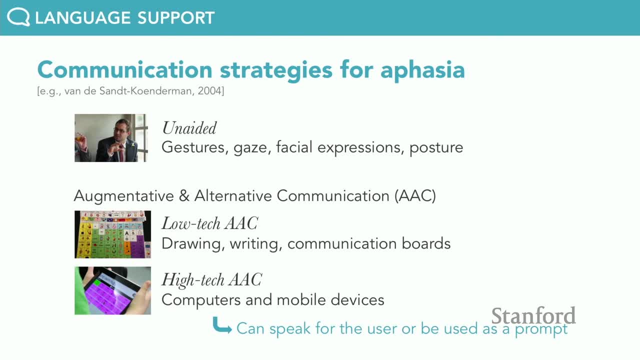 Other people speak more like the individual that you saw there, where they're having trouble coming up with the specific words, but the words that they're using are meaningful. But then, And also it can vary in terms of language modalities. So some people can read, some people can understand spoken language, et cetera, et cetera. 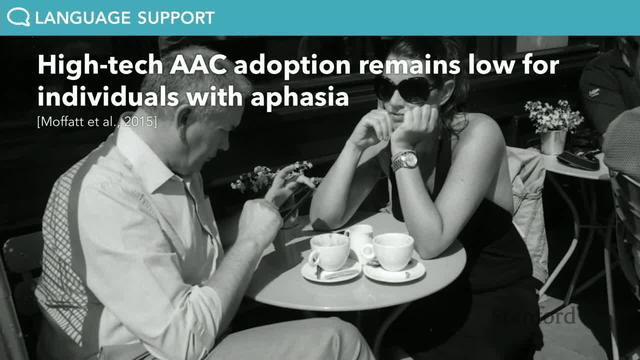 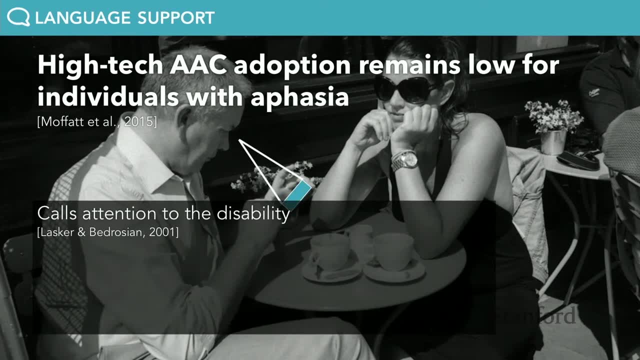 Highly varied. Okay, So high-tech adoption of AAC devices remains low for individuals with aphasia, because these call attention to the disability They tend to. They can replace rather than augment natural speech. So if their device is doing this text-to-speech output, then the user no longer has to speak for themselves. 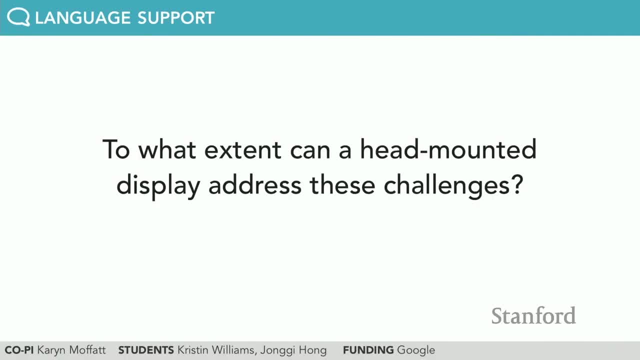 They can Divert gaze and impede use of visual cues. So we are exploring the extent to which a head-mounted display can address these challenges of attention replacing speech and diverting gaze. So here's a scenario we showed to participants in one of our studies. 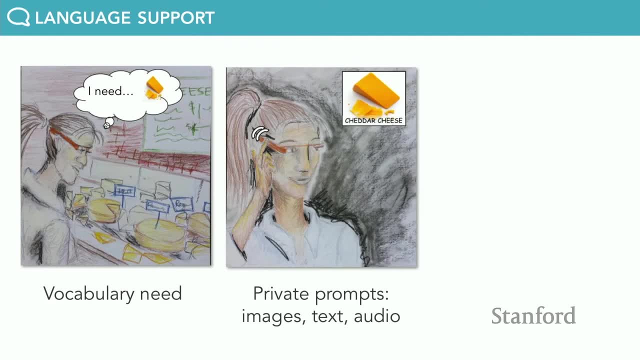 A woman's at the grocery store. She has a vocabulary need, but she's preloaded her grocery list onto this device so she can look up that word and get a private image, text and auditory prompt, any of which may spur her own ability to say the word, which she can then go do independently. 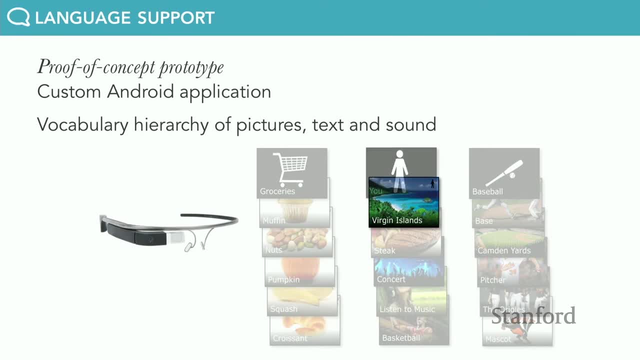 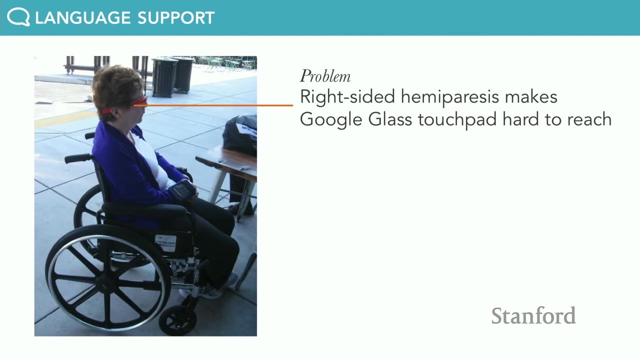 We built a proof-of-concept prototype on a head-mounted display and this again gives that picture, text and sound. prompt for a hierarchy of words. And because people with aphasia often have right-sided hemiparesis as a result of the stroke, this is weakness in the right side of their body. the touchpad on the side of Google Glass was hard to reach, so we used a wrist-worn touchpad here. 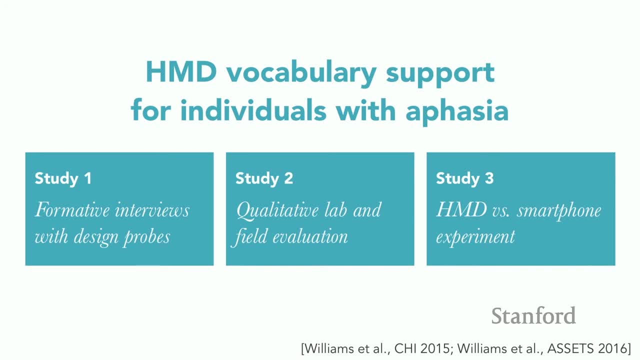 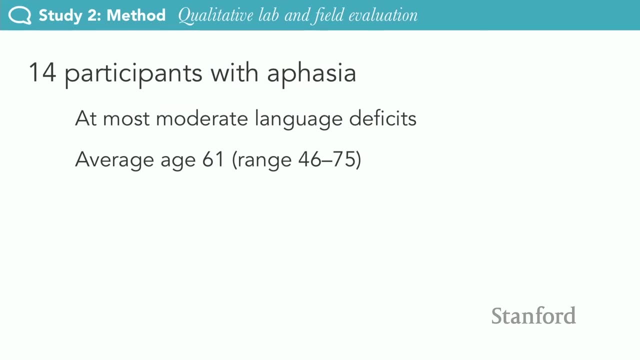 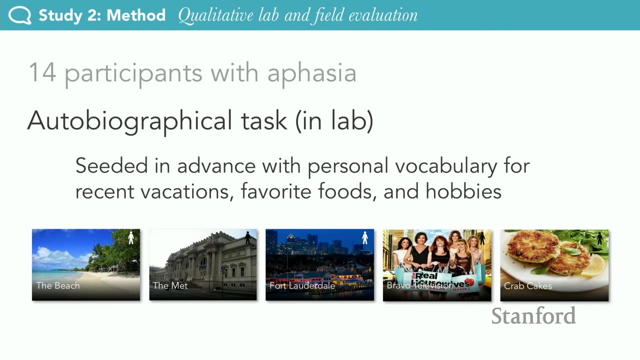 Now we've conducted a few studies. I'm going to tell you about the second one, a qualitative lab and field evaluation. Here we recruited 14 participants with aphasia and they completed a conversational task in the lab which was autobiographical, and we preceded the device with words related to their recent vacations, favorite foods and hobbies. 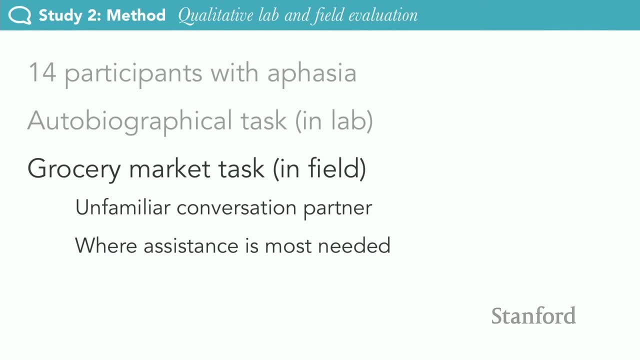 They then went out to the field and did a conversational task in the grocery market. So this is where, with an unfamiliar conversation partner, and is where help is most needed, Because at home, with a more intimate partner, you probably have communication strategies already built up. 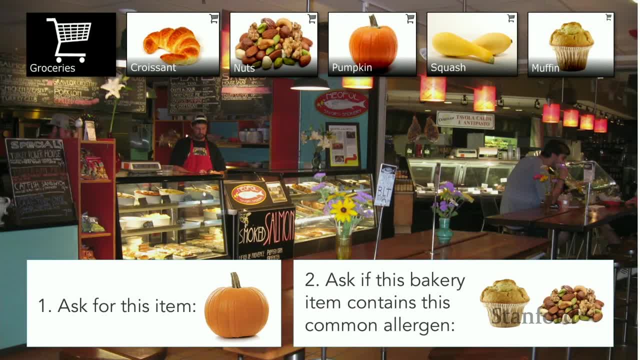 So here's our field site in Baltimore, and the task was to ask for this item- which of course we didn't say, but it was a pumpkin- and then to ask if this bakery item- a muffin- contains this common allergen nuts. 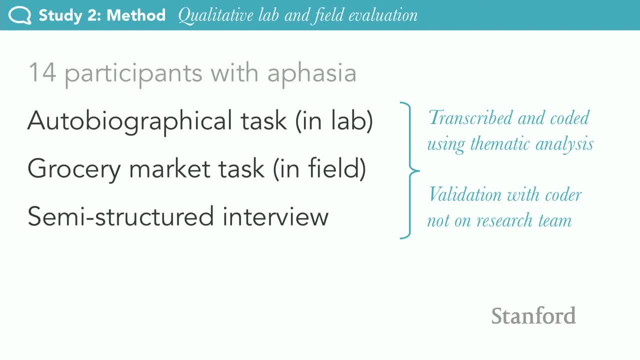 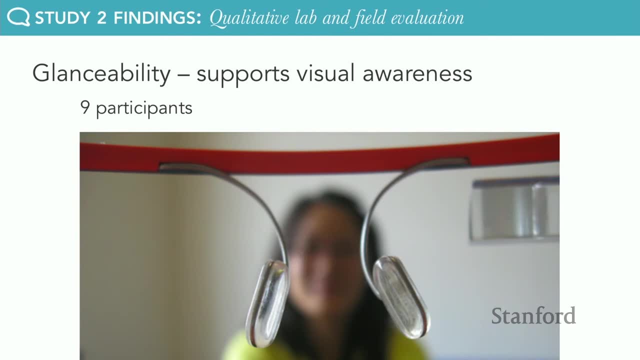 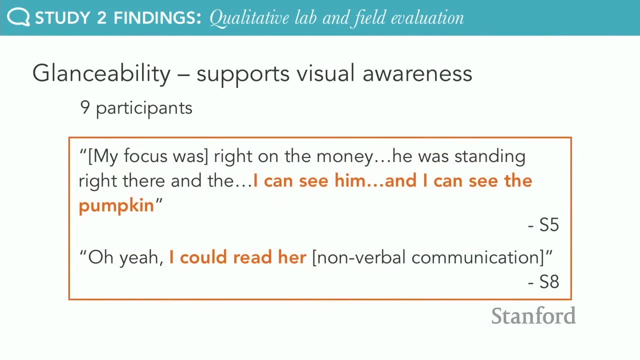 And then afterward we did a semi-structured interview. So for findings here, high-level theme was glanceability, So participants valued this support for visual awareness. For example, one person said my focus was right on the money. He, the clerk, was standing right there and I can see him and I can see the pumpkin. 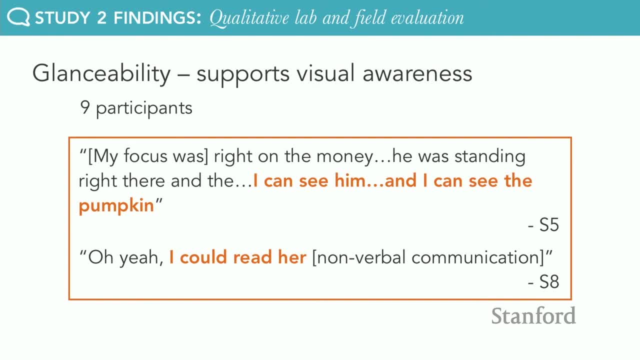 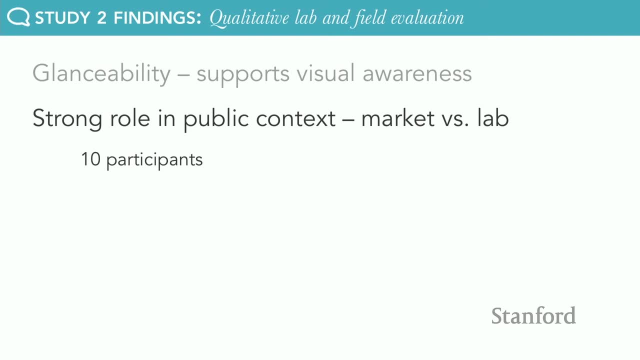 Another person said: oh yeah, I could read her nonverbal communication. A strong role was also seen for this kind of technology in a public context: that market versus lab setting. So, for example, busy place and friends or enemies meaning strangers. 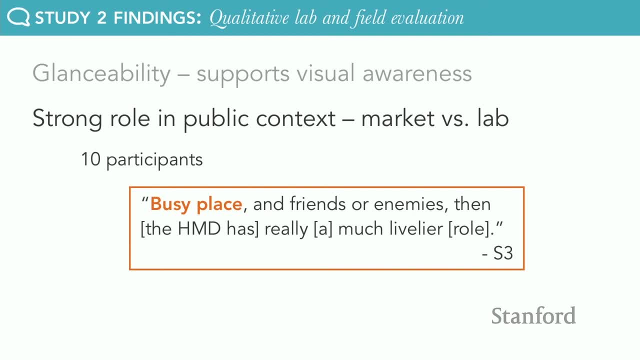 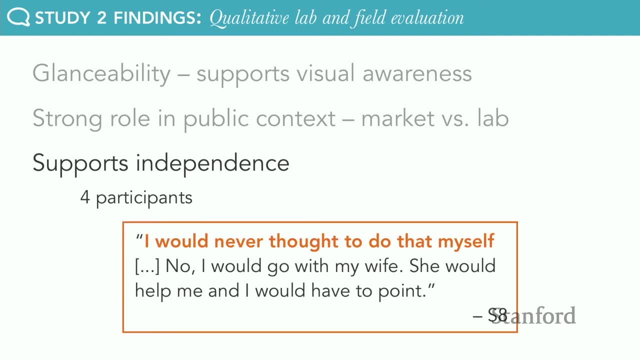 Then the head-mounted display really has a much livelier or stronger role. Some participants commented on feeling more independent while using the device, such as I would never have thought to do that myself. go to the market- No, I would go with my wife. 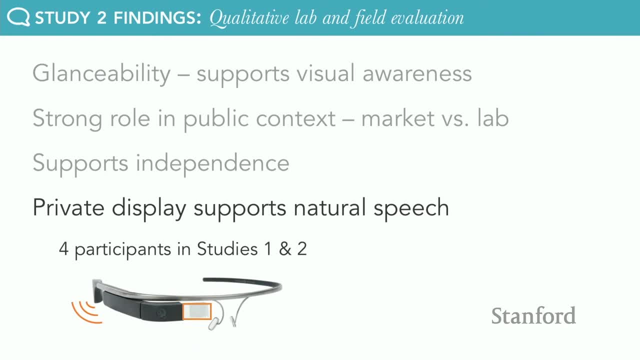 She would help me and I would have to point. And then, finally, some participants commented on valuing the private nature of that visual and auditory display that the head-mounted display provided. So, for example, I can't say it, but I know it. 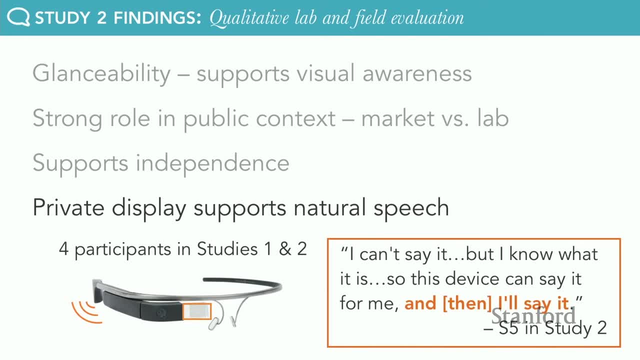 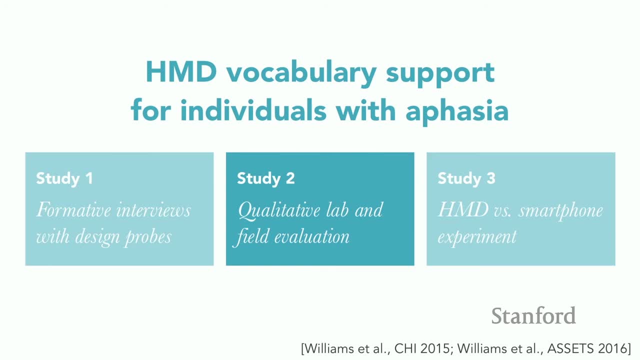 I know what it is, so this device can say it for me and then I'll say it. So that study provided some positive suggestion that this might be a useful approach to take, but it was qualitative and there was no comparison to a status quo. language support. 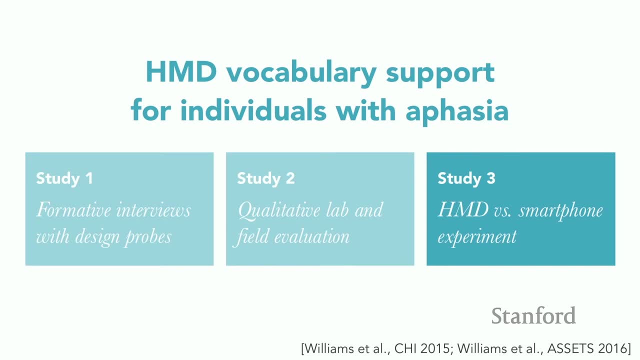 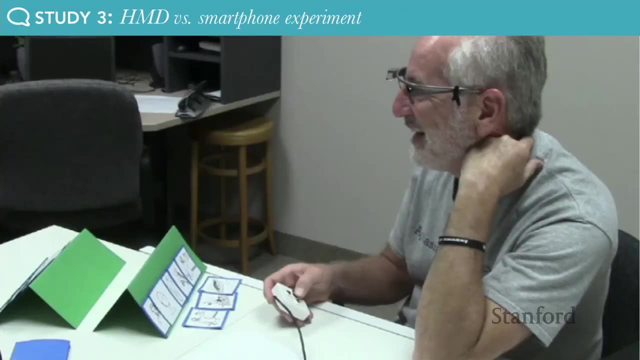 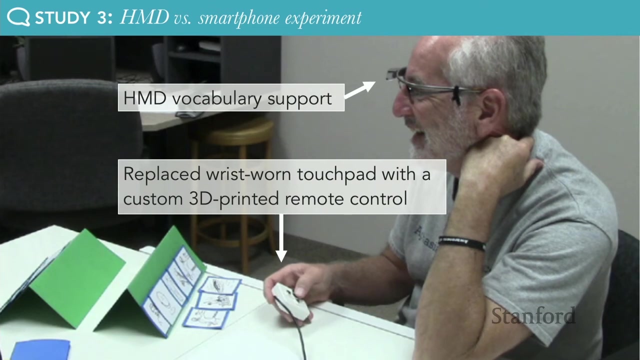 So in a follow-up controlled experiment, we showed the same vocabulary on a head-mounted display and a smartphone. So here is a participant Wearing the head-mounted display, and then we replaced that touchpad, that wrist-worn touchpad, with a 3D-printed remote control with tactile indicators, so you don't have to look at it. 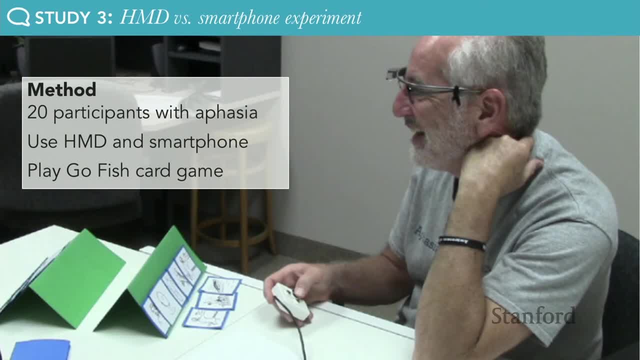 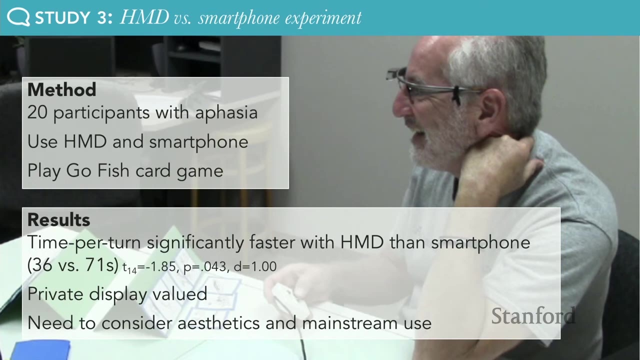 And then we had 20 participants use the head-mounted display and the smartphone and play a go-fish card game, which allowed for a constrained conversational task. Some highlights from the findings are that time per turn in the game was significantly shorter with the head-mounted display than the smartphone. 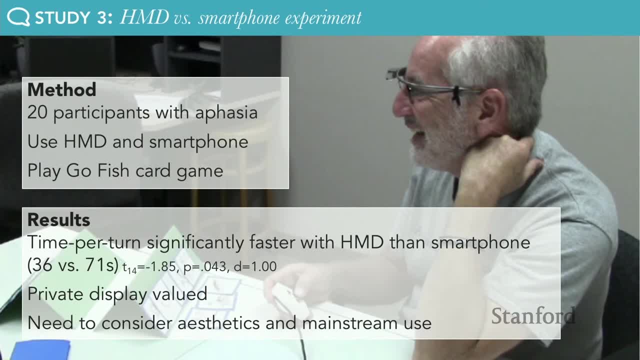 So more efficient game communication, And that the private nature of the display was valued, so similar to that theme from earlier. However, there was some comments about the aesthetics of the device and whether something like this would become used for mainstream use, or whether people would just be looking at them and thinking: what do you have that on your head for? 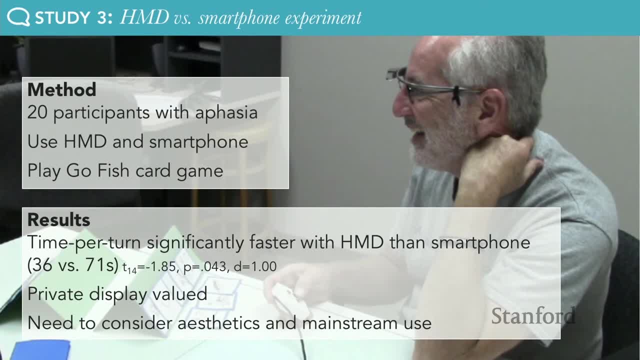 And this was probably around the time when Google Glass was starting. Well, Google Glass ultimately, As you all know, received a fairly negative response, but it was a fantastic technology for exploring some of these ideas, And so we presented it as sort of an early prototype of what this might look like. but this was anyway around that time too. 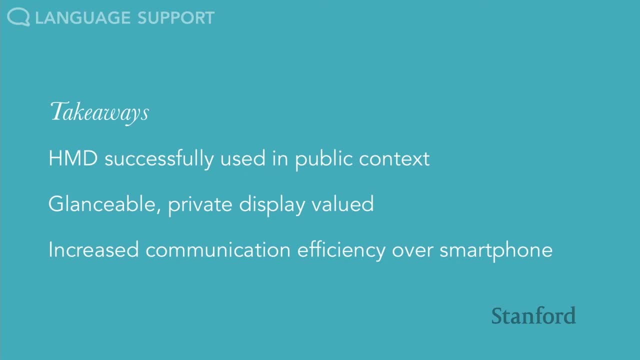 So, in terms of takeaways, the head-mounted display was used successfully in a public context. The private glanceable nature of the display was valued and in that controlled experiment we saw increased communication efficiency over the smartphone. So there are, However, 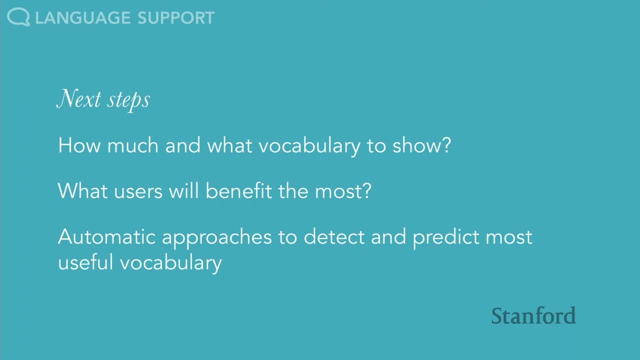 Many open questions here that I would love to work on- although I'm not currently doing it, so I also encourage you all to do it. So things like how much and what vocabulary to show what users will benefit the most, and we talked a little bit about some of the variability in users' language abilities. 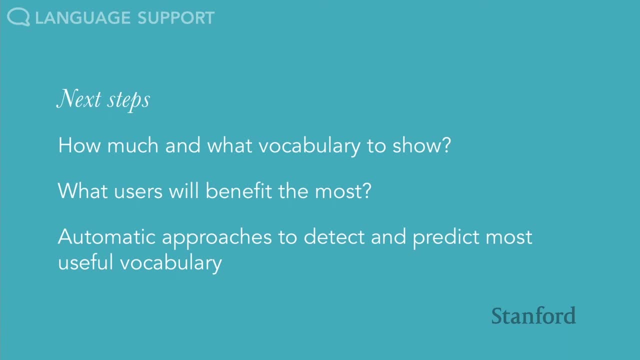 And then related to the first question, I think automatic approaches, context-sensitive approaches for detecting and predicting the most useful vocabulary, And this is going to be particularly useful for users, And this is particularly important with a head-mounted display, compared to, say, a tablet or a smartphone, where you might feel you know that you're going to be willing to navigate through all kinds of information in your AAC app. 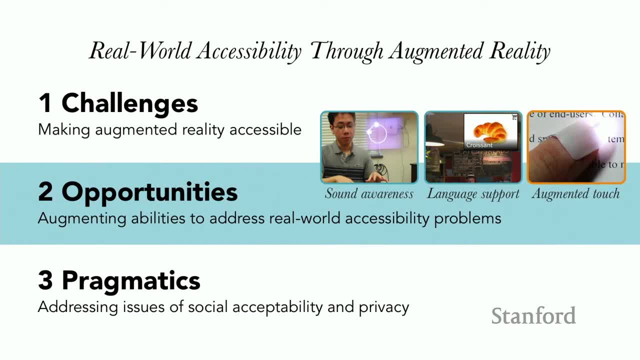 Now for this third project. I want to move on briefly, tell you, very briefly, tell you about this third project, which is different in that it doesn't use a head-mounted display. And here we're augmenting physical touch with computer vision. 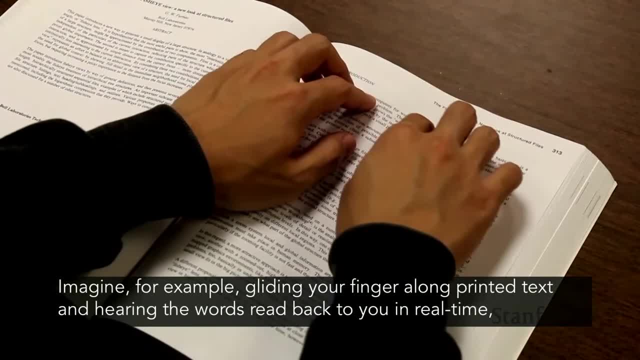 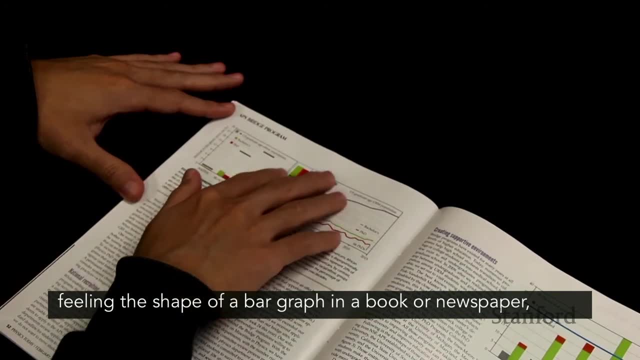 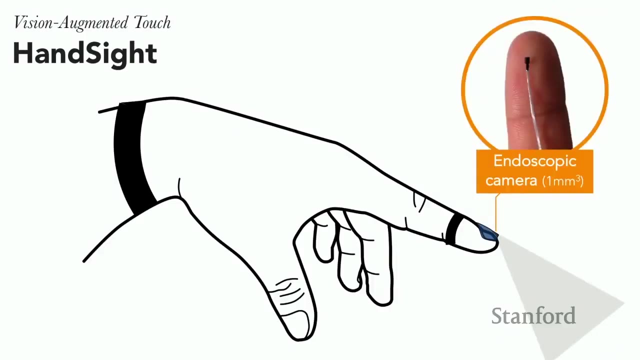 So imagine, gliding your finger along, You're looking at a printed text and hearing the words read out loud, or feeling the shape of a bar graph in a book, or touching a piece of clothing and hearing a description of that fabric. So here's an illustration of our approach. 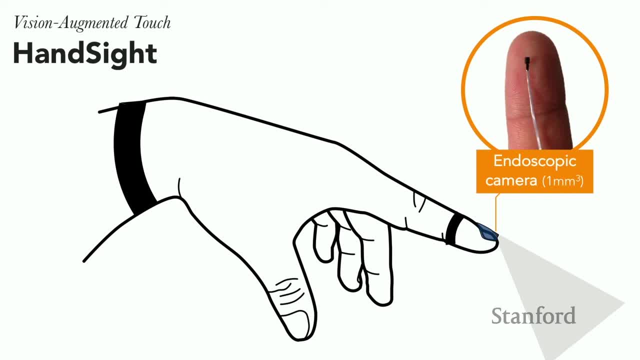 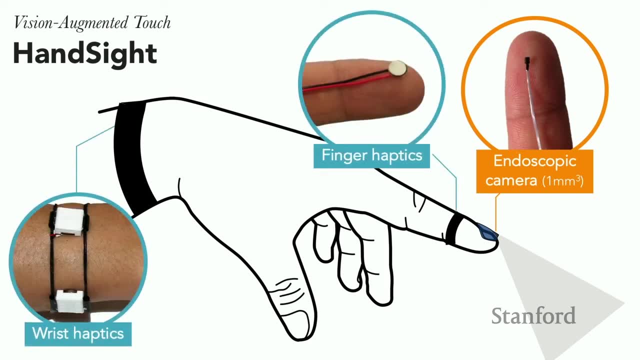 We used a tiny camera, originally designed for endoscopies. It's one millimeter in diameter, but if you add lights to it it is two millimeters in diameter, so huge. And then we add microhaptic actuators on the finger or the wrist. 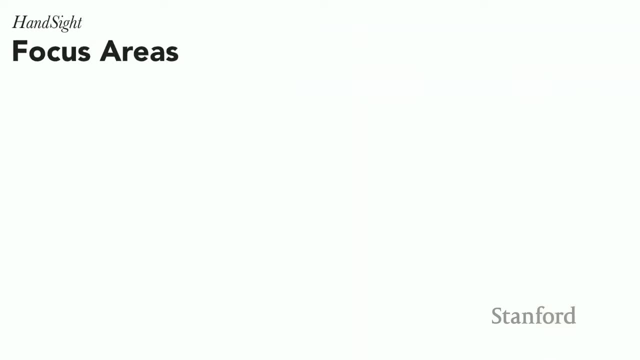 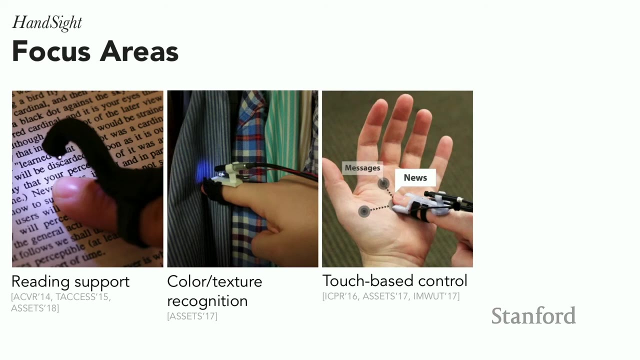 And our work here has been largely application-driven. so looking at instrumental activities of daily living like reading support, color and texture recognition. We've looked at touch-based control of mobile devices or mobile information, And then haptic and auditory feedback to guide the user's hand. for these other application areas, 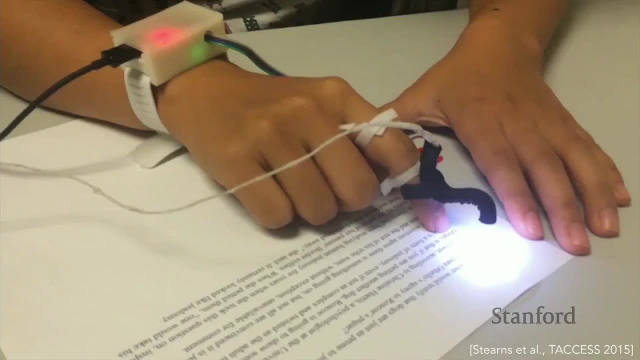 So let me show you two quick video clips. This first one is one of our early reading prototypes. This is for a blind user, Where you can read a printed text on a printed page and the system does OCR and reads the text aloud. 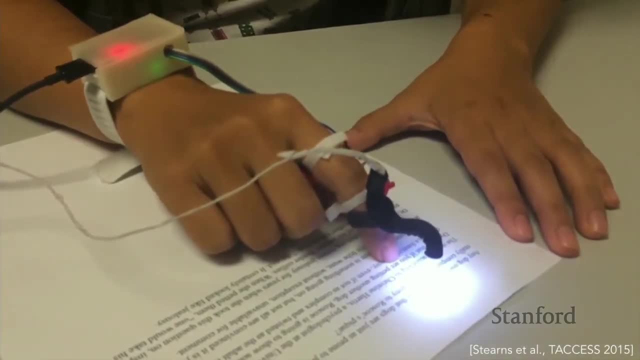 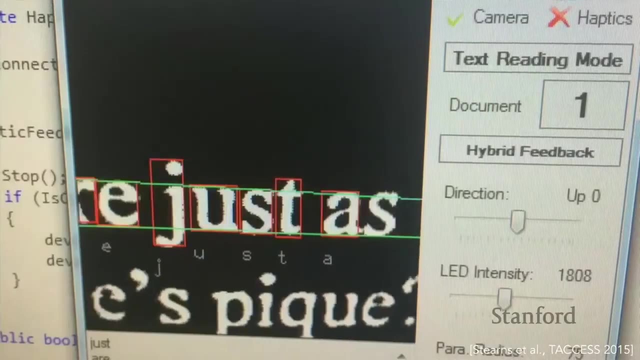 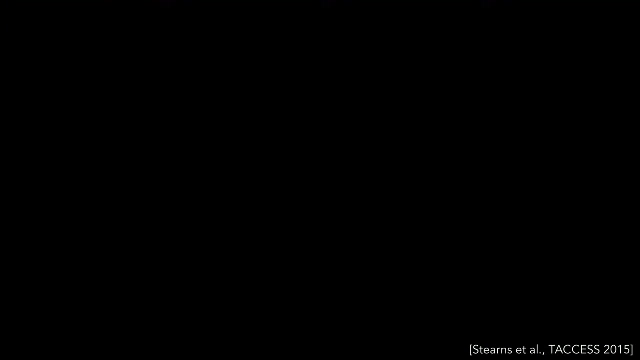 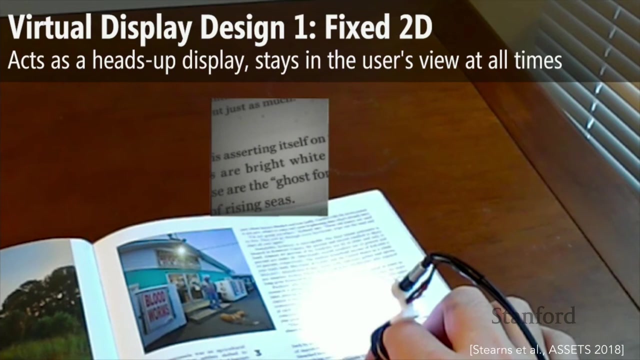 Any dog over the woods testified that dogs are just as prone to jealousy as humans. Okay, and then in this second example- this is more recent work, Actually, we just presented this. The lead student on this project just presented this last month at the ASSETS conference. 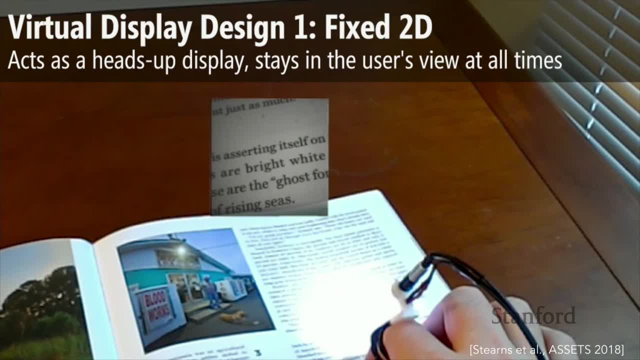 Here. this is for low-vision users, and we're taking the feed from the finger-mounted camera and we're magnifying it and doing some other manipulations on it. But, in particular, the study that we presented is exploring if you present this information on a HoloLens device. 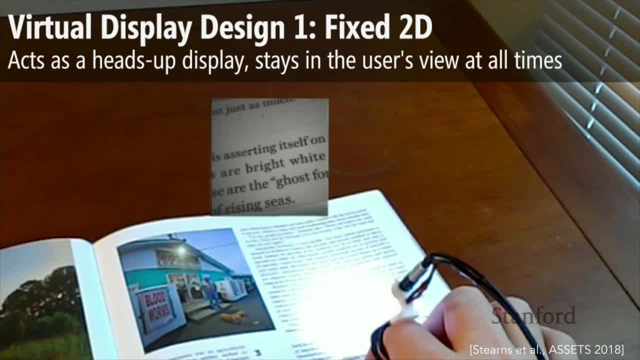 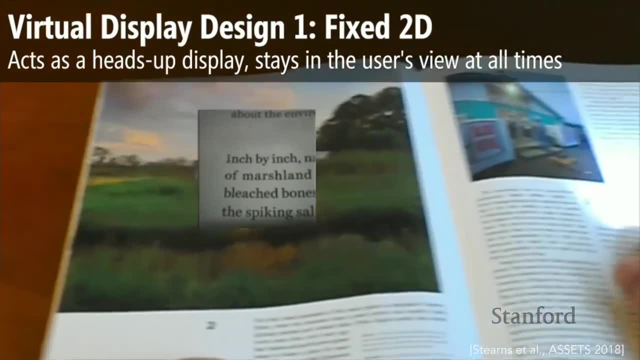 what does it mean to be able to attach that magnified view to real-world objects and so on? So one of our conditions had the view moving. It's moving within the user's field of view, like that, The magnified view as the user moves their head. 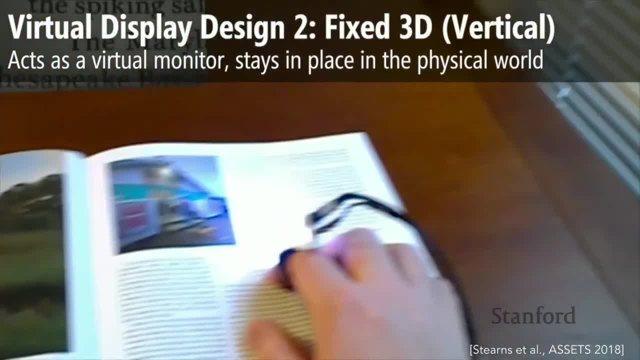 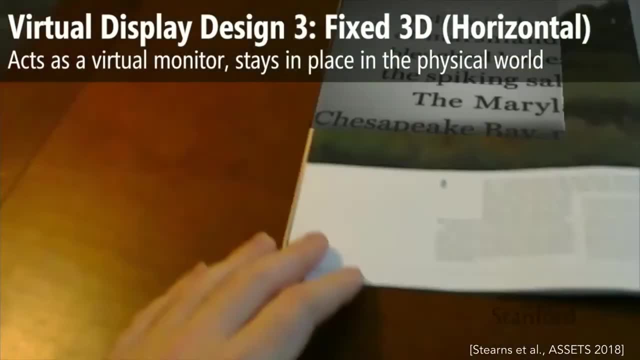 Here's another condition where the view is vertical. The magnified view is vertical and it's affixed to the top of the desk. And then here it's horizontal, affixed to the other page of the magazine that the person is reading. 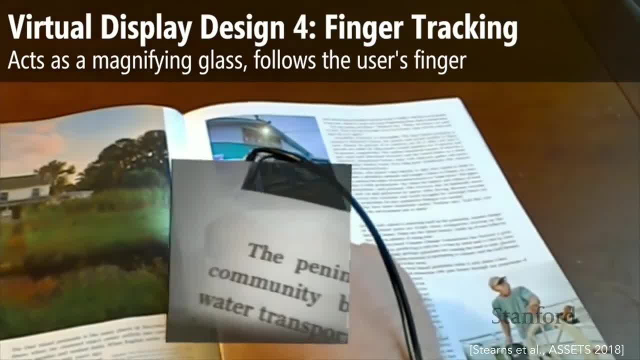 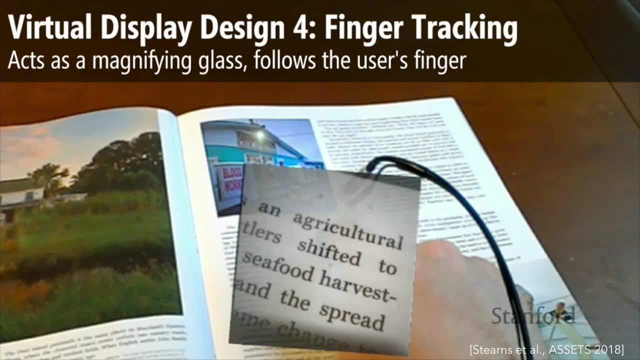 And then this one is where it's attached to the top of the finger. It's tracking the finger a little bit like a physical magnifier might work. So if you're interested in that, you can check out our ASSETS paper. Okay. 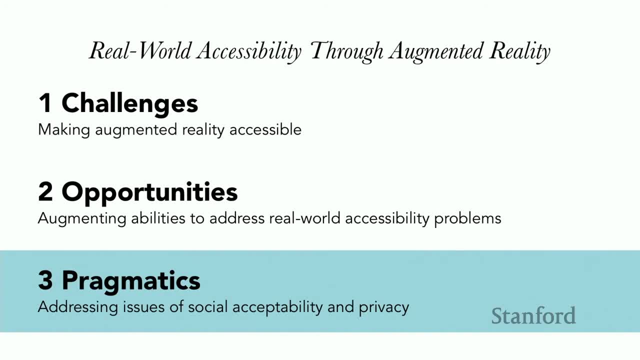 Now I want to turn to this last thread of work on practical issues and just talk about one study here briefly. So, like I said, if we want to have any of these technologies actually adopted and used in the real world, we need to think about issues like social acceptability and privacy. 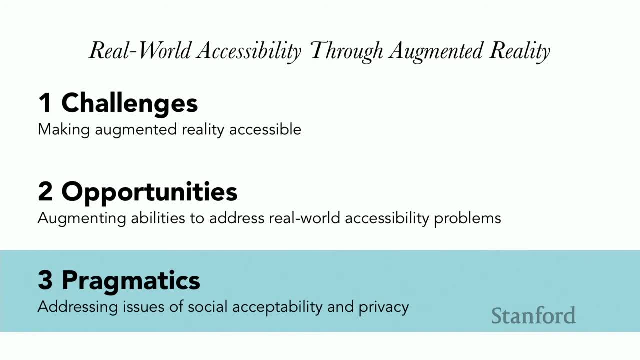 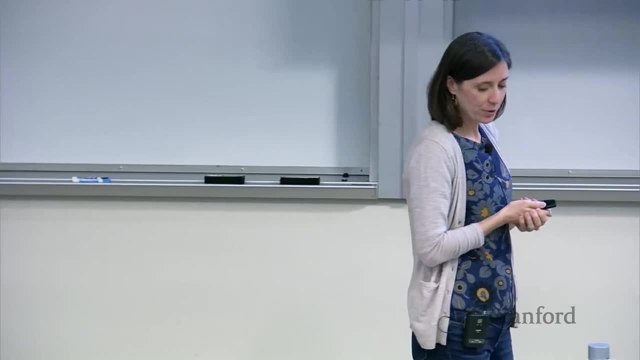 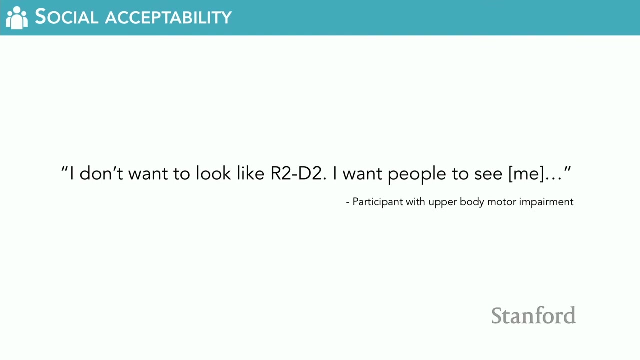 A lot of the technologies that might be particularly impactful for people with disabilities in terms of augmenting abilities might be sensing all kinds of information about other people in the environment, And so that can lead to questions about privacy and social acceptability. So, for example, here is a quote from one of our studies reflecting a sentiment that comes up from time to time. 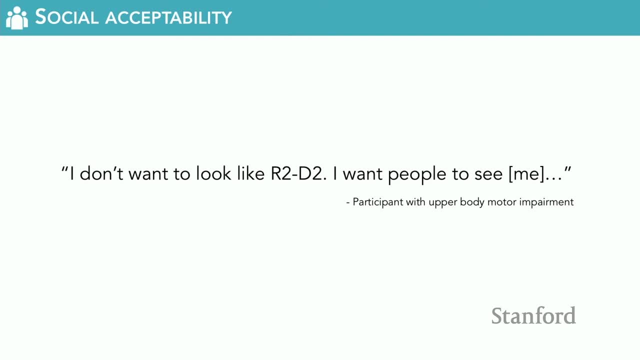 And this is from a participant with a motor impairment who actually liked the technology that he was trying out. He said: I don't want to look like R2-D2.. I want people to see me and not this wearable thing that you've created. 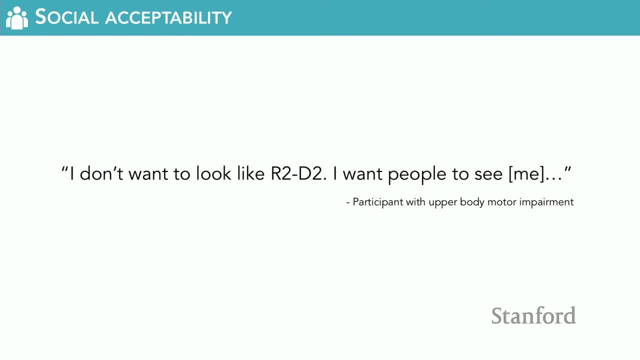 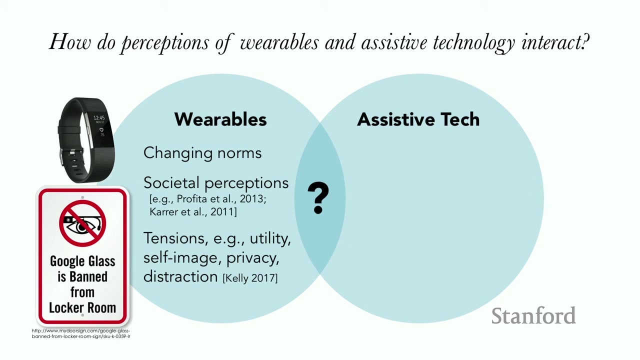 So we started to look at this question of perceptions of wearables and assistive technology along with Sean Kane and Holly Profita at the University of Colorado at the time. So perceptions, like for wearable devices, changing norms, changing societal norms around these devices. like probably, many of you in this room have Fitbits. 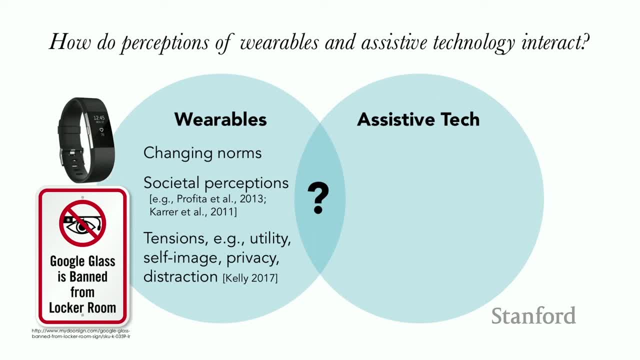 Lots of people have Fitbits But at the same time, in the end, Google Glass. people did not like that. It got banned from places. in fact, There are these tensions around the utility of the device. your self-image: What do other people think about you when you're wearing this thing? 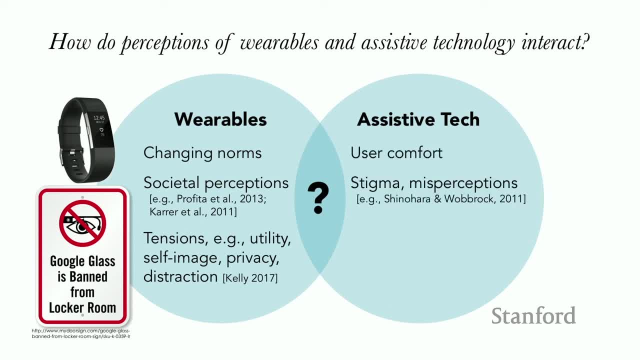 And then privacy and distraction is some examples. But then with assistive technologies we also have issues like the user's sense of comfort in using the device, stigma and misperceptions around it. What do you think about assistive devices? Here's a quote from Shinohara and Wolbrook that I quite like that kind of gets at all of this space. 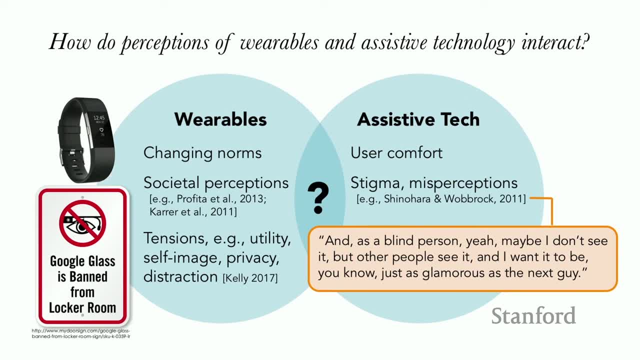 which is a blind person talking about their mobile device. And as a blind person, yeah, maybe I don't want, maybe I don't see it, the device, but other people see it and I want it to be. I want to be, you know, just as glamorous as the next guy. 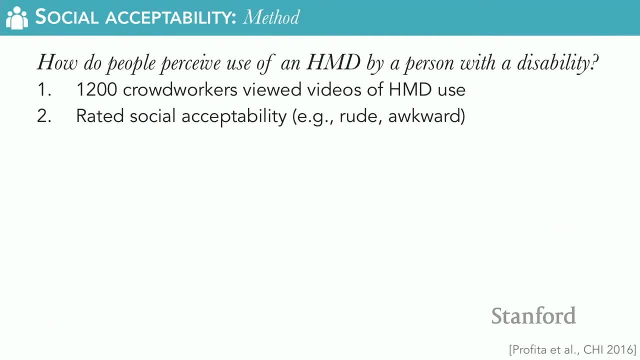 So we conducted a study with about 1,200 crowd workers To look at this question of how people perceive use of a head-mounted display by a person with a disability, And so the crowd workers viewed videos of head-mounted display use, and then they rated those videos on several dimensions. 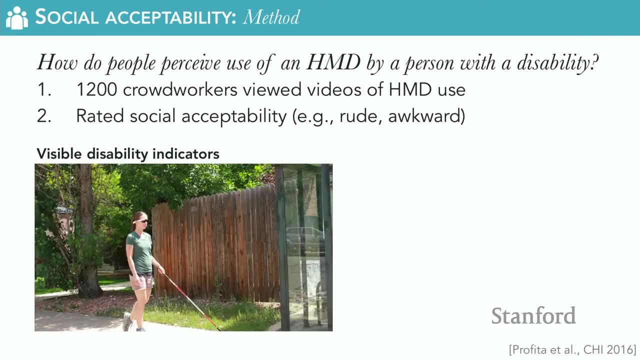 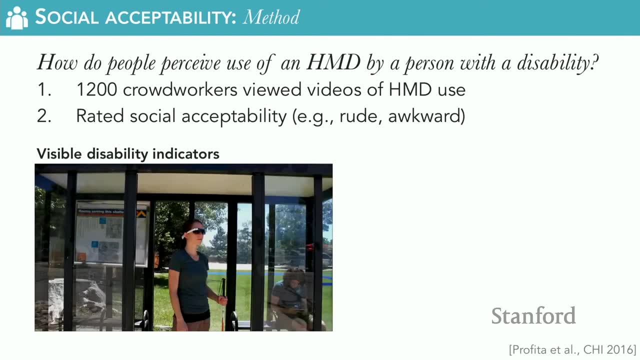 like whether it looked rude or awkward to use the head-mounted display. So here we had two videos. The first one included a visible disability indicator, So the actor wore the head-mounted display along with dark glasses and held a white cane. She's standing at a bus stop. 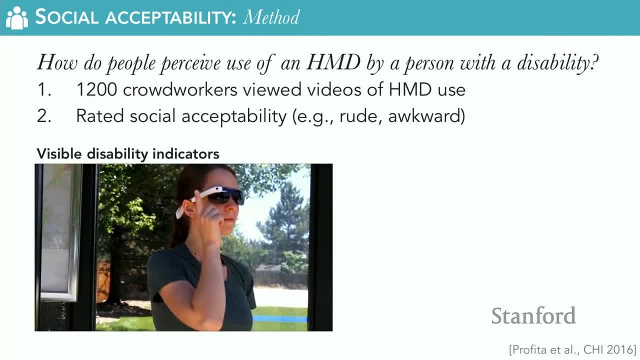 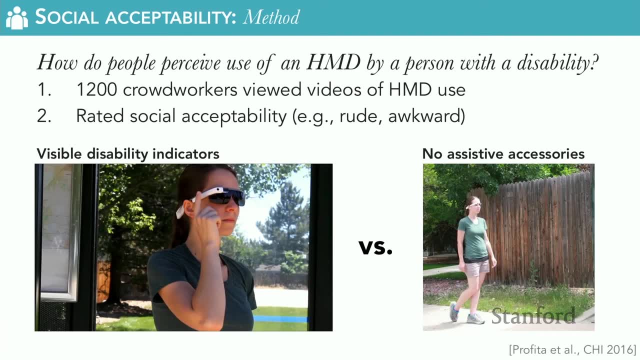 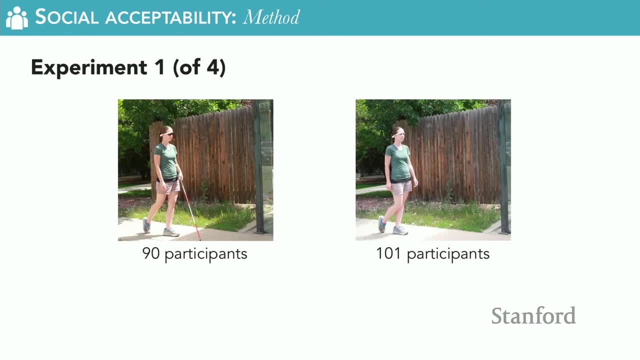 And she's going to do some taps and swipes on that head-mounted display. Okay, So that's what the one video was like, And the other one was exactly the same, except that it didn't include those visible disability indicators. So in the first of four experiments, which is the only one that I'm going to talk about for sake of time, 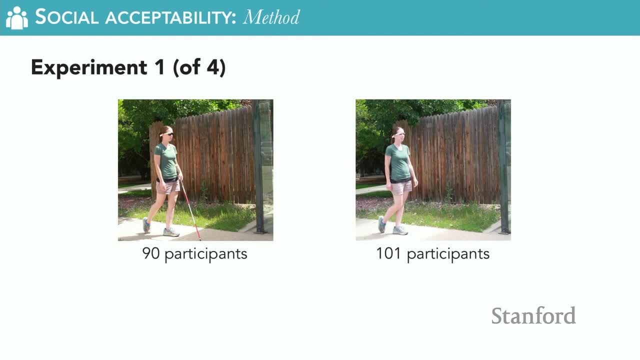 we had a number of participants view one or the other of those videos, but we gave the same video description for both groups. The following video shows a person at a bus stop using a wearable computing device. So here are some results from this experiment. 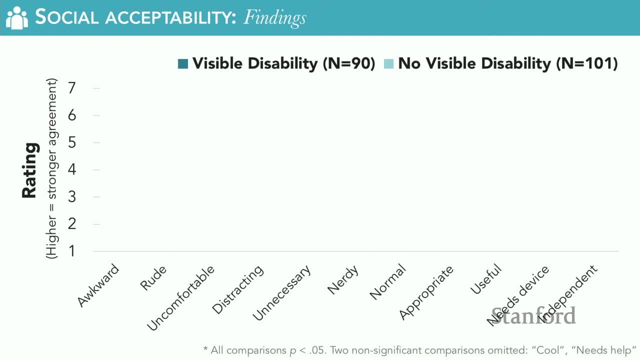 On the y-axis we have our different social acceptability dimensions And on the y-axis are the ratings. so higher numbers indicate stronger agreement. So overall the negative perceptions of the head-mounted display use were significantly lower with the visible disability indicators than without. 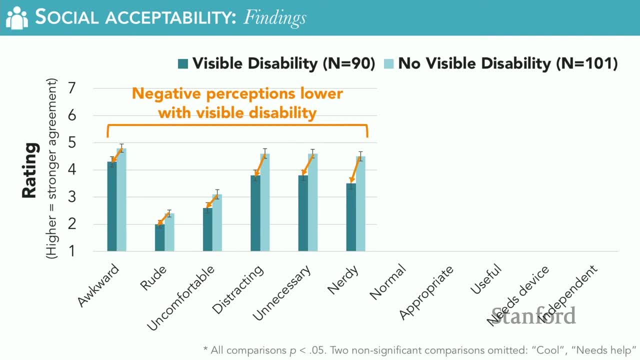 So, for example, the video with the person holding the white cane was seen as significantly less awkward Or rude. Yes, What's the baseline number here? Like what would it be if they weren't wearing anything? We did not have that. 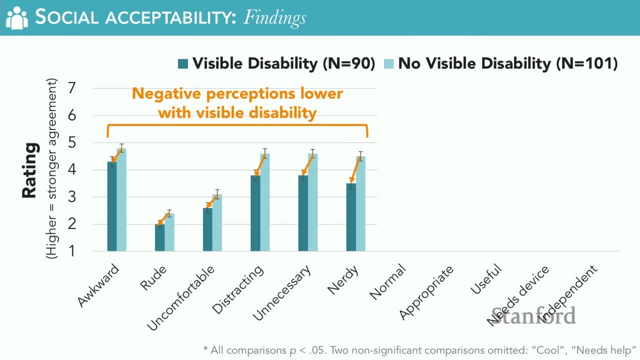 So that's a good quote. If they weren't wearing anything like, just how awkward or rude is it to be standing at the bus stop? Yeah, I guess my reaction is this seems like a really small change in effect size, but maybe it's just that you know the baseline numbers wouldn't be that much lower anyway. 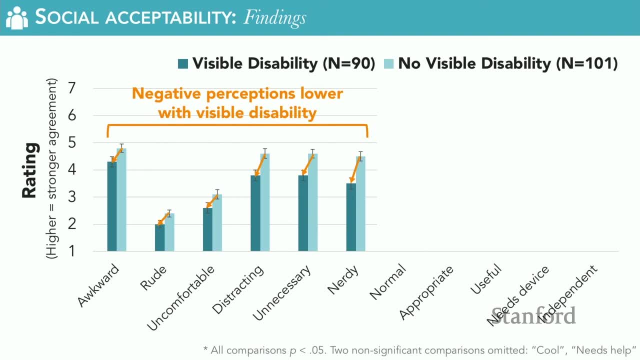 Right, Like I'm wondering if maybe it's just that there's not much for them to control. They can't go down much. I'm just surprised that, like it's only slightly less awkward- I mean significantly less, but slightly. 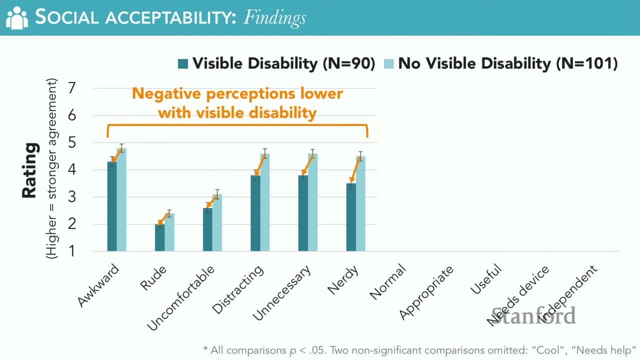 Yeah, You know. one thing that I actually don't remember is if this is neutral in the middle, Oh, Stronger. So I'm providing you with a relative result here. Yeah, So it might be interpreted as a two means very –. 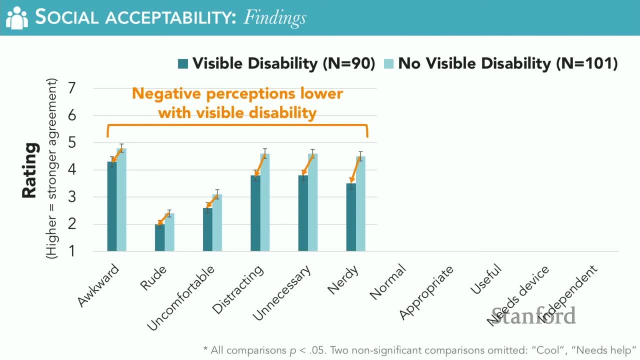 I disagree that this is rude. I will have to look that up, Although actually I warned the students I might do this. Did anyone? –? some students read this paper recently, Do you remember? Okay, Fair enough, Fair enough, Okay. 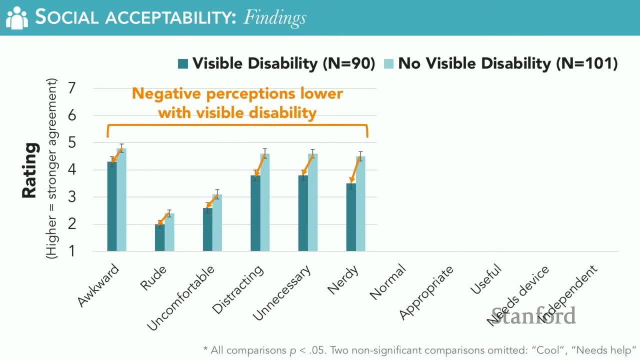 I can tell you later, Because then it gets more rude if it's – that's weird, Right? Yeah, So the overall trends here are that negative perceptions are significantly lower, and this is relative. It would be interesting to know. It would be interesting to know what the baseline is too. 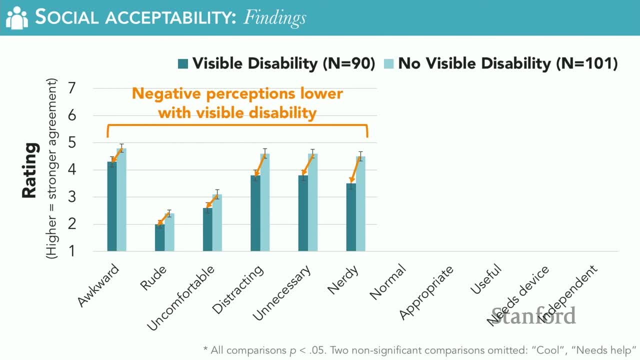 But this relative experience distinction still exists, regardless of what the baseline is. And then positive perceptions were significantly higher, So it seemed to be more appropriate or useful. And then there were some mixed results around whether the person looked like they were needing – dependent on the device, whether they needed the device. 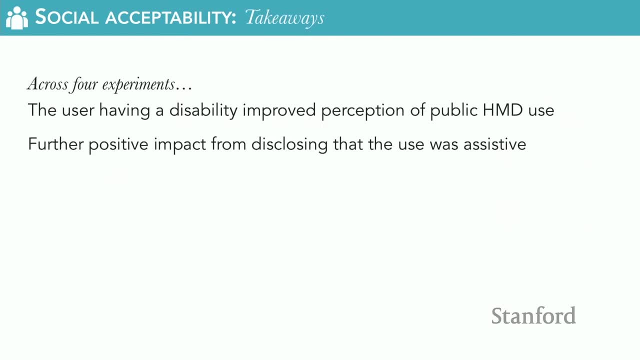 Okay, So across the four experiments – and now we'll have five After this, I'll go start that up: The user having a disability improved perception of head-mounted display use and that there was a further positive impact from disclosing that the use was assistive. 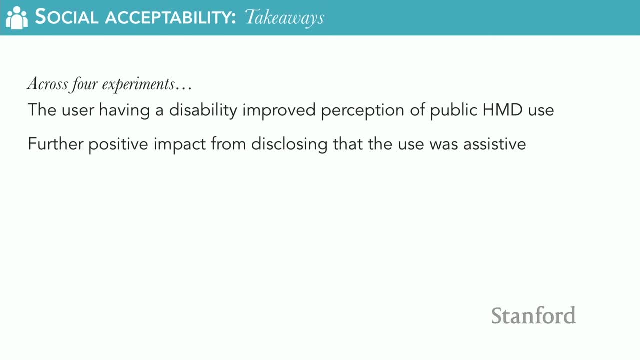 So, for example, saying that the device was being used to read street signs, versus the person was checking their Facebook feed. Now, there is an important tension here in that many people – yes, Question. I'm wondering if it has something to do with the trustworthiness of the device. 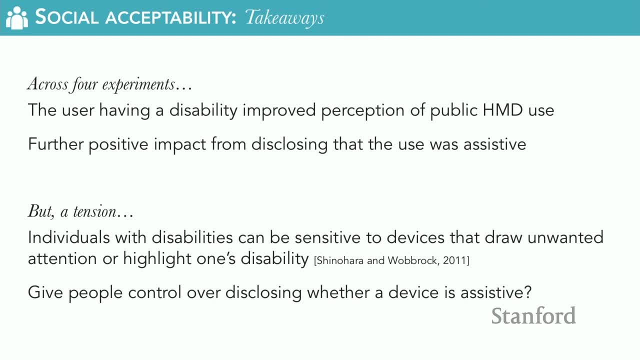 Because, regardless of who is using it, I would rather be – I mean, I would know that the device is recording me And the data might be shared with companies or somebody else. Yeah, Apart from helping the user, So does that also like influence my decision to say okay, that's rude. 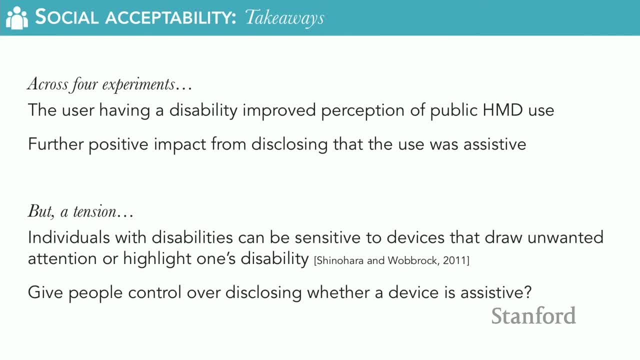 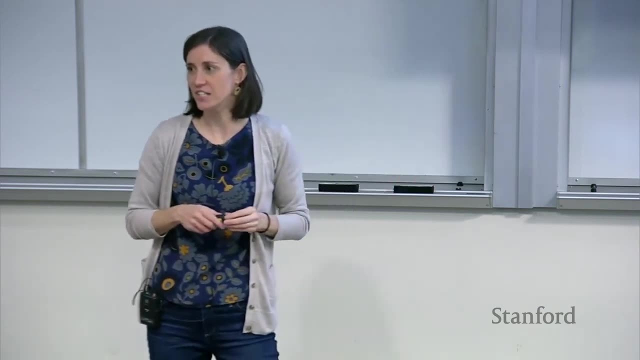 I don't want to be recorded, right. Right, I'm sure it does, Yeah, So the characteristics of the device and whether the person thinks that it might be useful, Whether the person thinks that it might be recording them, will probably impact how people are reacting to this question. 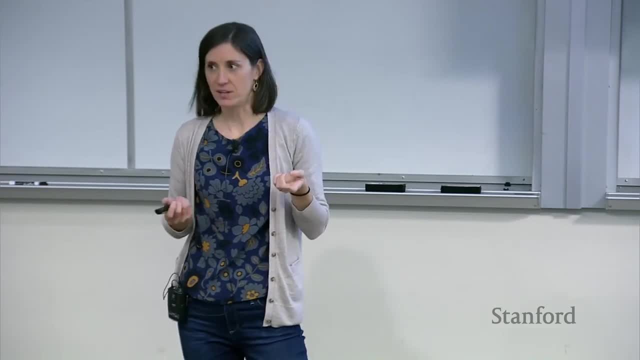 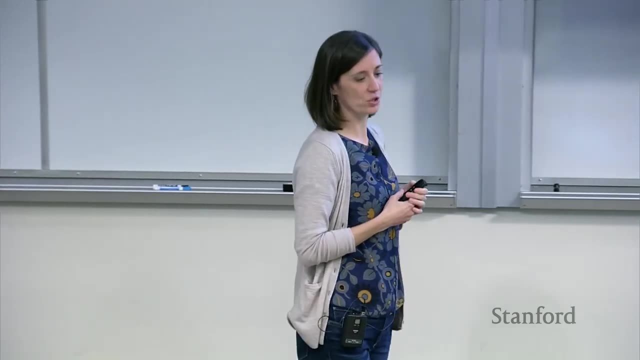 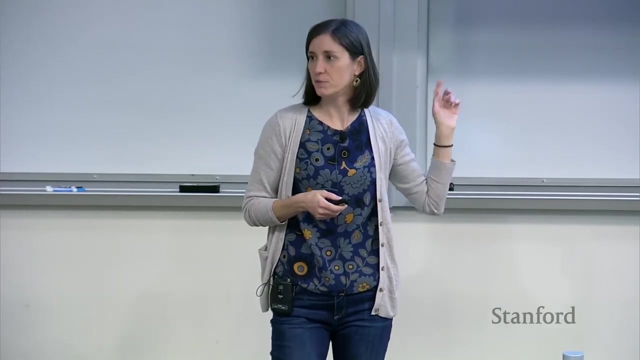 Yeah So, you know the fact that the head-mounted display in this case has a camera, which we mentioned? Yeah So, but you know if you have a – so these findings are specific to this kind of device, Although my guess is that, if we replicated these experiments with different devices, 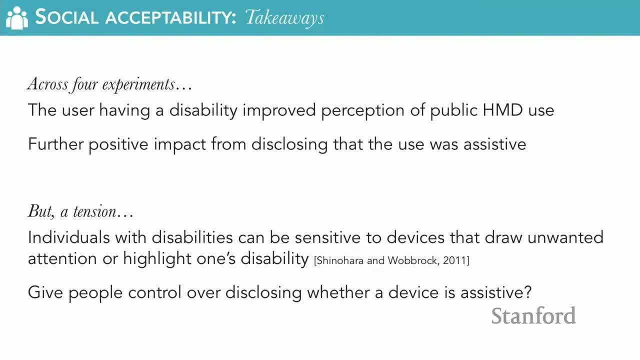 you'd still find similar trends. You know, maybe the bars would be overall higher or lower, you know as a baseline, But you'd still find similar trends. So yeah, It's a good question, Interesting to think about. So individuals with disabilities can be sensitive to devices that draw unwanted attention, which I've already mentioned. 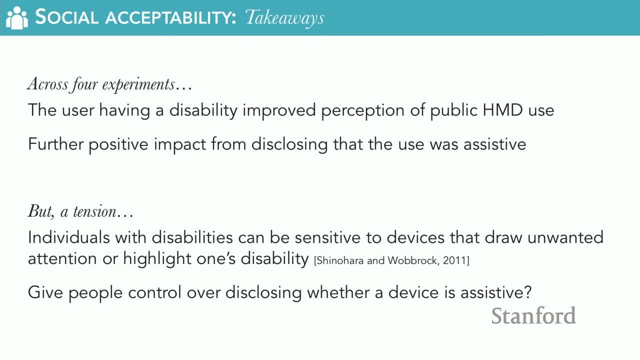 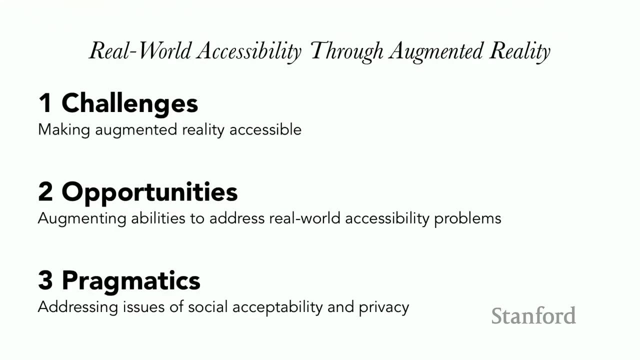 And so I think there's an interesting design challenge here to think about. How can you maybe give someone a chance, How can you maybe give someone control over disclosing whether a device is assistive or not, so that, if they want to, they can do that and possibly tap into this positive outcome, you know, if the tradeoffs are there for them? 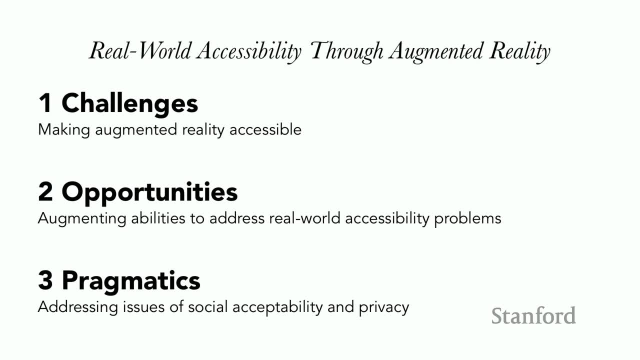 Okay, So that study is just a first step in starting to explore these issues of social acceptability and privacy, And I think there are huge ones, And some of the student conversations that I had this morning I had some nice discussion around some of those issues. 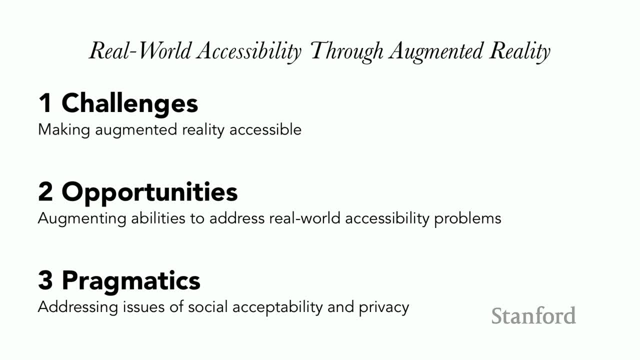 So it's good to see that a lot of people are thinking about them. So toward I think that overall augmented reality holds tremendous potential for improving real-world accessibility for people with disabilities And, to get there, that we need to think about all three of these threads of work.